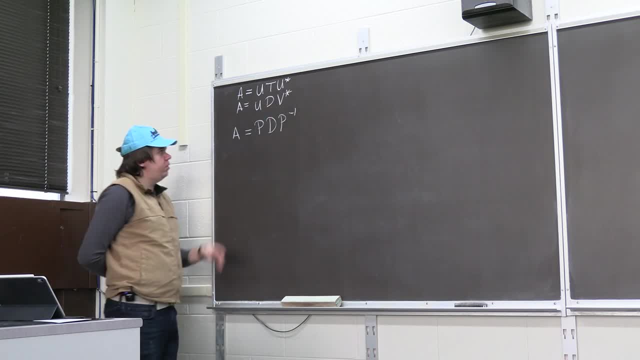 So that's when we write it of this form. But now U and V are not necessarily the same matrix, Right? They're not necessarily the same basis. U is some unitary matrix, V is the Inverse or the conjugate transpose or some other unitary matrix. 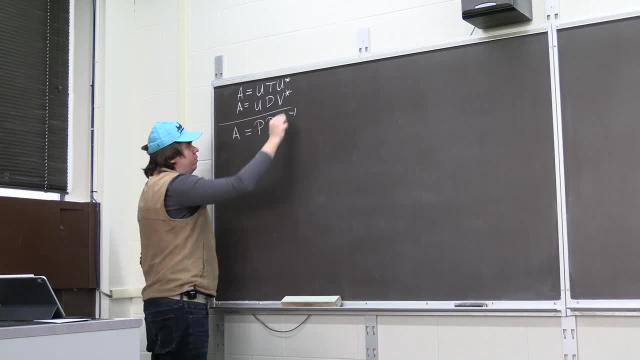 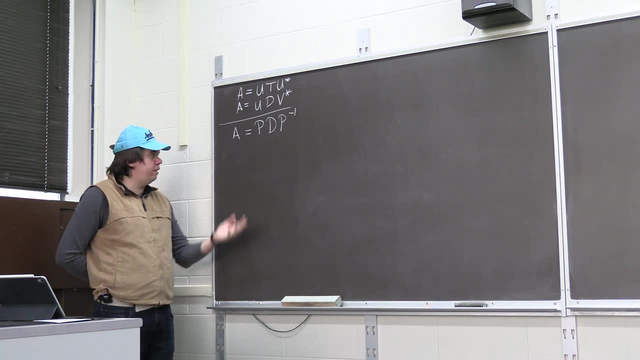 So it's like those kind of have this vibe But neither one really gives you in general a diagonal matrix And that's because in general you can't Right, If you're given some arbitrary matrix A, you're not always able to diagonalize A. 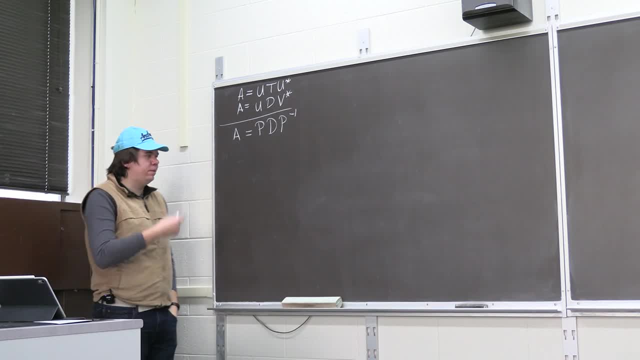 So maybe if you think back to your first course in linear algebra, you're given some conditions about. you know a matrix is diagonalizable if and only if, And you have these kinds of conditions. I want to remind you of that with an example. 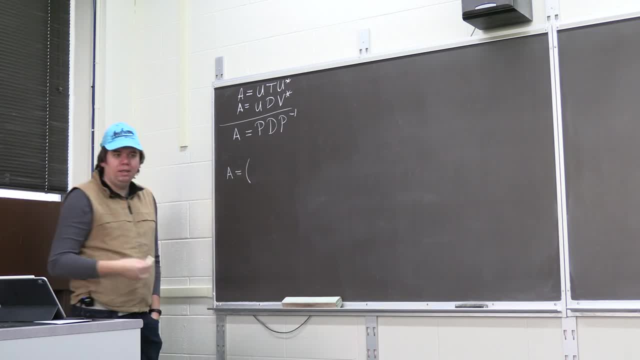 So I want to show you an example of where diagonalization might fail and try and help you remember what's all going on there and why it fails. And then we're going to say, well, is there some way to patch this up, to do our best to diagonalize a matrix? 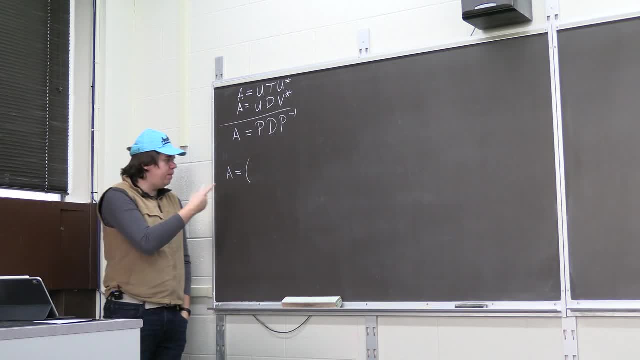 Maybe it won't be exactly diagonal, but maybe we can get pretty close. So the matrix A I want you to think about is this guy. So I want to open with a really concrete example. I did this out last time, So I want to open with a really concrete example. 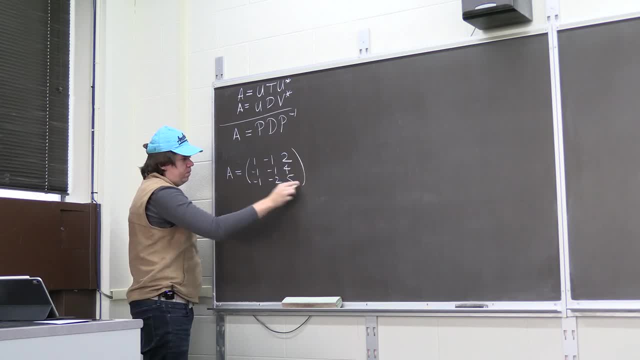 I did this out last time, So I want to open with a really concrete example. I did this out last time, So I want to open with a really concrete example. So I want to open with a really concrete example. So here's the matrix. 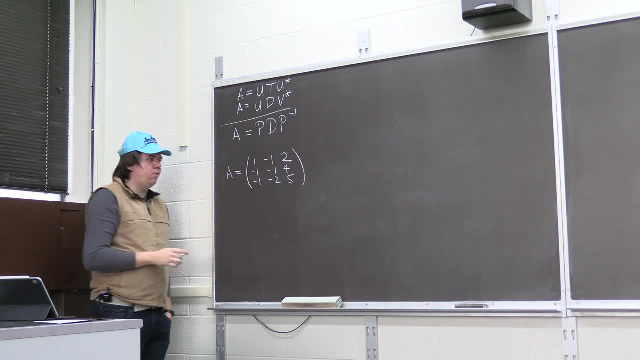 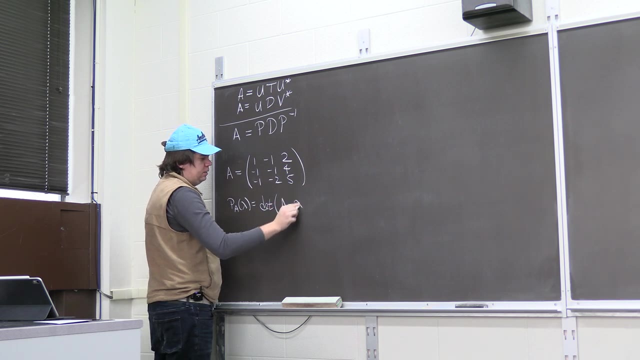 OK. So we want to know if this is diagonalizable, And so one first thing we can do is calculate the eigenvalues of this matrix. And so we find the eigenvalues by looking at the characteristic polynomial, which is defined to be just the determinant of A minus lambda times the density. 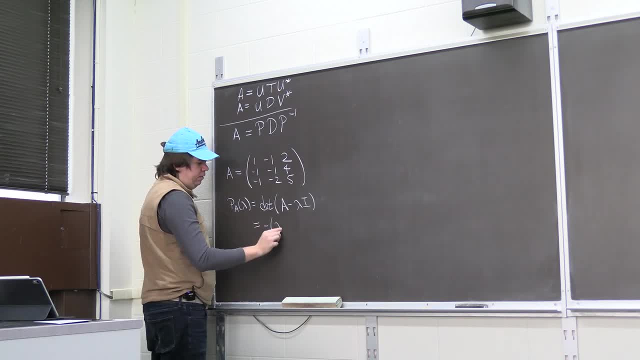 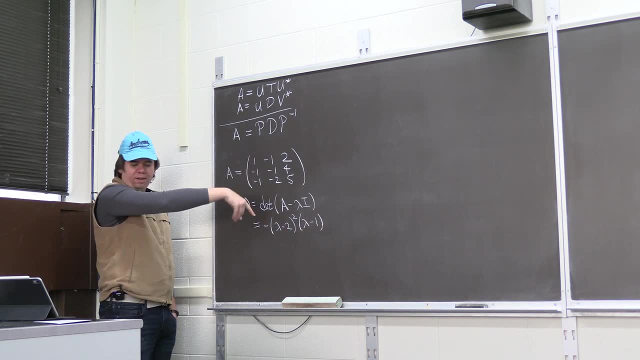 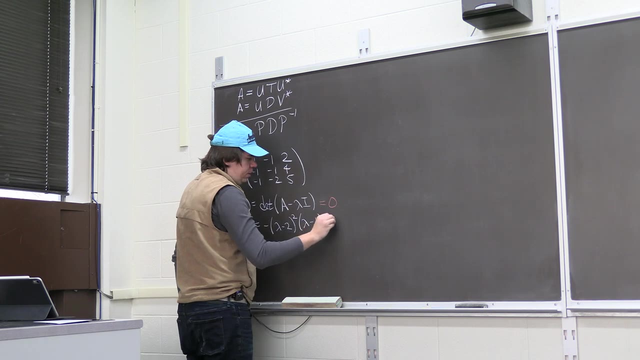 And if you calculate that it comes out to be negative- lambda minus two squared times lambda minus one- So you can calculate that out And then factor it and this is what you get. And so then, if we look, we want to ask: well, when is this equal to zero? 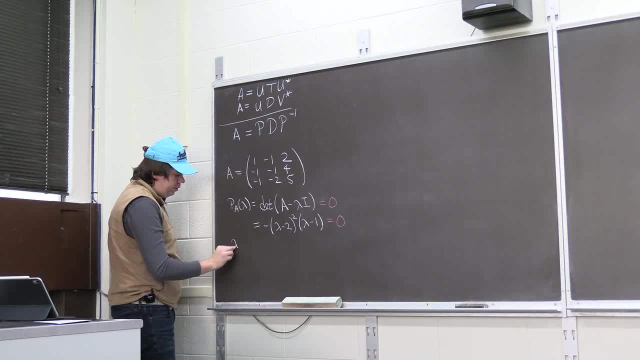 That's going to give us the eigenvalues. We recover that our eigenvalues are one and two. Right, Although the fact this is squared means that we could record the data that this one is equal to zero. one has an algebraic multiplicity of one. 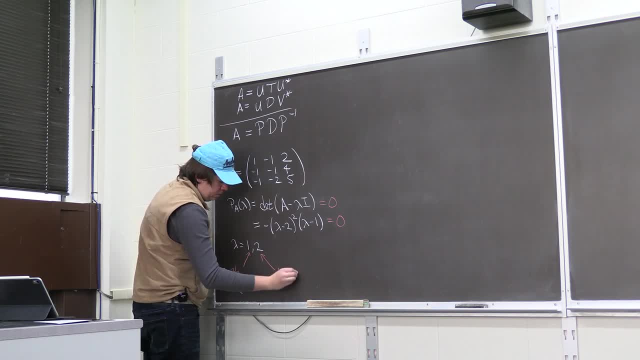 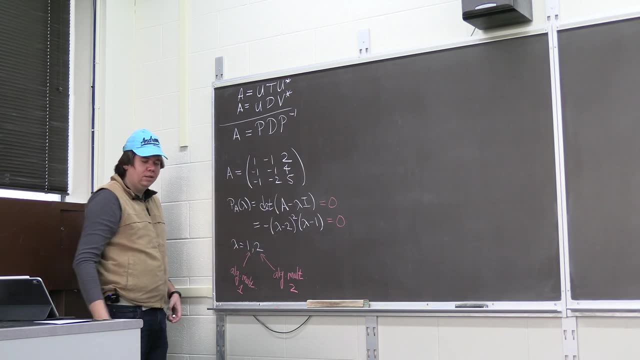 and this two has an algebraic multiplicity of two. Essentially, two is showing up twice as an eigenvalue, whereas one only shows up once as an eigenvalue. Okay, so now that I may remind you of this word: algebraic multiplicity. 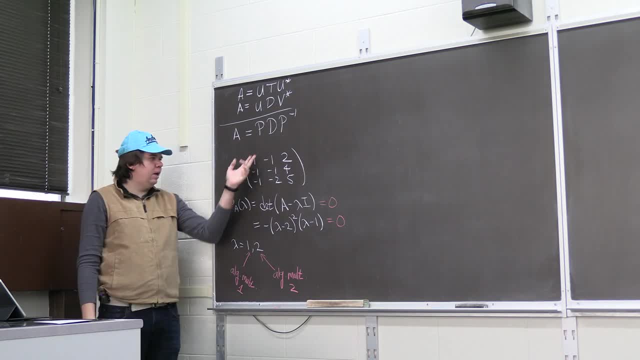 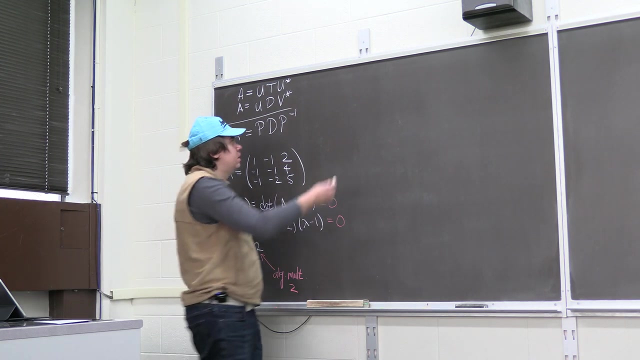 do you remember the criteria for when a matrix is diagonalizable? Something to do with this? No, so not quite. It's going to be when your geometric multiplicity equals your algebraic multiplicity. So let me remind you what I mean by geometric multiplicity. 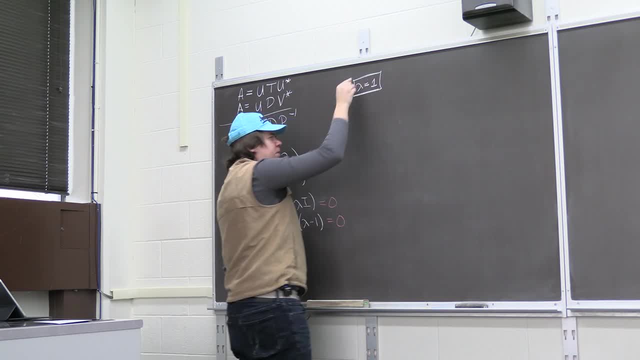 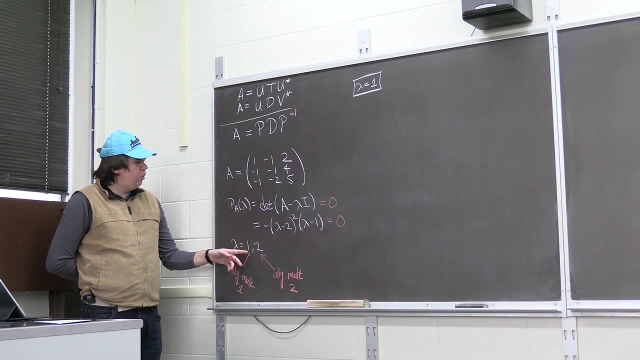 So if I look at the eigenvalue lambda equals one- I think this is something you probably saw in like an introduction to linear algebra course- If you look at the eigenvalue lambda equals one, we can look at this matrix: A equals one minus I. 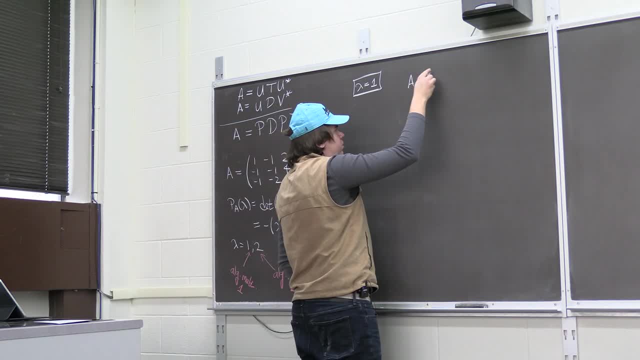 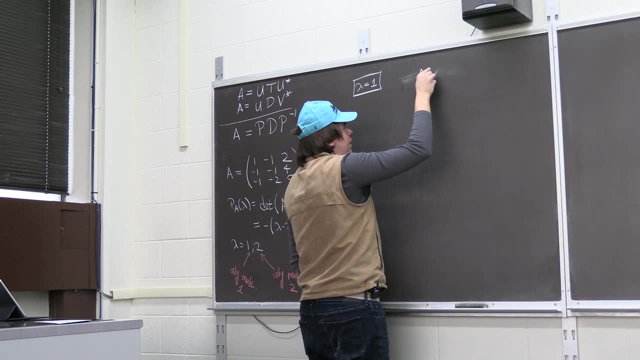 So where is this coming from? Well, we're interested in when is A equal to lambda I right? And so, in particular, we're trying to solve when is A times a vector V equal to your eigenvalue, times the vector V right? 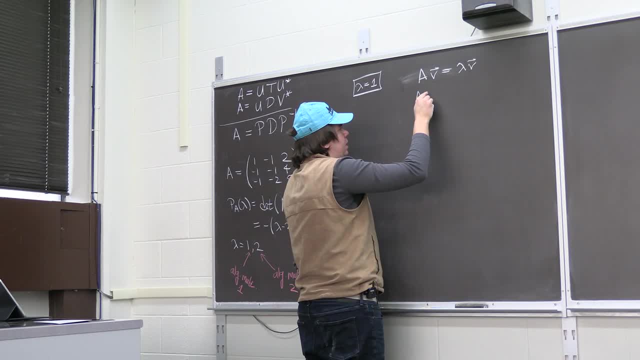 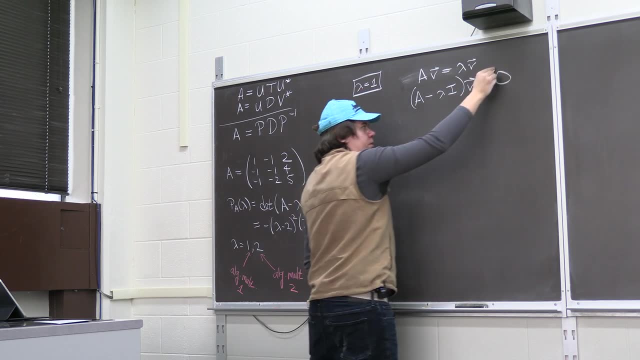 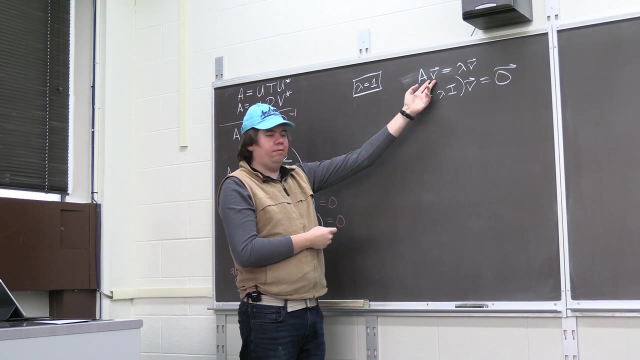 And you're like: well, that's going to be true when A minus lambda I times V is zero, right? Just factor out my V on this side. And so what I'm really interested in to find my eigenvalues is: I'm trying to find. 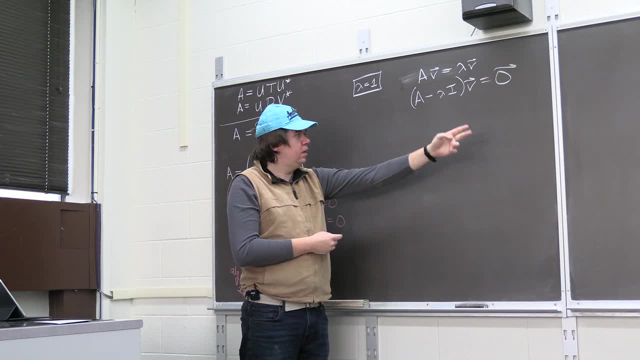 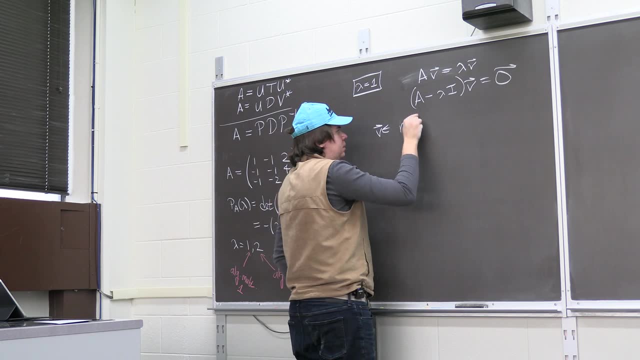 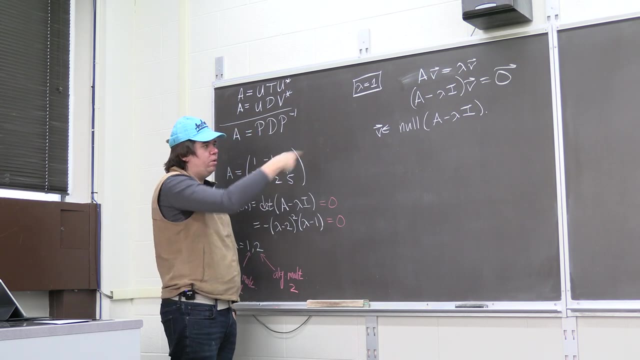 all of the vectors that you multiply this matrix by to get zero, And those vectors are, when you multiply them right, called vectors in the null space. v, we'd say, is in the null space of a minus lambda i. So if you want to calculate the null space, for example for lambda, equals. 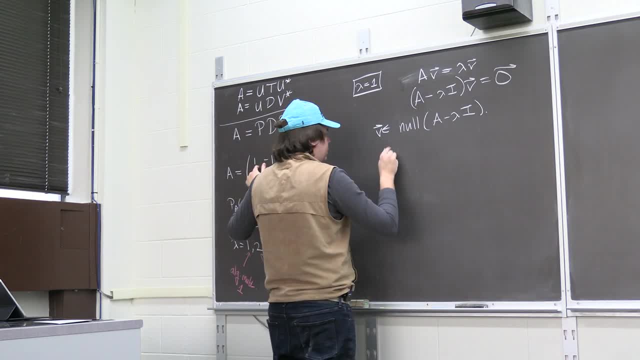 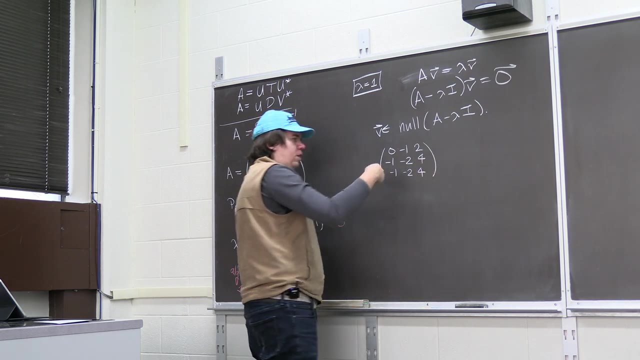 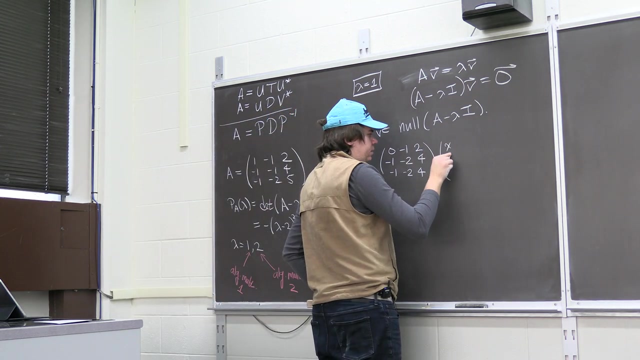 one. our matrix is just becoming zero minus one. two minus one minus two, four minus one minus two, four. So you're trying to calculate this null space, That is, we're trying to find vectors, v, vectors of the form, say, x, y, z. so this comes out to be zero, zero, zero. 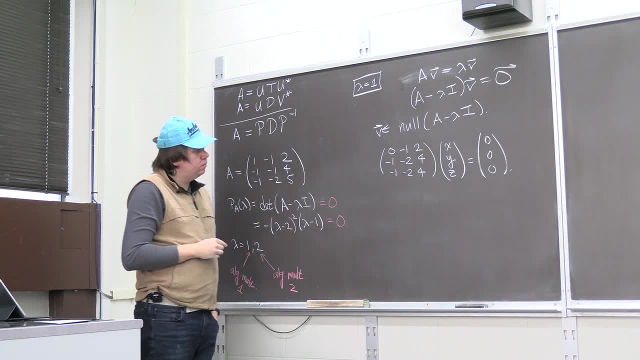 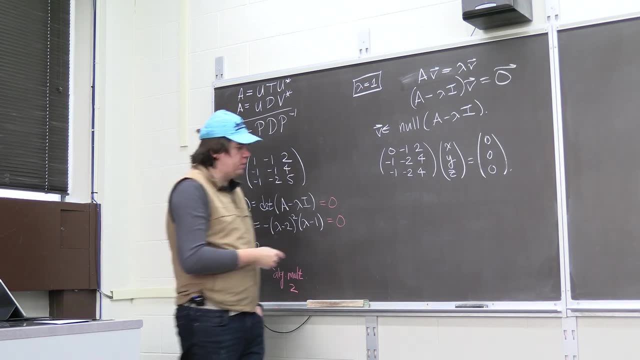 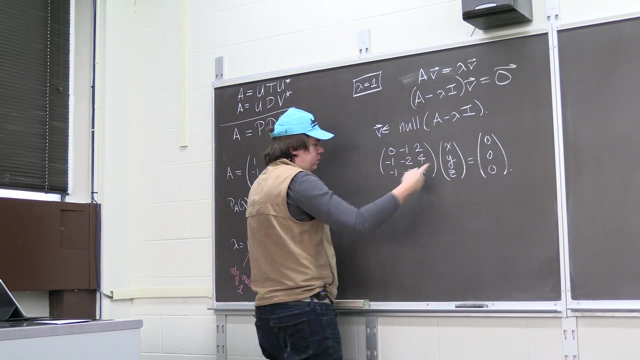 All right, so you might look at this and does anyone see like a solution for what x y z could be? What's one possible solution for x y z? Zero, two and one? Great one solution for v is you could set your v to be zero, two and one, So like plug. 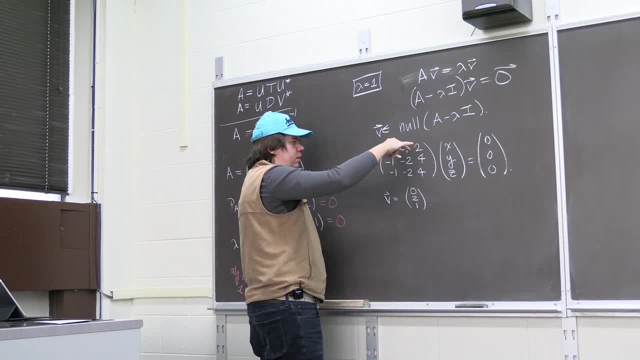 that in that gives you the first row, vanishes the second row, you get two times this and one times this and notice the second guy is always negative twice the first. the third guy is negative twice the second. so that's always going to work. So that's great. 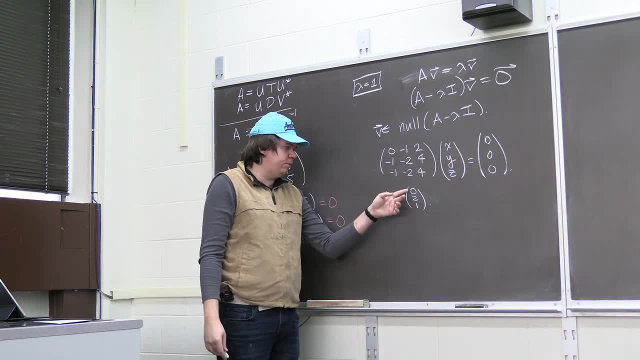 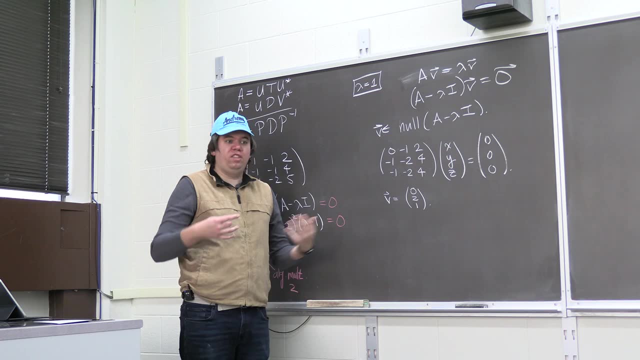 Are there other guys? Well, yeah, you can scale this by whatever you want. you could have done zero four, two or zero six, three. that would have also worked right. But then you're like: well, is there anything else that's linearly independent from this v, Or is this the only? 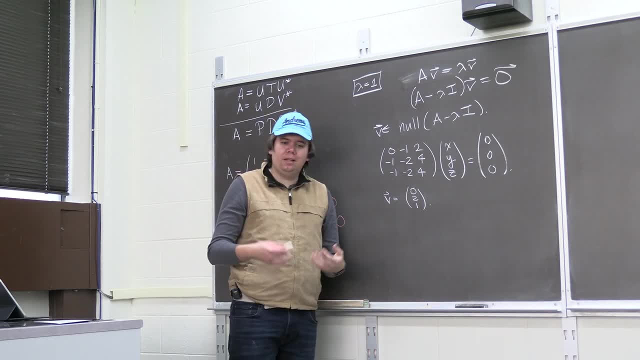 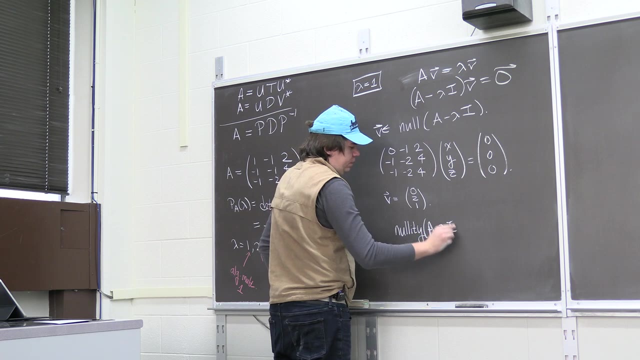 is it only just scalar multiples of this guy? And that's now asking a different question. You're now asking what is the dimension of the null space, and that's what we call nullity. The nullity of some vector is just asking me for the dimension of the null space. How? 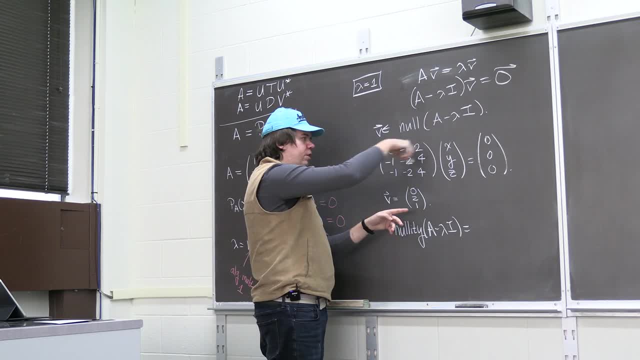 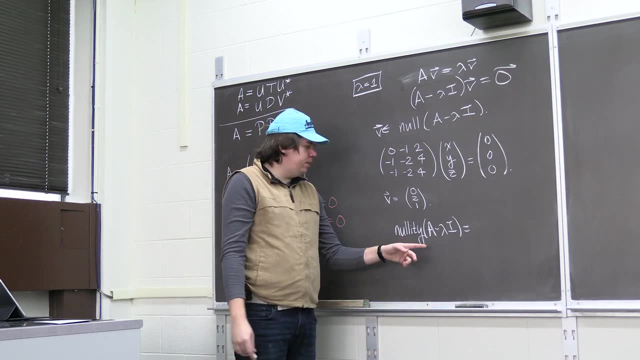 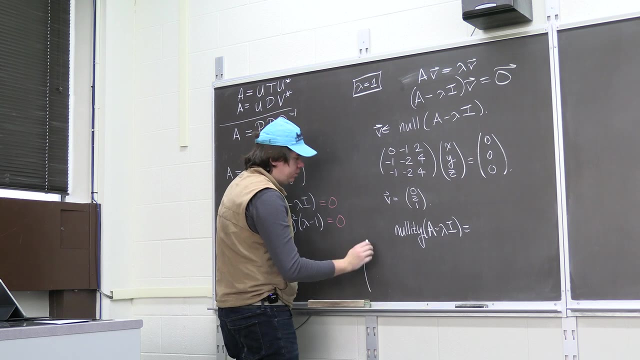 many linearly independent vectors are there that are in this null space. How do you find that? Well, one way you can find it is by remembering that the nullity is preserved under row operations, So you can row, reduce this matrix. You can have some matrix like zero minus one, two. 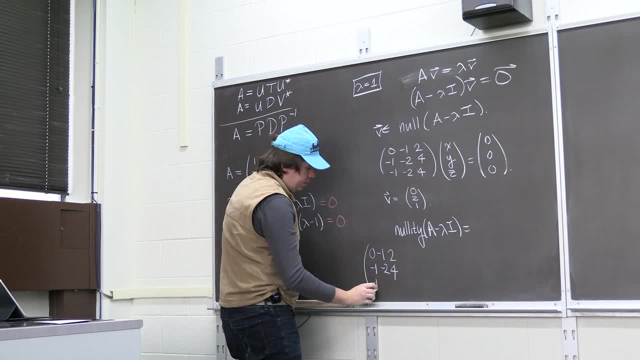 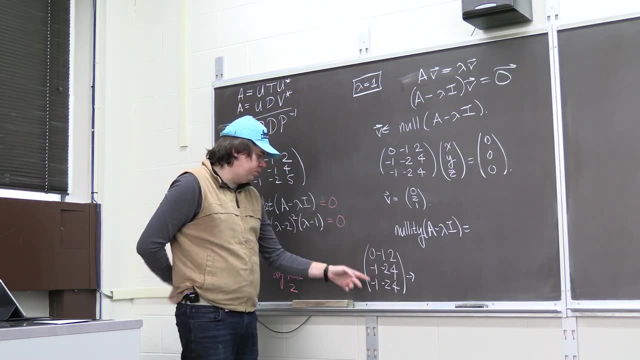 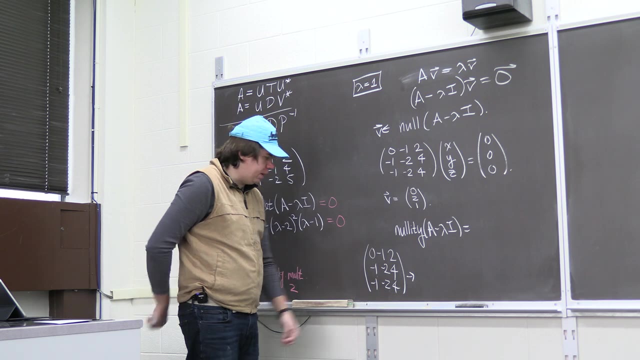 minus one minus two four minus one minus two, four. and you just row, reduce them And so you're like: oh, these bottom two guys are the same. So if you track a copy from the second row, from the last row, you get zero on the bottom now. So now I'm going to get 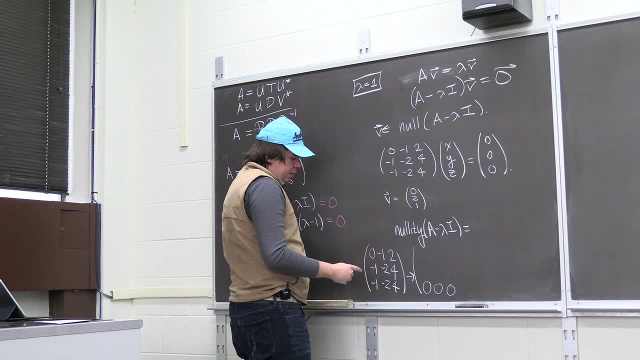 all zeros on the bottom And then you're like, oh, I'm going to get zero on the bottom. And then you're like, oh wait, this guy is like two copies of the row under him, Like if I subtract two copies. 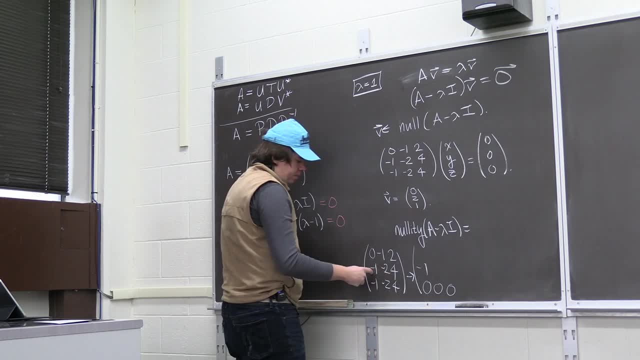 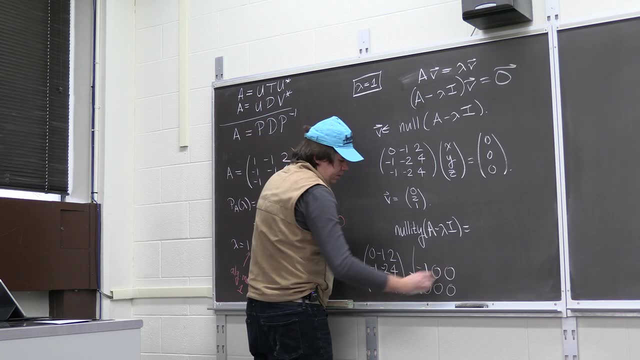 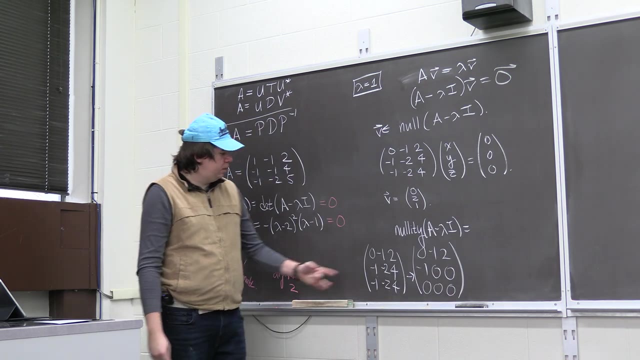 of the first row from the second, my negative one remains negative one, But minus two, minus two copies of this gives me a zero, And four minus two copies of two gives me a zero. And then on top I still have zero minus one, two. So it's like, okay, the nullity of this. 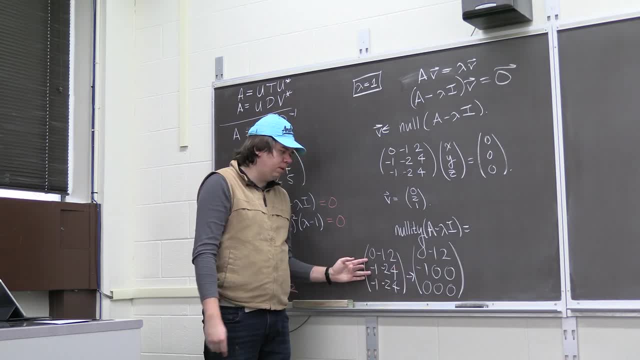 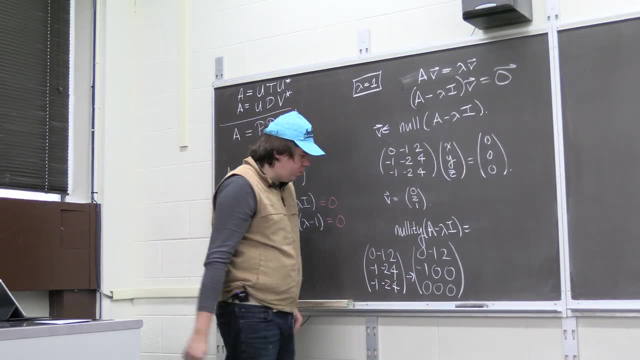 matrix is the same as the nullity of this matrix. That is, the dimension of this null space is the same as the dimension of this null space. This is row reduction, And then you can simplify things a little more if you want. If you want to like, multiply this by. 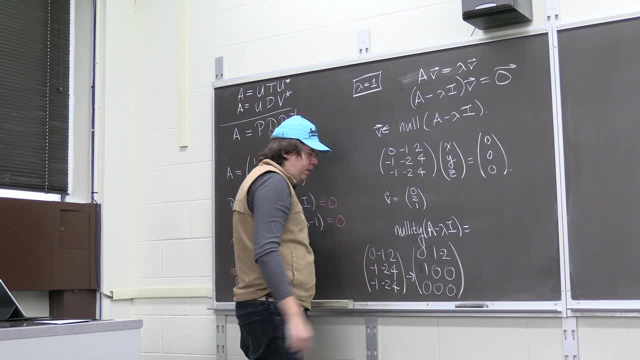 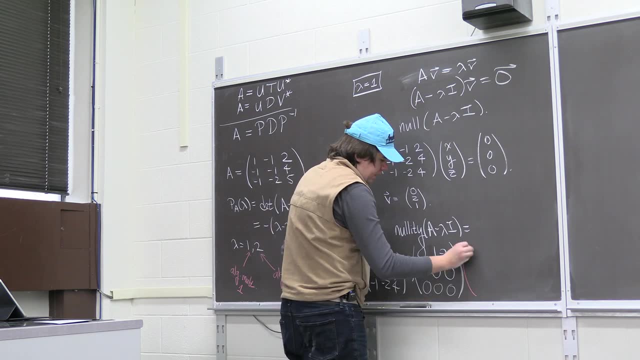 a negative one, you could. If you want to multiply that by a negative one, you might. But then it's just like sit down and think, Like what is the nullity of this If this is timesed by x, y, z to give you zero? what does that mean? Like what has to be true of. 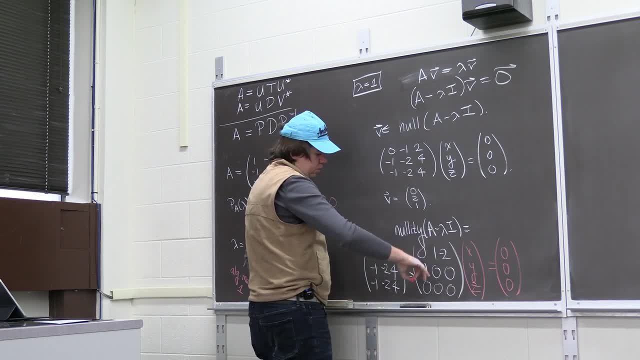 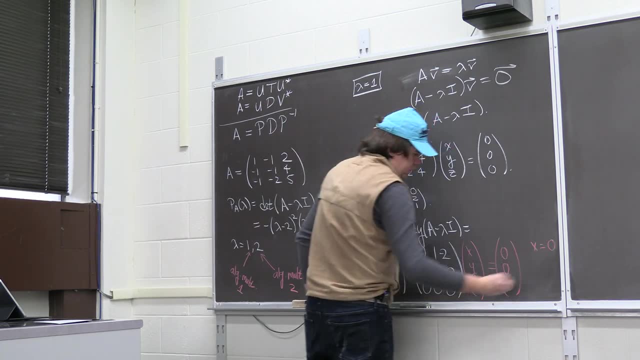 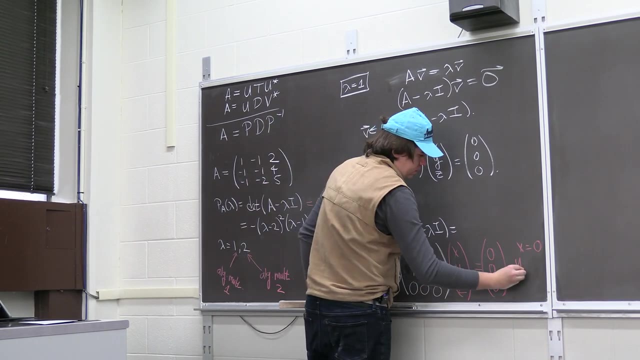 x, y and z for this to come out to be zero. And you're like, well, this second. multiplying the second row tells you x has to be zero. And then, multiplying the first row tells you that your y equals two z. And then your last. 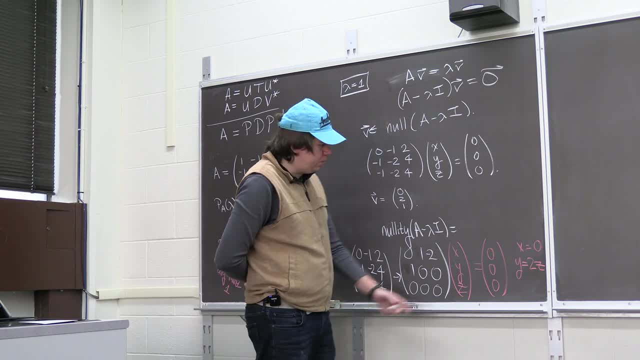 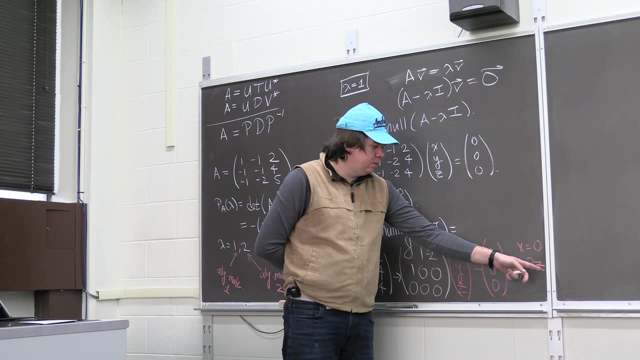 row doesn't give you any constraints, You just have zero, zero. Then how many degrees of freedom do you really have? x is locked in. It has to be zero. Y is determined by whatever z is. So the moment you determine C. 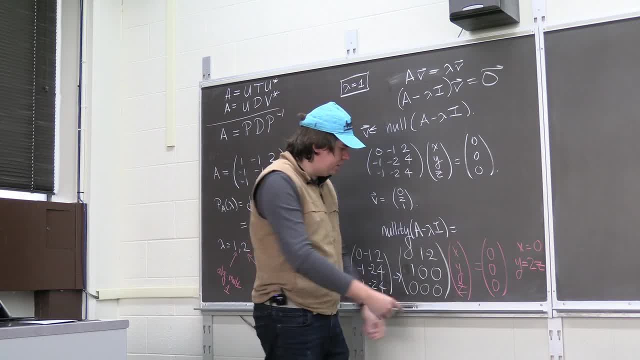 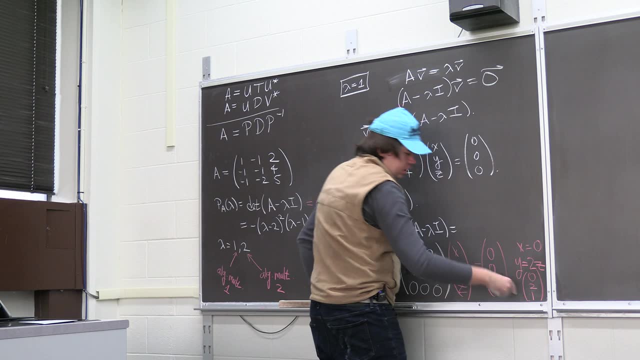 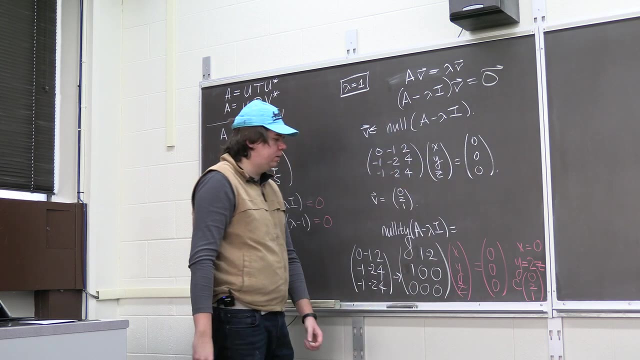 you also determine X and Y, right? So this is saying that this null space is just guys of the form zero two one Linear combination. multiples of this Scalar: multiples of zero two one. So multiples of zero two one. 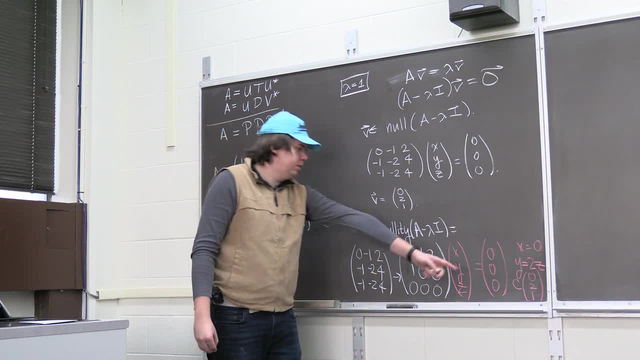 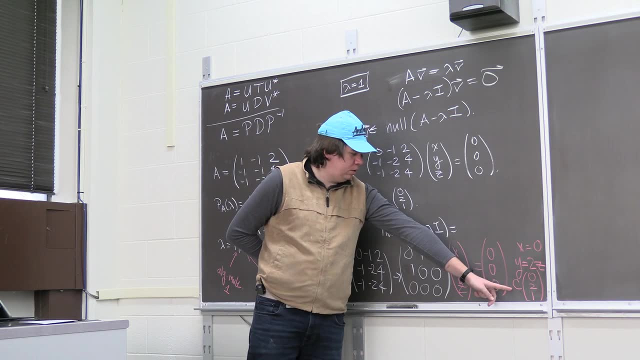 Now, that is not gonna be the same as well. okay, this is exactly the same as what we just had, but the point is, all I'm interested in here is just the dimension. This is dimension one. It's just multiples of a single vector. 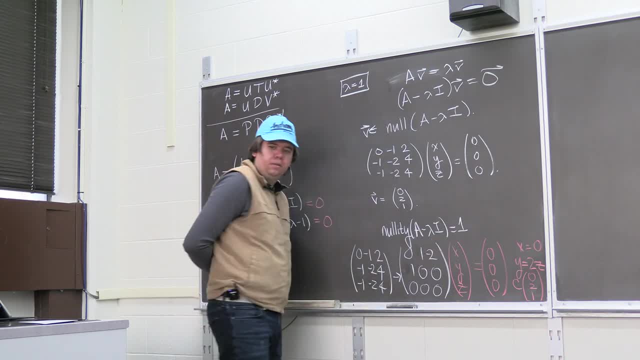 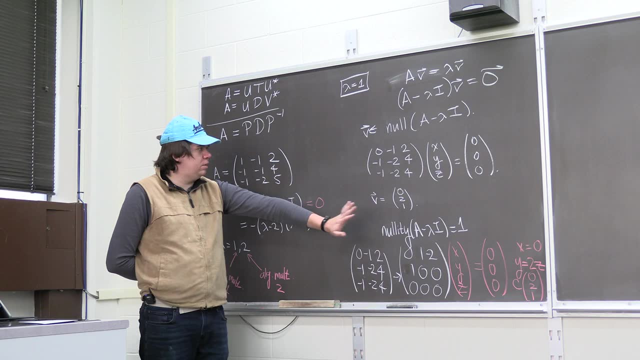 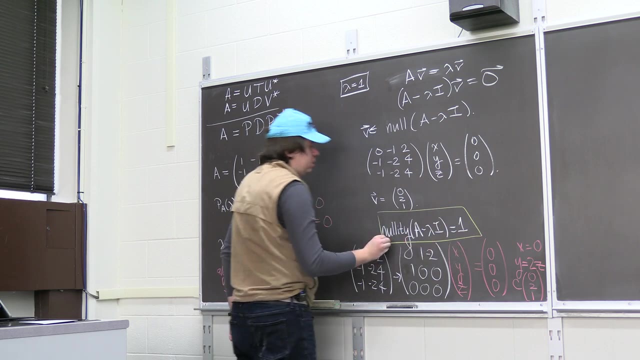 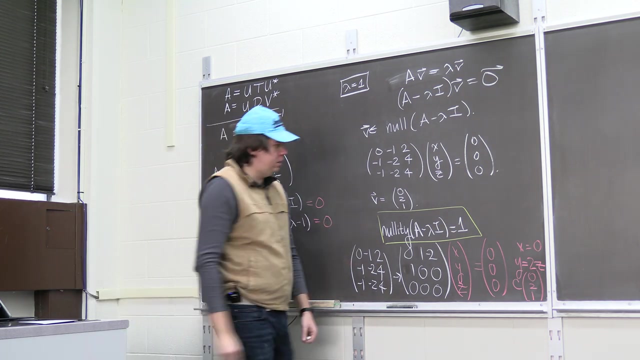 and so the nullity is one. Okay, great, There's my nullity, the dimension of this null space, And what I wanna highlight is this: nullity for one was the same as my algebraic multiplicity. So your nullity is sometimes called: 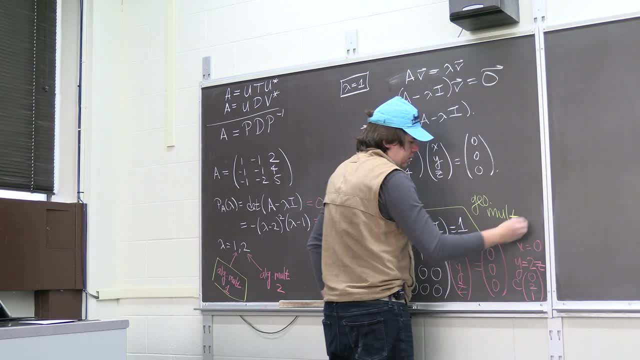 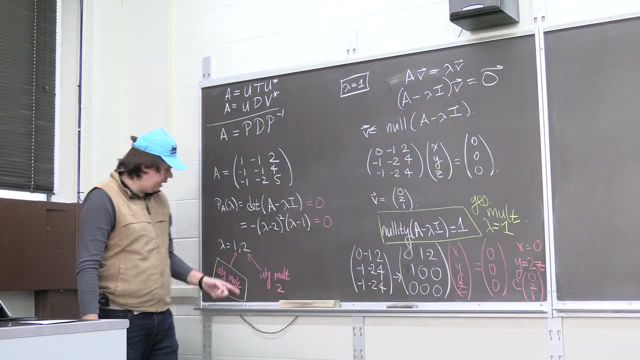 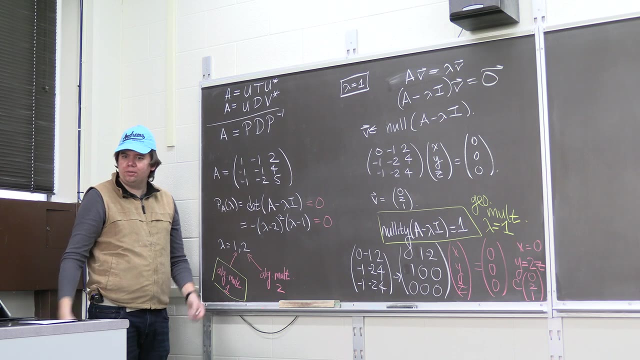 your GMT. It's a geometric multiplicity for your eigenvalue, for the eigenvalue lambda equals one, And in this case my geometric multiplicity came out to equal my algebraic multiplicity. Does this seem vaguely familiar at all? Did you guys do a little bit of this in your last course? 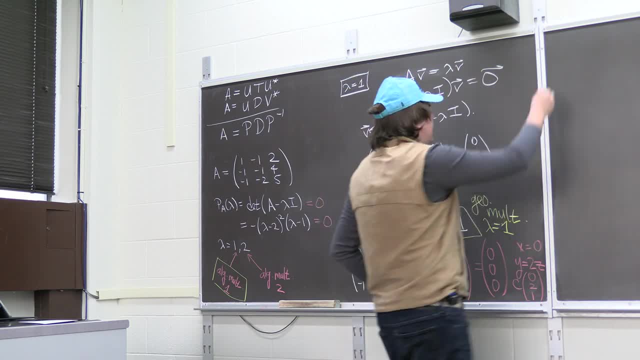 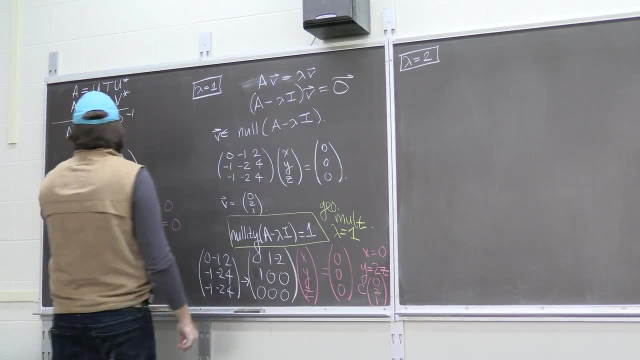 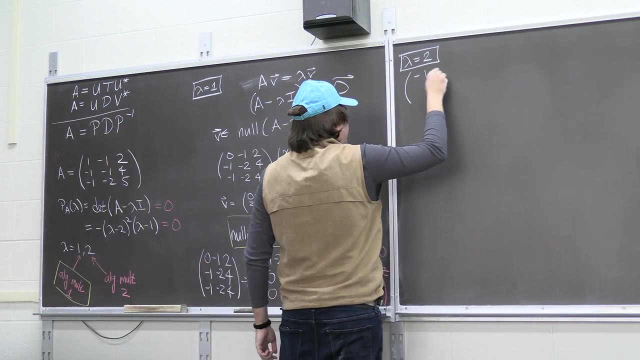 Okay, well, now let's investigate the case of my second eigenvalue of lambda equals two. At lambda equals two, I'm now gonna be looking at my matrix A minus two identity. So that's going to give me the matrix minus one. 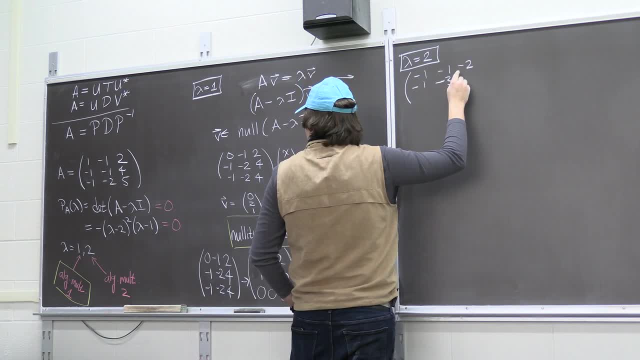 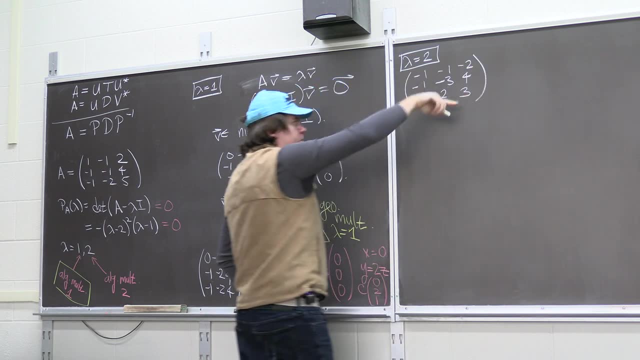 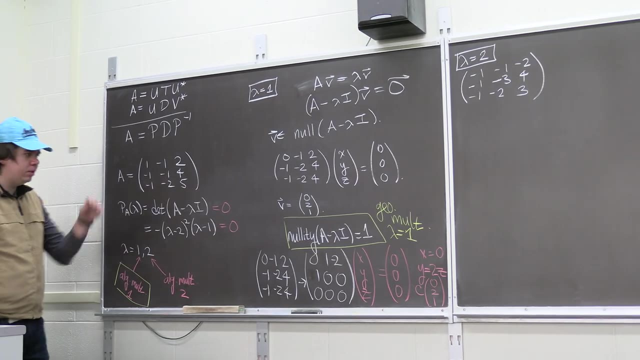 This second row, I get a minus three in the center. Everything else is the same. And then the last row: the bottom right value moves from five to three, subtracting two times the identity. Okay, so let's play the same game, right? 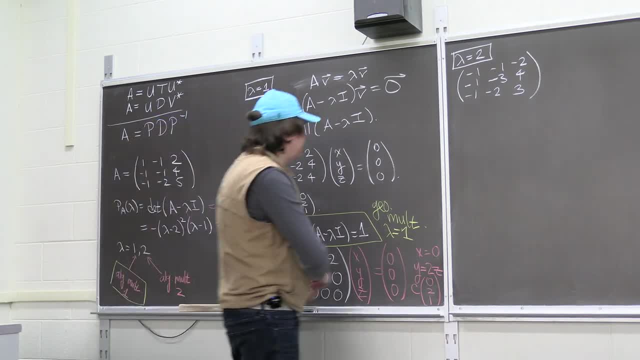 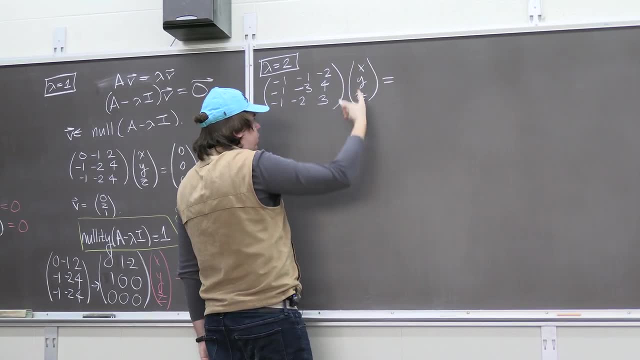 It's like, ultimately, at the end of the game, at the end of the day, I'm gonna wanna know, like, what are the full set of solutions to this, or what is the dimension of the space that contains all vectors that give me this? 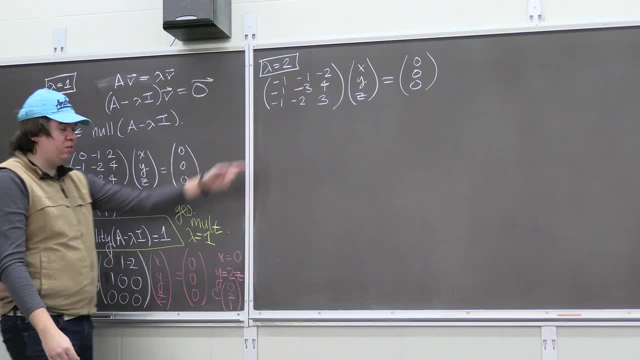 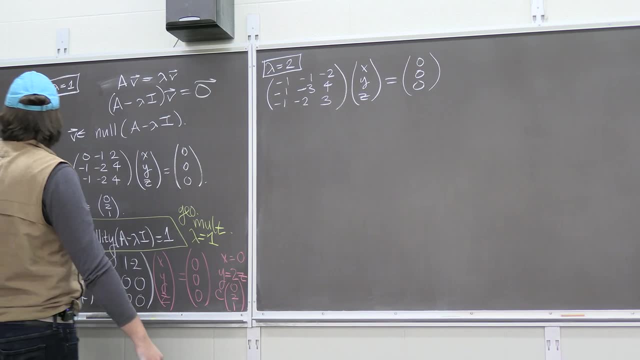 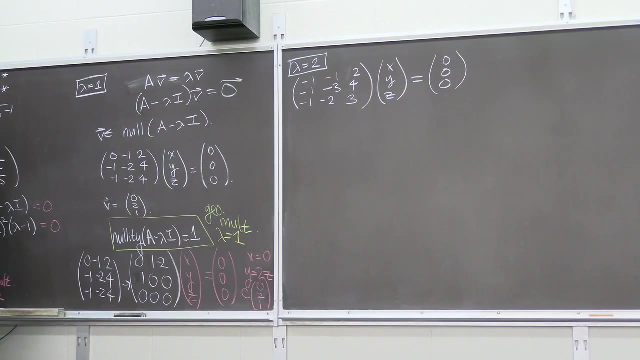 It's like, maybe by looking at it, you can just see one such vector already, Like can you see one? Ah, that two is positive. Maybe now you can see one, One, one, one, right. So like one example of a vector. 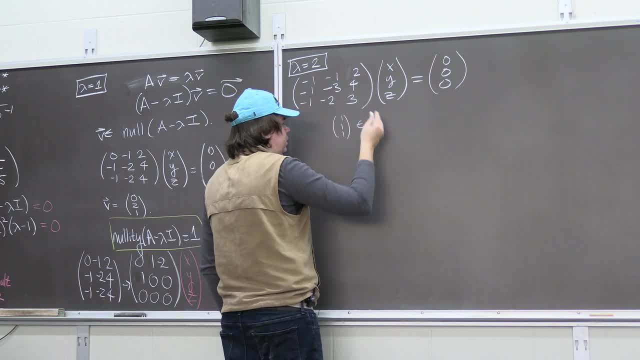 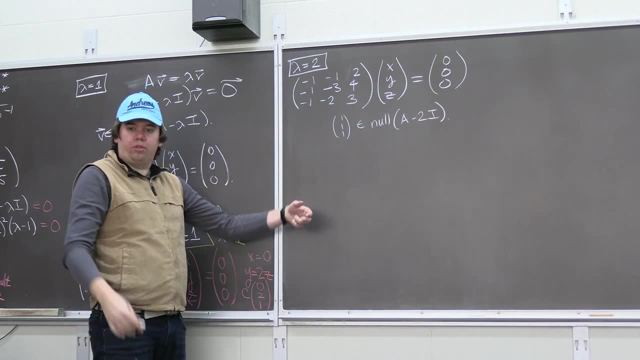 that would be in your null space would be one, one, one. That's one such example, that's in your null space, of A minus two I, But there are other ones: two, two, two, three, three, three. Okay, so all scalar copies of this. 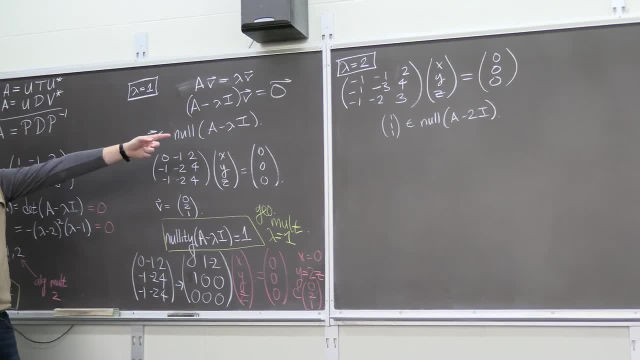 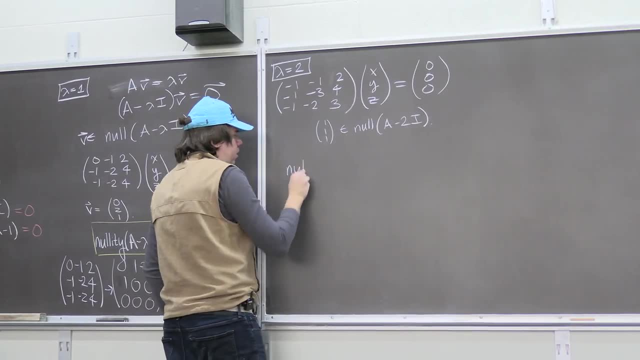 Is there another one in there, Something linearly independent from one one one? Well, let's check, Let's try and calculate the nullity of this guy. So I'm interested in calculating what is the nullity, What is the dimension of the null space of A minus two? I 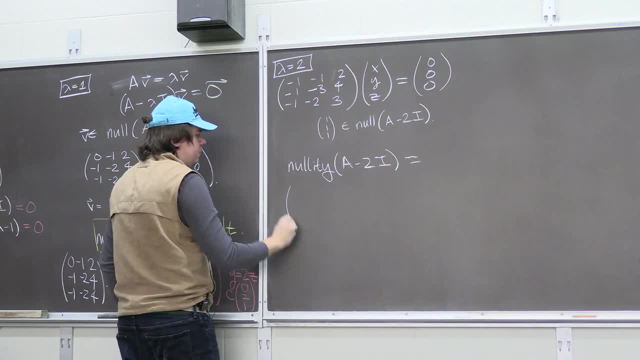 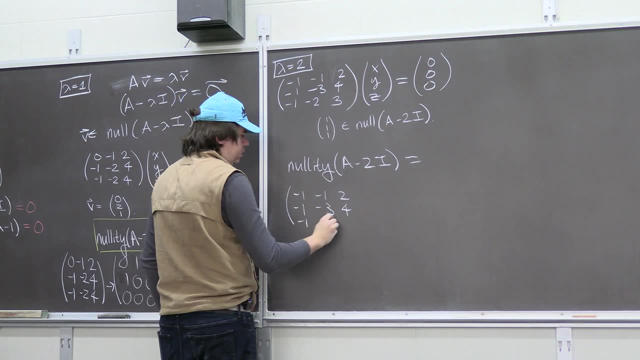 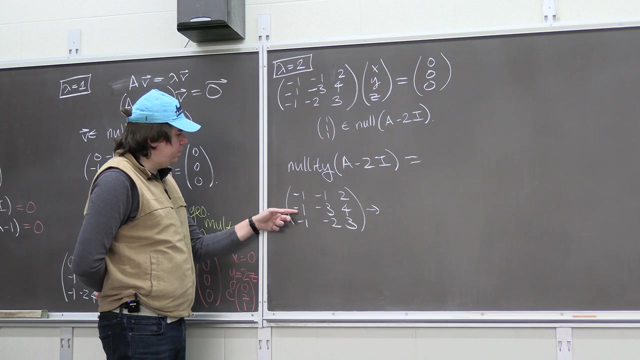 And so to do that, I'm just gonna do row operations on this matrix And you're like well check it. This second matrix is just the sum of the first and the last, So lots of ways you can play around with this. 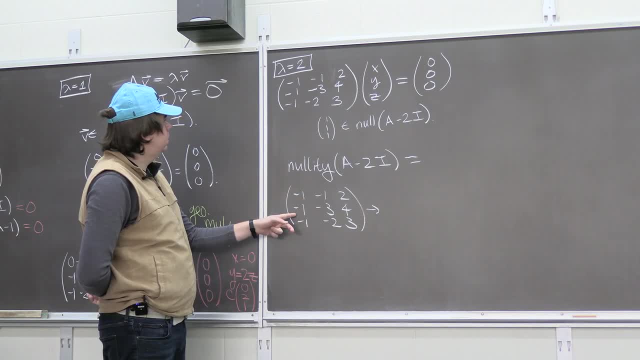 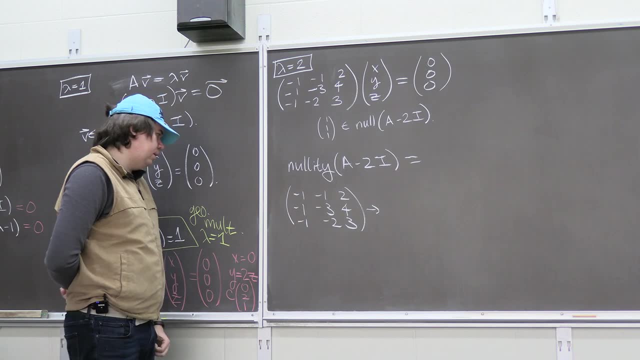 One way is: oh, that's not quite true, is it? No, it's not the sum, This guy and this guy's the sum. Oh no, he's not even close to the sum. Okay, so that was a lie. 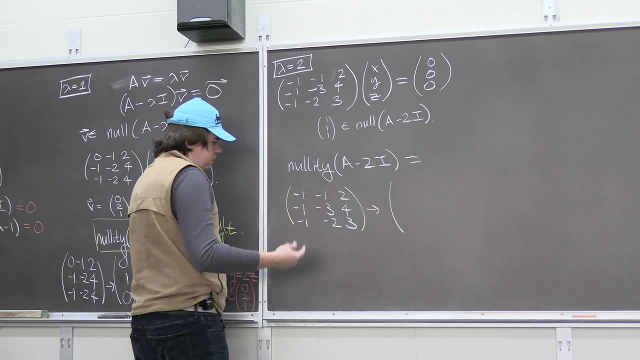 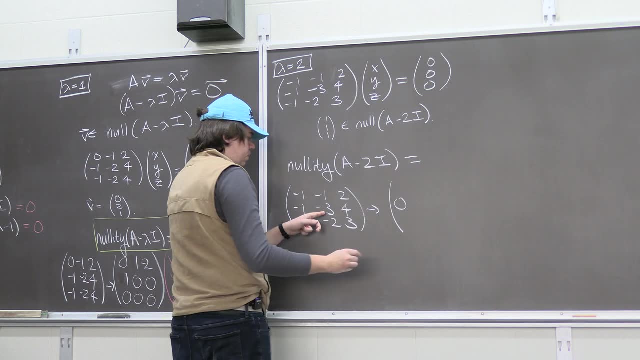 Ah, let's just subtract the rows from each other and see what happens. Let's subtract the last row from the second row, So he's now going to be zero minus one one. Let's subtract the first row from the last row. 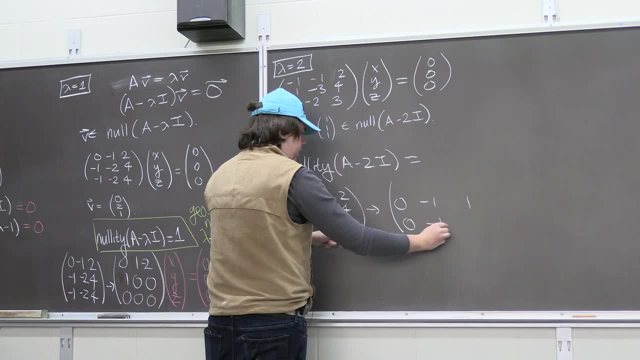 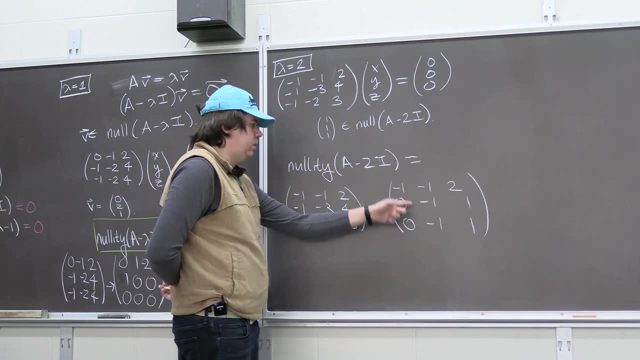 He's now going to be zero minus one one and minus one minus one two, And then you're like: okay, well, that bottom row is now a duplicate of the guy above him, So if you subtract him from the guy above him, 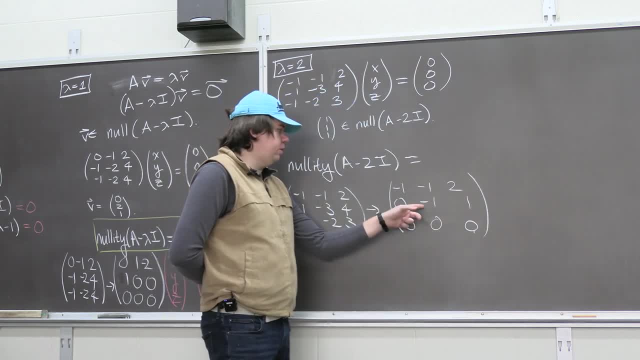 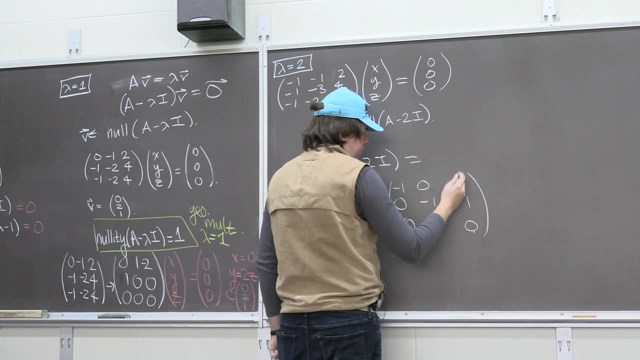 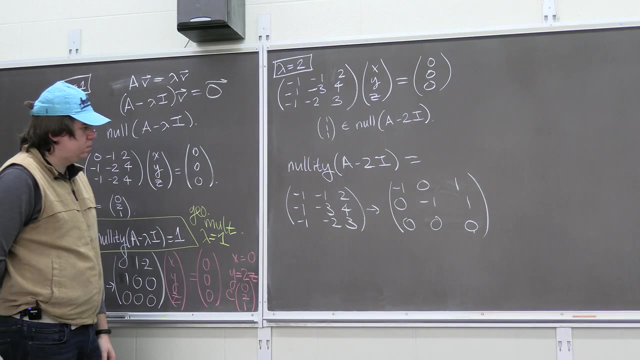 you get zero, zero, And then you can subtract the second row from the top row. So minus one minus minus one is zero, And two minus one is one. Well, this is looking pretty good. So, like what's the nullity of this guy? 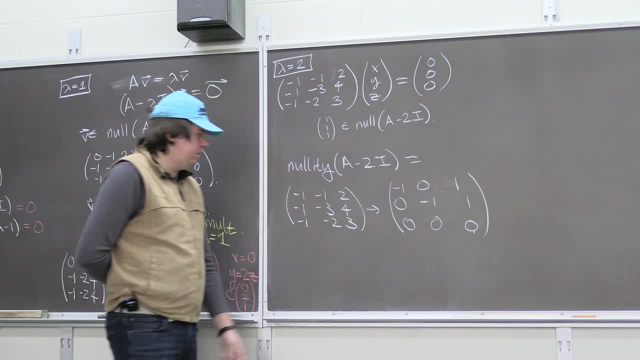 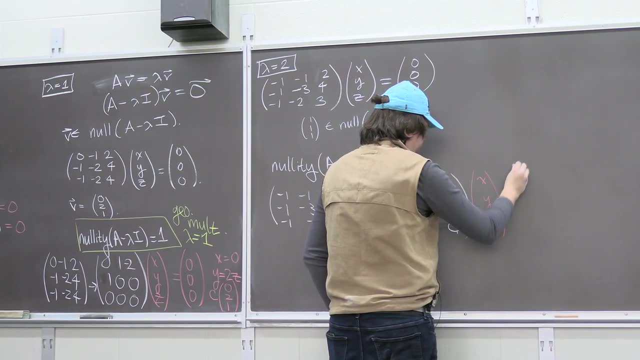 Huh, Yeah, it's one just like before. If you want to like, like, convince yourself, you're like okay, if I have X, Y, Z and I want to know when it comes out to be zero, zero, zero. 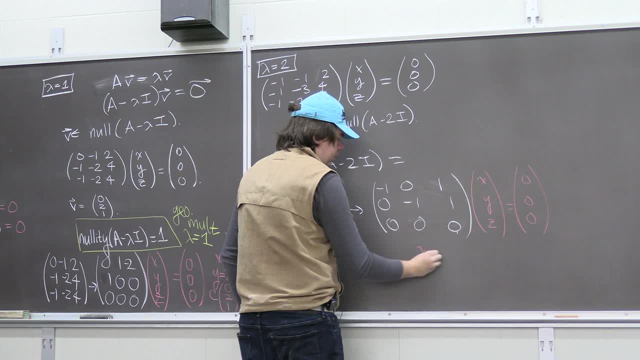 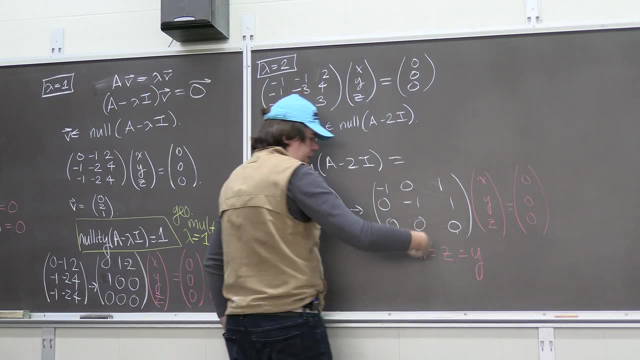 this first guy introduced the constraint that my X must equal my Z, But then this condition gives you that Y is also equal to Z, And so your X, Y and Z must all be equal to each other, And so you only have one degree of freedom. 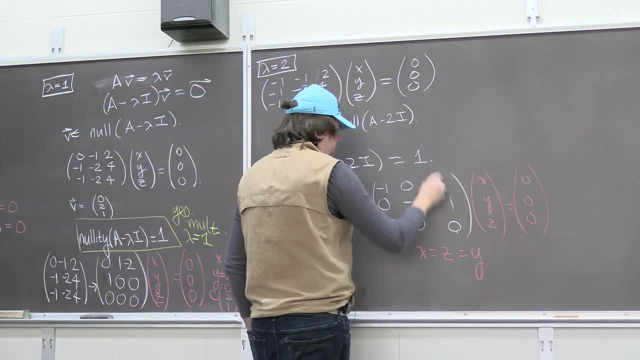 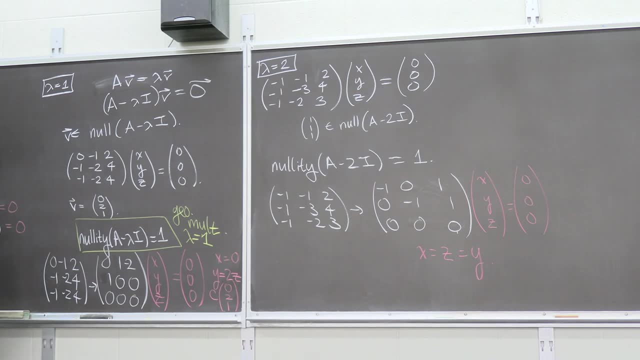 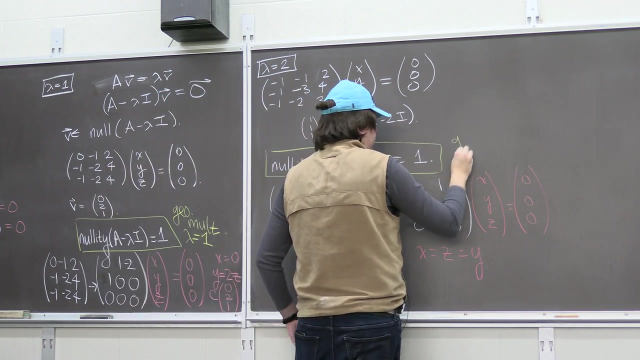 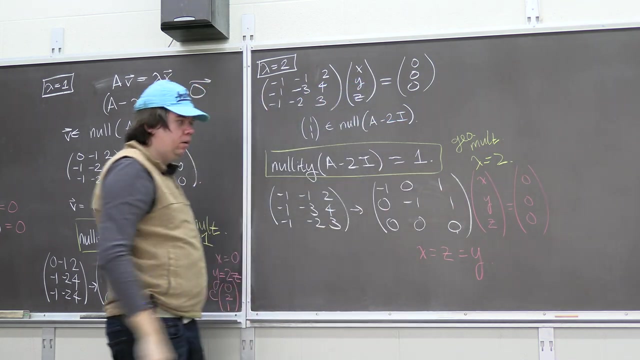 And so your nullity has dimension one. It's just all scalar copies of one one. one, right, Okay, Cool. So my geometric multiplicity for the eigenvalue two is one. Uh-oh, My algebraic multiplicity was two. 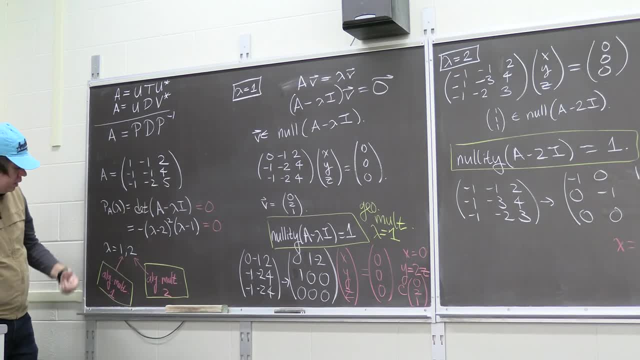 It's not a problem. It turns out in general- I mean, this is something you proved in your last course, If you think back- that your geometric multiplicity is always less than or equal to your algebraic multiplicity. But it also turns out- it turns out that you know. 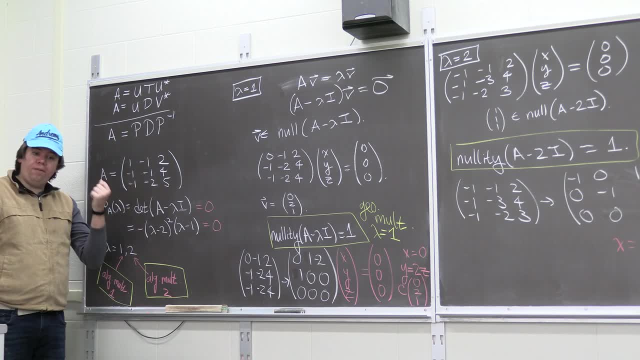 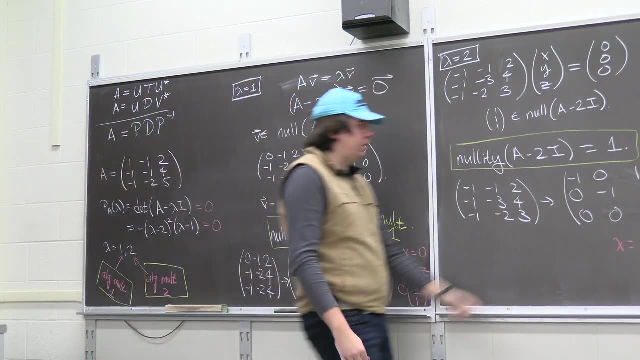 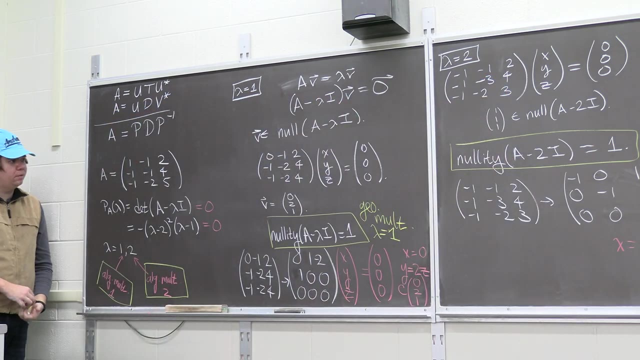 it also turns out that you're able to diagonalize if, and only if, your geometric multiplicities equal your algebraic multiplicities, And it's because we came up short here that we're not able to diagonalize this matrix Right. So so there's no way to diagonalize this. 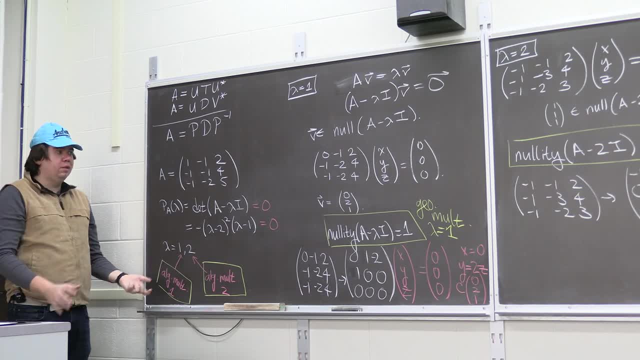 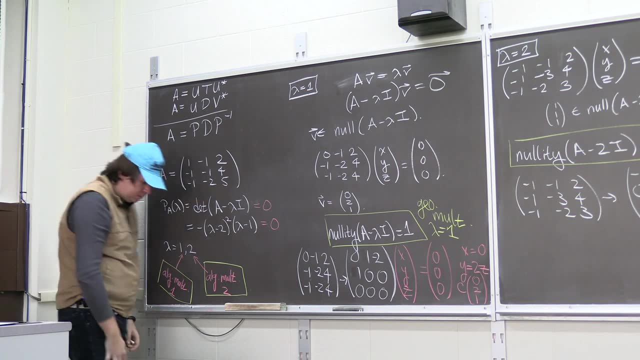 Not even over the complex numbers You might be like, is it just because you know sometimes you have real matrices and the eigenvalues are complex? but it's like, even over the complex numbers you can't, you know you can't- diagonalize this. 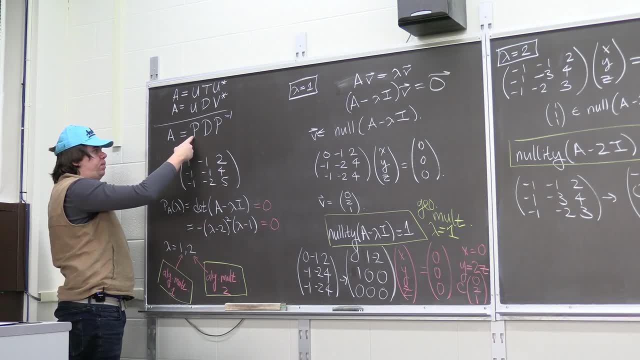 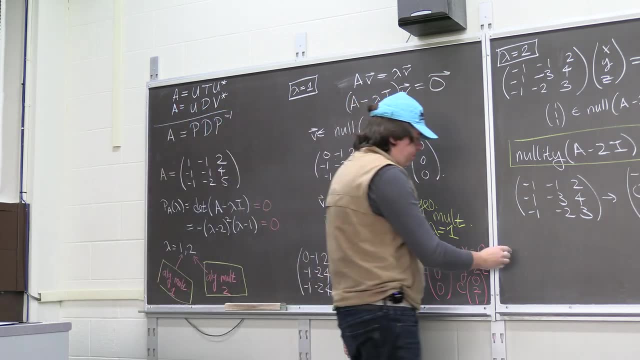 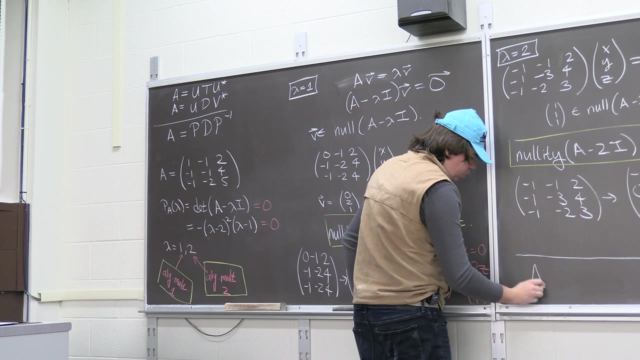 So we cannot write A as some PDP inverse. So our goal for today is we want to start asking the question. we're going to be spending this week talking about this. Well, is there some way that, given any square matrix A, so given any? 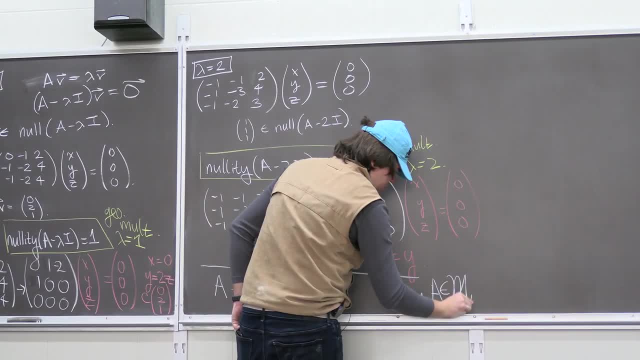 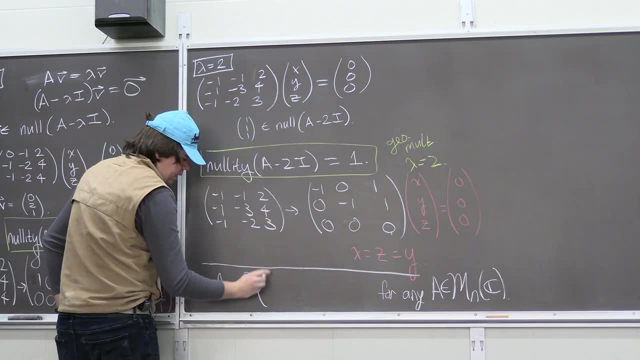 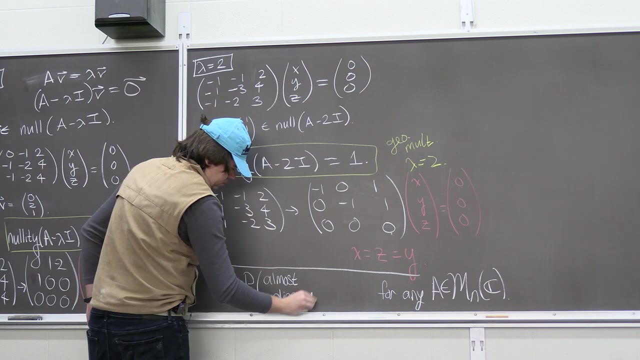 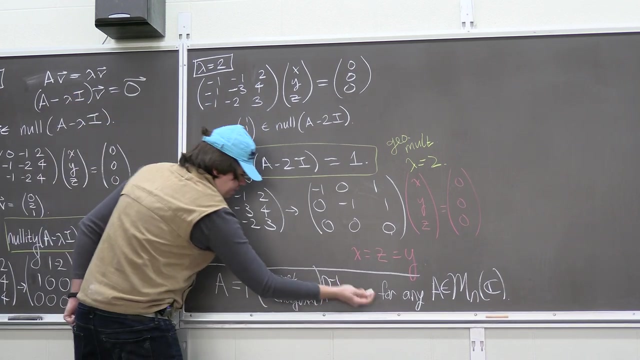 square matrix A. let's say we'll do it in general, of the complex numbers that we can write A as P times something almost diagonal times P inverse. So can we do a change of basis not to a diagonal matrix- we just said we couldn't- but to something almost diagonal? 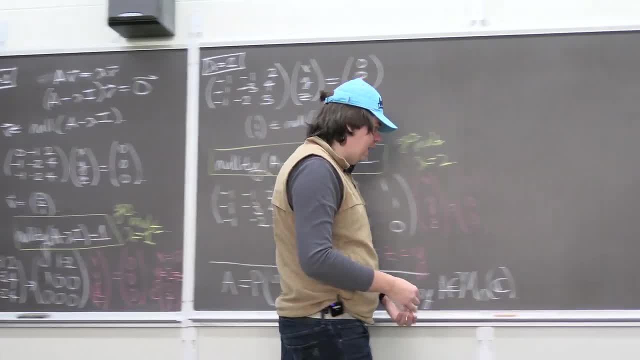 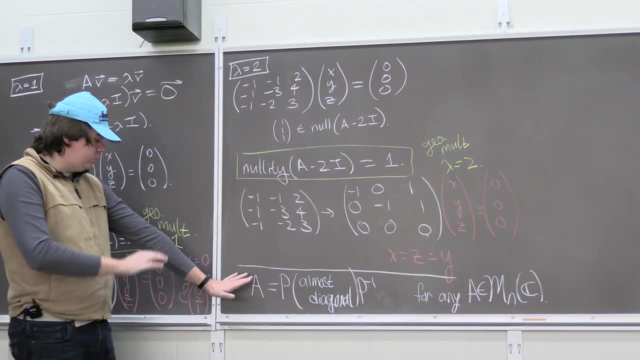 And and yes, we can right This is. this is what we're going to do. This is our last, So this is going to be our last decomposition results. We're going to see in this class the last way of representing A as for any square matrix A. 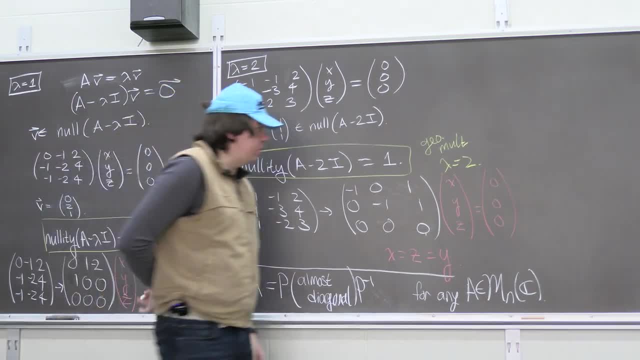 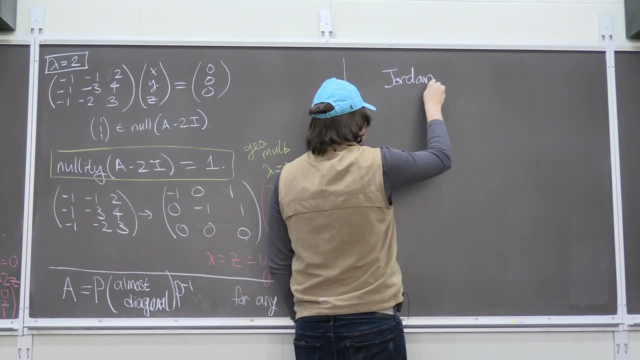 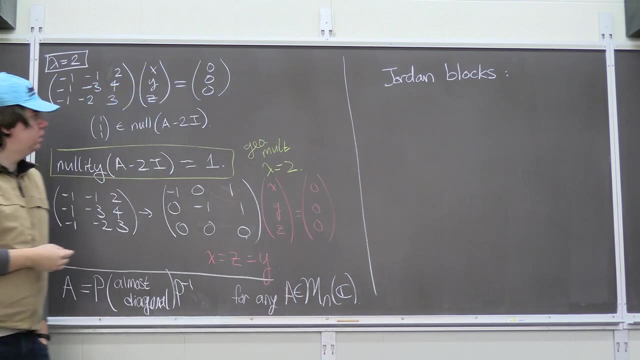 can be written as well, a special form that we're about to talk about. So first let me show you some terminology. We're going to be talking about Jordan blocks, So we're building up to a Jordan decomposition And- and here's the idea of a Jordan block- 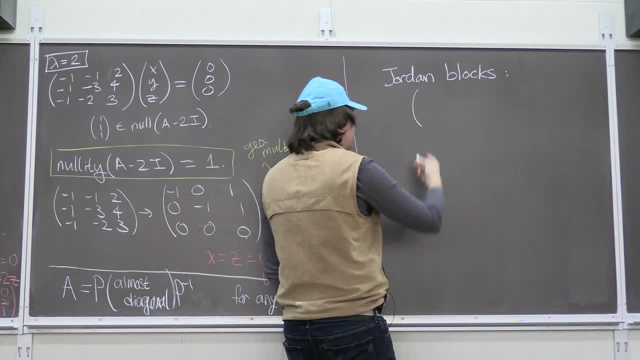 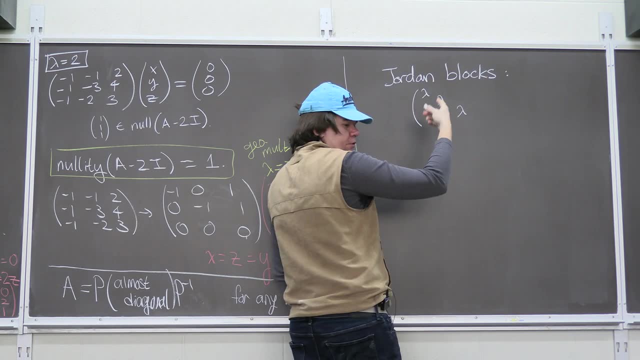 A Jordan block is a matrix that has some entry along the diagonal. I don't know what it is, I'll call it a Lambda. So Lambda, Lambda, Lambda, however many you have, And then you have ones on the super diagonal. 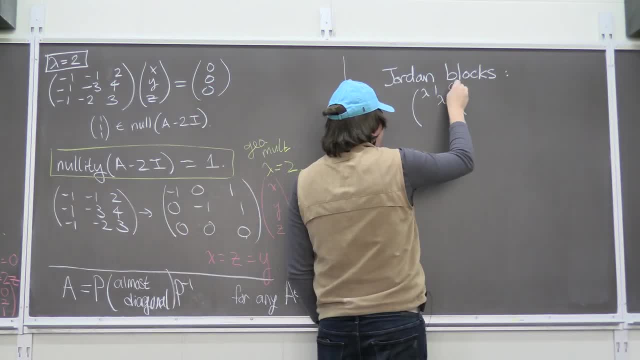 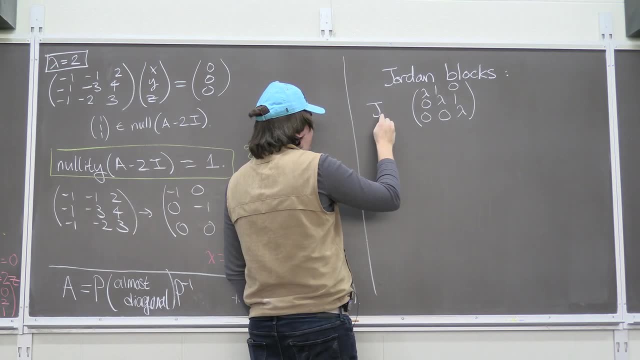 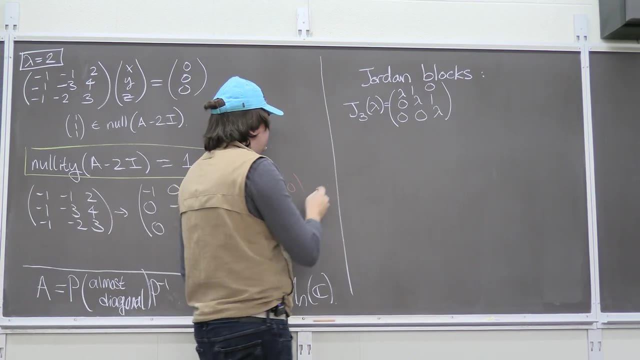 on the diagonal, above the diagonal and zeros everywhere else. So this would be an example of a three by three Jordan block with diagonal value Lambda. Some Jordan blocks are very simple. You can have a one by one Jordan block with some value like three. 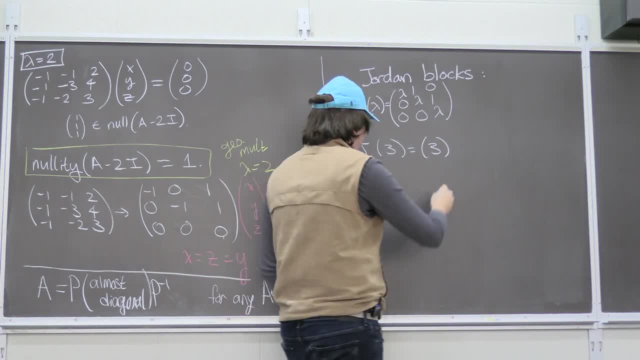 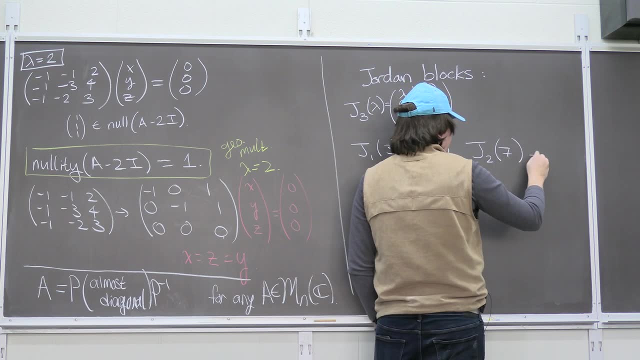 That's just going to be the matrix, with just three. right, If you want to have, let's say, a two by two Jordan block with the value- I don't know- seven, that's just going to look like sevens here and a one above it. 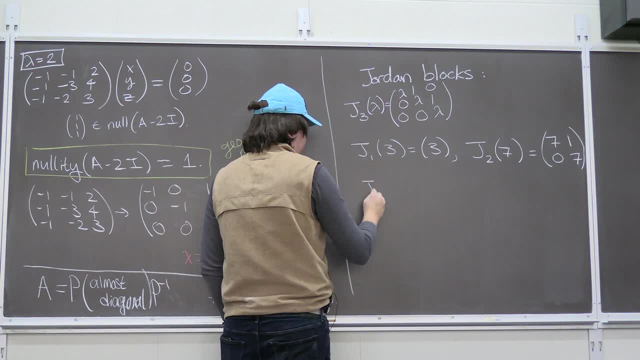 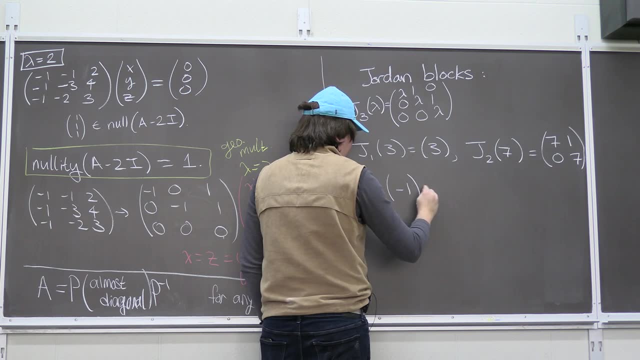 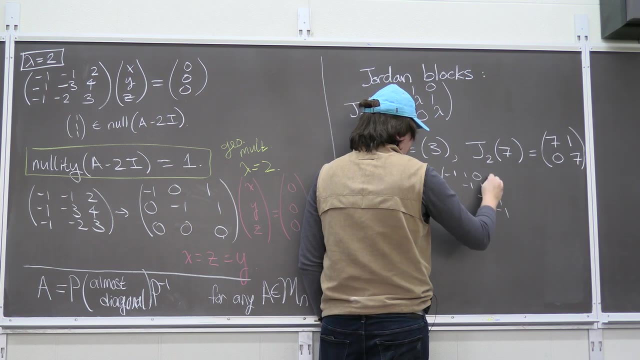 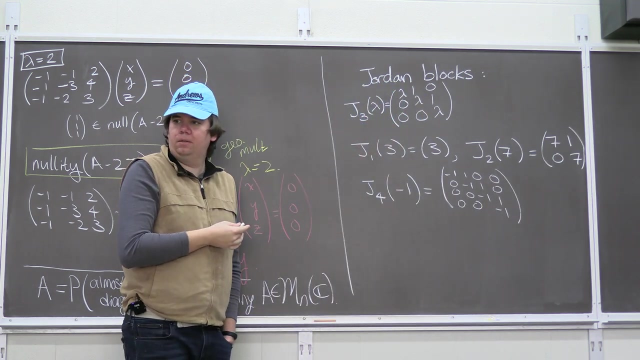 And if you want to have, I don't know, something more complicated, like a four by four Jordan block with some number like negative one, that's going to look like four copies of negative one and ones above them. Yeah, get the idea of a Jordan block. 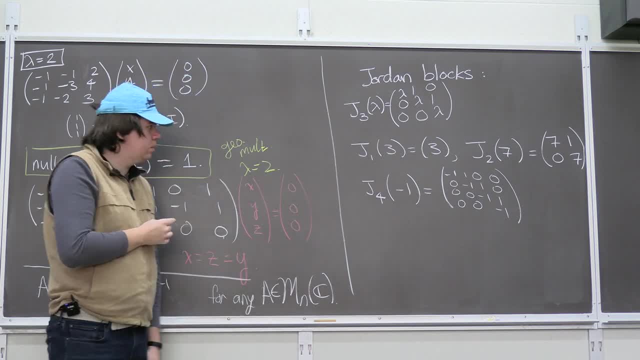 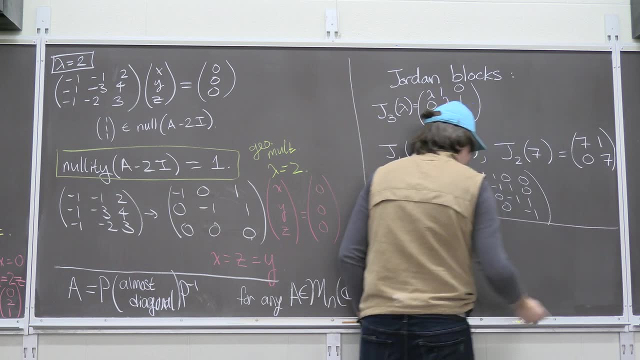 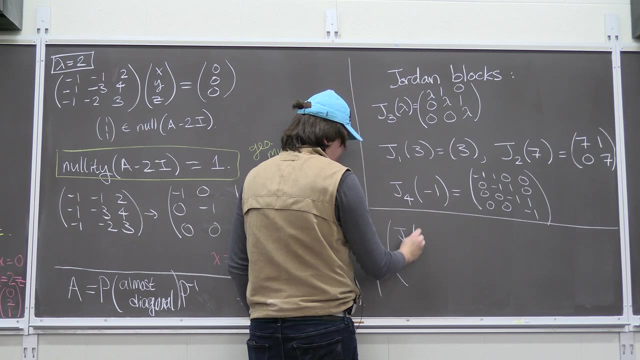 Okay, so these are Jordan blocks. We can also have matrices that are built up out of several Jordan blocks. So, for example, I might have a matrix that has a two by two Jordan block with diagonal value zero, And then another matrix that has I don't know. 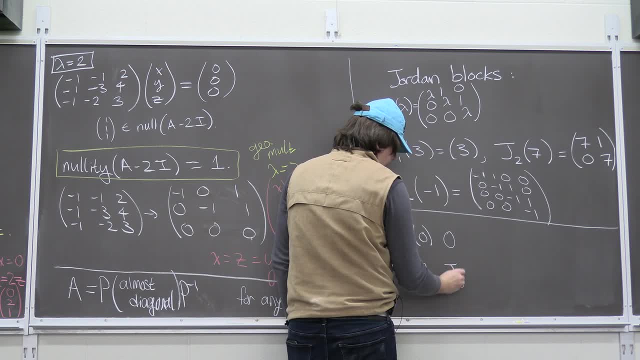 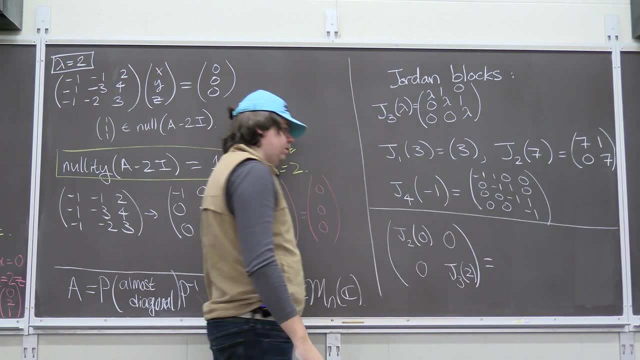 let's say a three by three Jordan block with diagonal value two. So what is that going to look like? Well, overall, it's going to be a five by five Jordan block. It's going to be a five by five matrix. These zeros represent matrices. 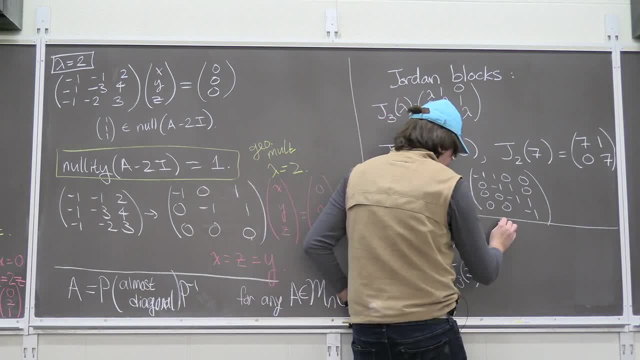 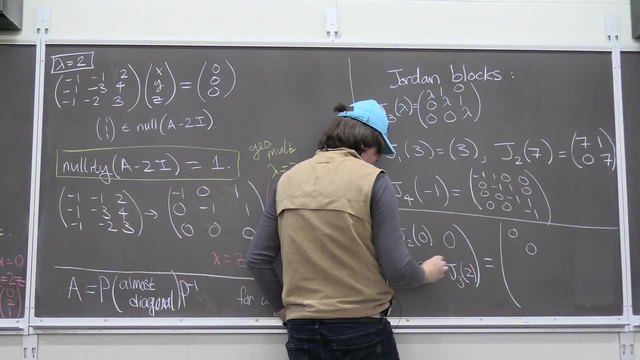 So this is a two by three and three by two matrices, But we're going to end up here with this guy is going to be zeros along the diagonal, a one on top. So here's my first Jordan block corresponding to this guy. 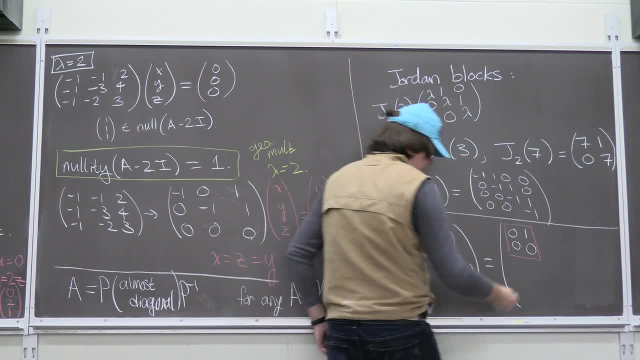 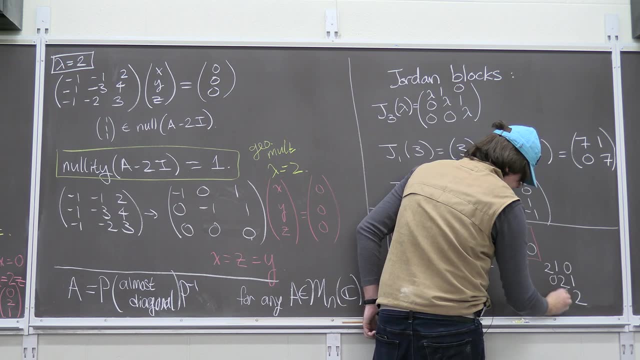 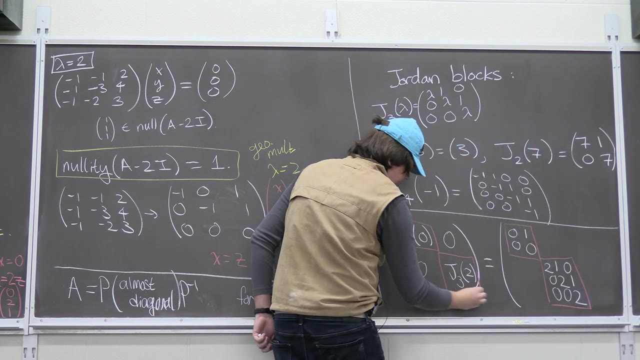 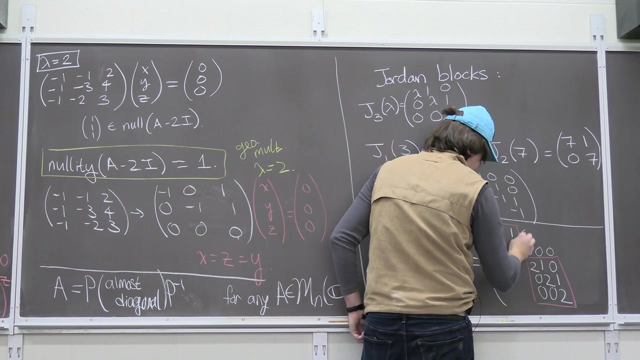 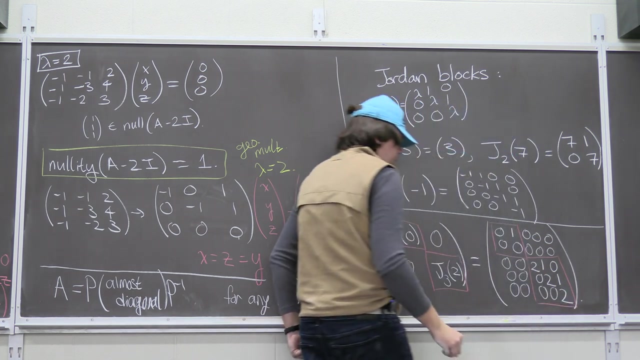 And then I want a Jordan block here, a three by three Jordan block, with twos on the diagonal. So here's my two by two Jordan block, a three by three Jordan block corresponding to this guy, And then zeros everywhere else. Okay, are we happy with the notation so far? 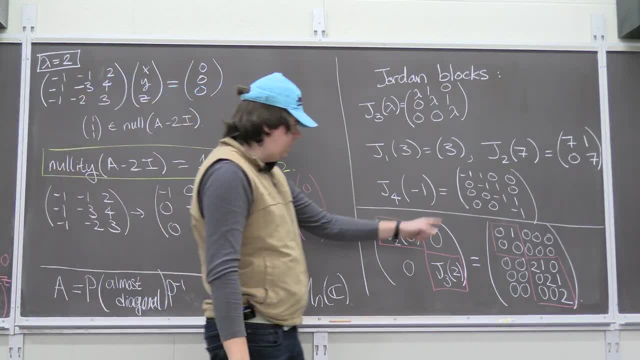 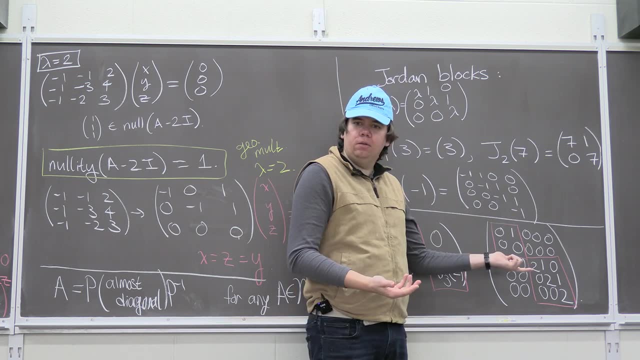 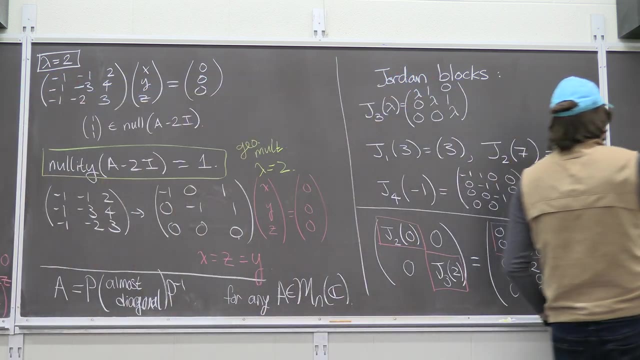 So this matrix is not a diagonal matrix. right, It's got some extra stuff, some extra ones, But it's almost diagonal And it's going to turn out. this is exactly what we need to satisfy our condition. So here's the big theorem. 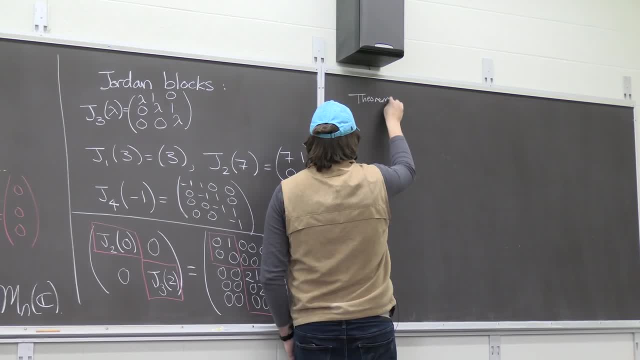 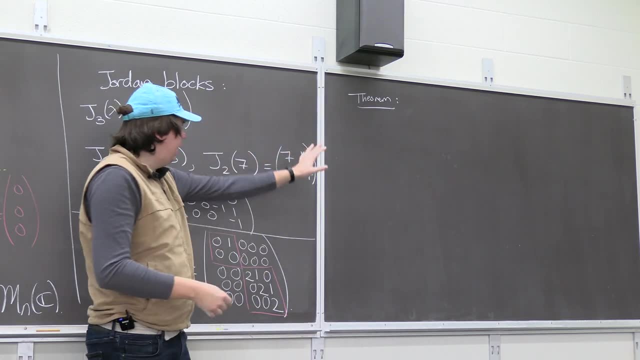 We're not going to prove it today. We'll make a little bit of progress towards it. We'll focus on the proof, next class and then some applications on Friday. Today I'm trying to introduce it and we'll talk a little bit about how to work with it. 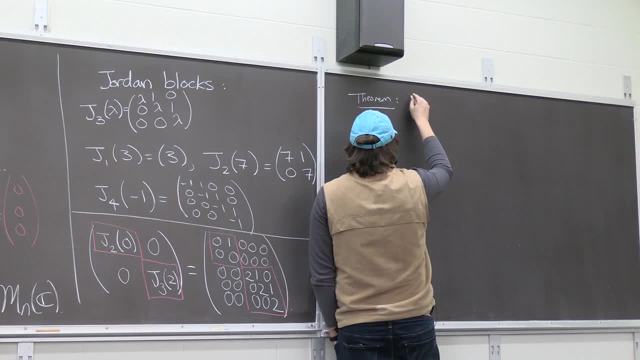 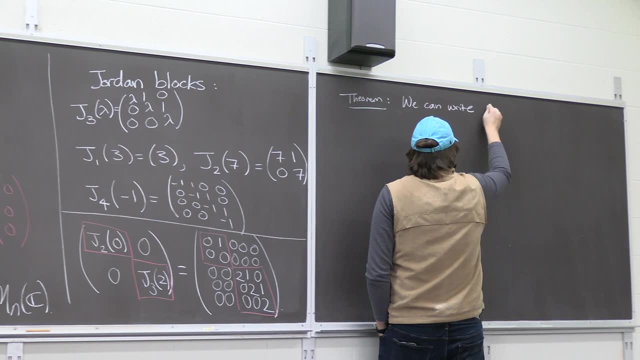 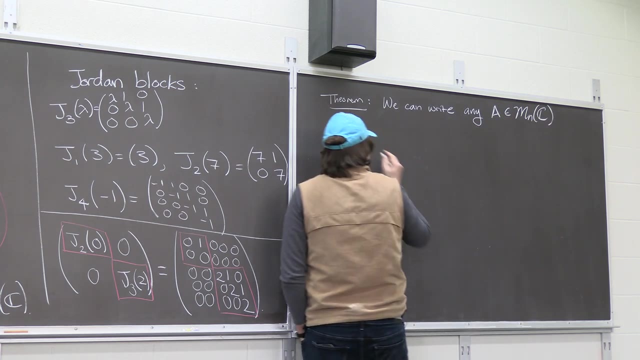 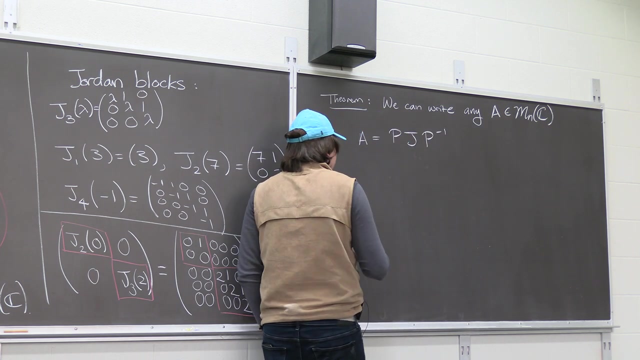 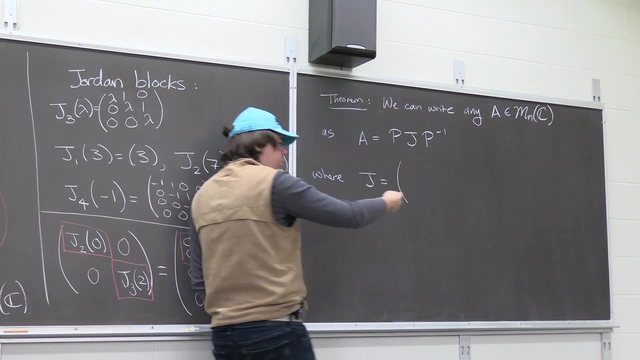 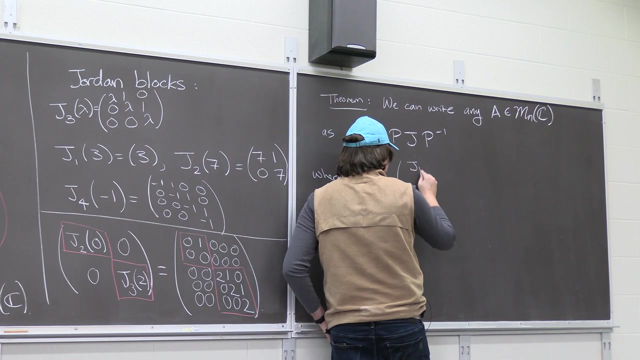 So here's our theorem. We can write any matrix, any square matrix, as A equals P, J, P inverse. where J is your square matrix, It should sum almost diagonal matrix made up of these Jordan blocks, like this guy, So I don't know how big these Jordan blocks are. 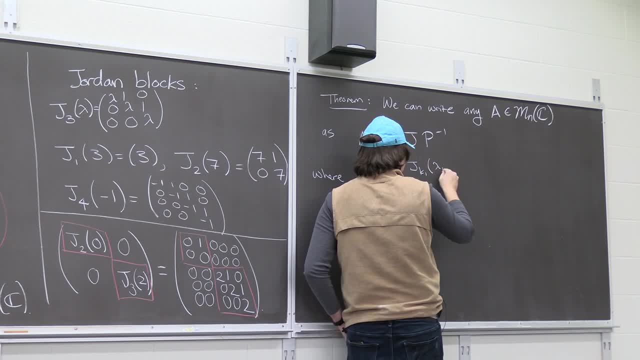 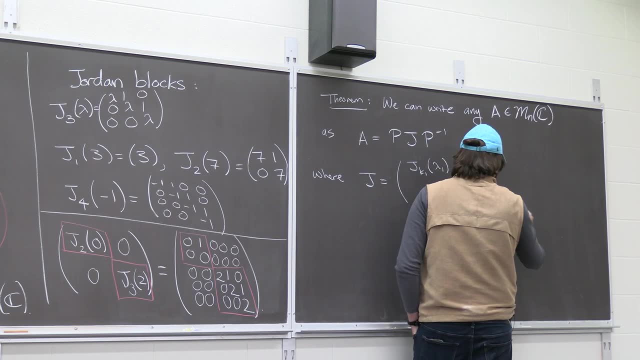 I'll say K one, so it's a K one by K one matrix with some value lambda one. I'll call this K two with some value lambda two Down through it. whatever the last one is, It's like K M with some value lambda M. 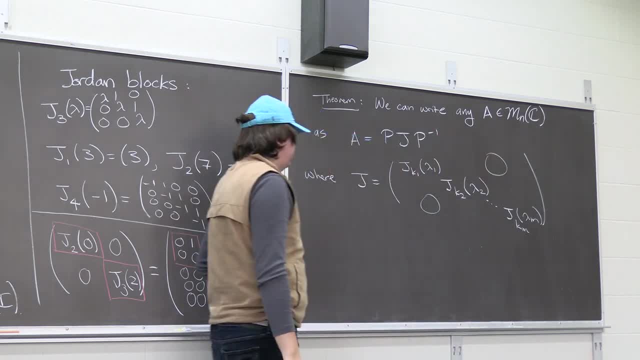 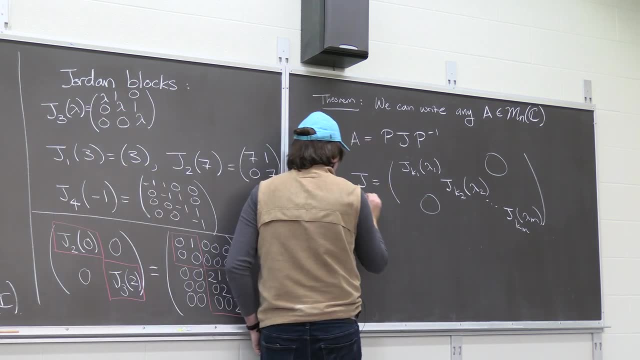 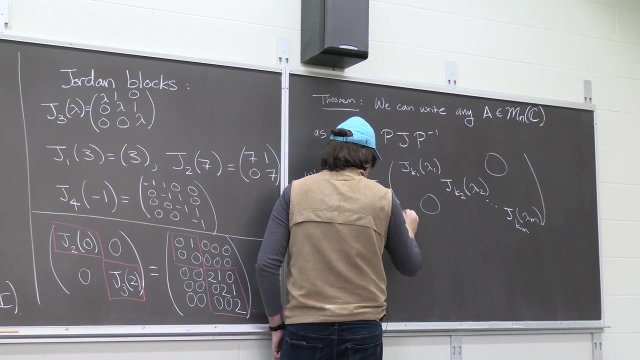 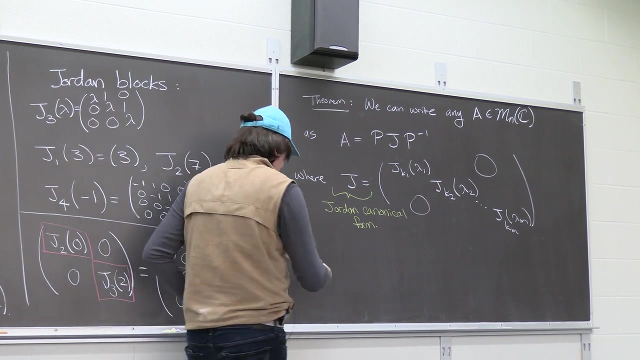 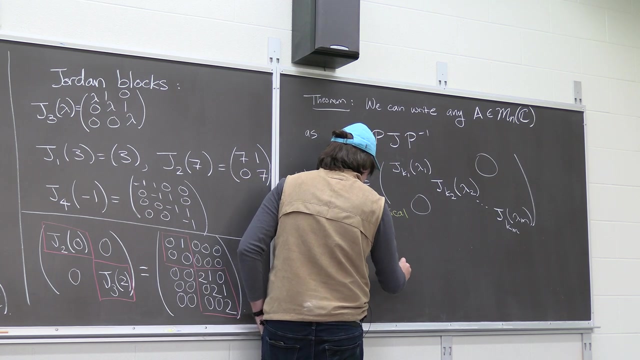 And zeros everywhere else. All right, zeros everywhere else. This matrix, this J, is called the Jordan canonical form, And my goal, by the end of today's class, is to try and convince you that J is unique. It's an unique matrix. 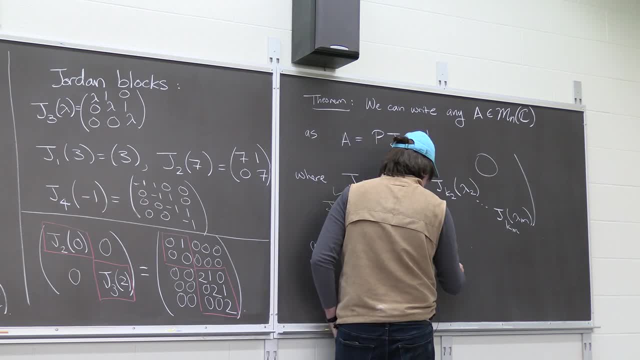 It's unique because A is unique, An unique matrix. So J is unique because A is unique And A is unique because A is unique. So the problem is this: matrix T is just aienie matrix up to dH, to the vector. 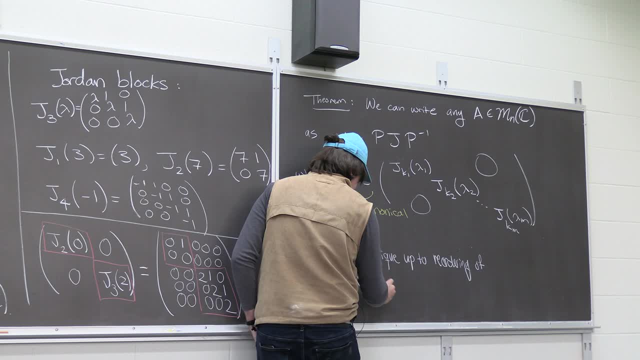 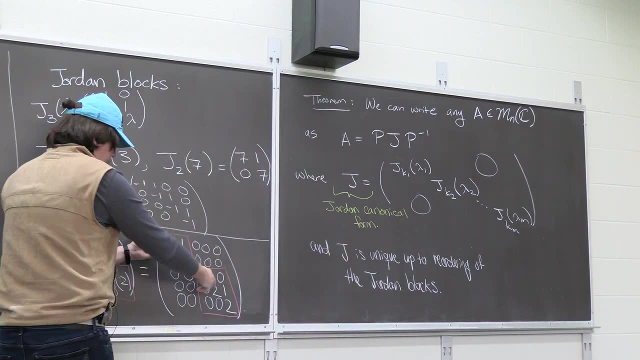 So this, nothing but the original matrix by the last two. So now these pieces of this matrix are worth P to the vector in the first case, because B is the matrix of the vector, And if we subtract the value of the vector then we can figure out that this is the matrix. 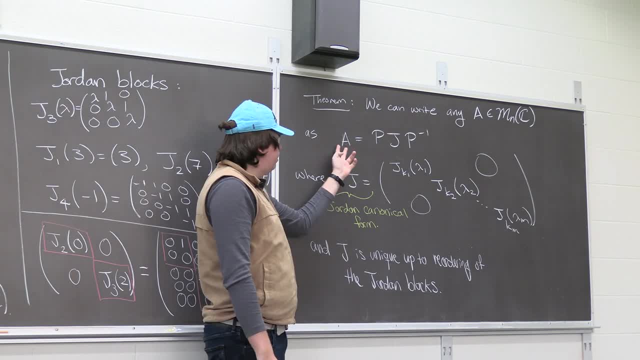 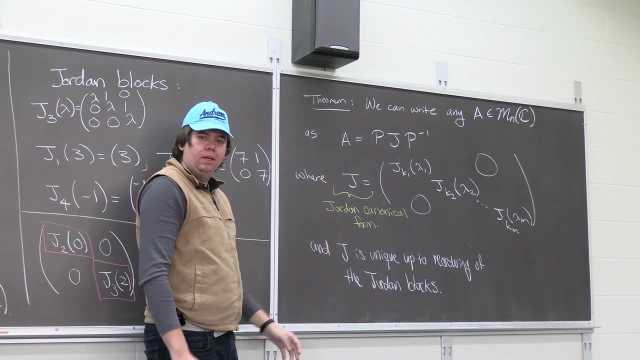 of the vector you're looking at. So these are two parts to this part of this theory For a. there's two different parts of this theory: change of basis in this Jordan canonical form, And the second is the uniqueness right. So I'll build up to talking a little bit about uniqueness by the end of 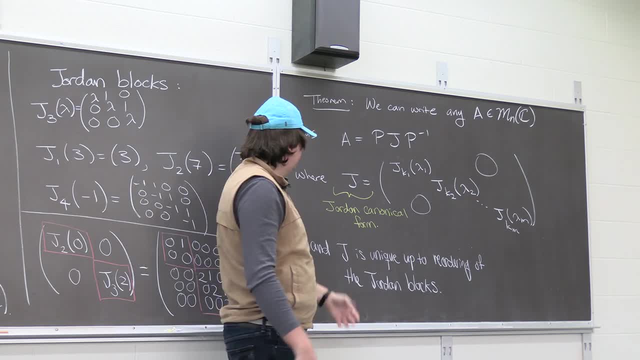 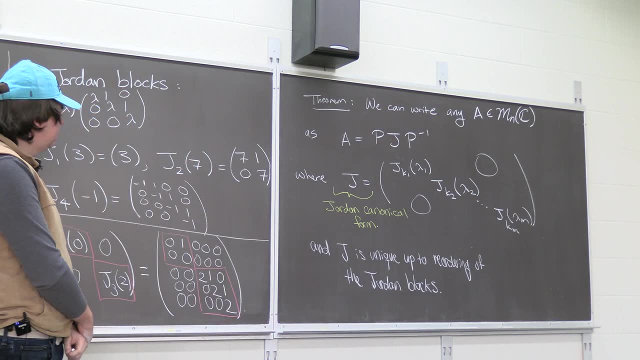 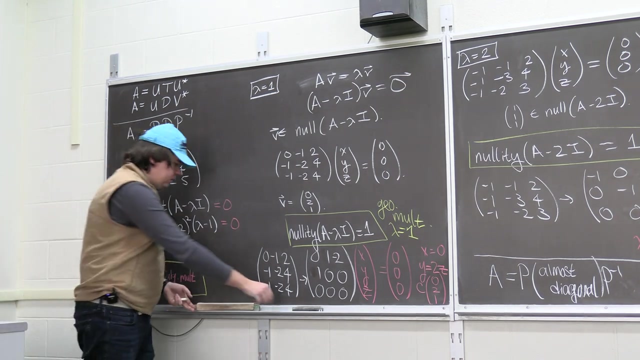 today's class, but then we need to come back um in our next class and talk more about the existence, why you can always do this, right, Okay, Okay, I'll come back to this example in a few minutes, So let's just remind ourselves where we already found. 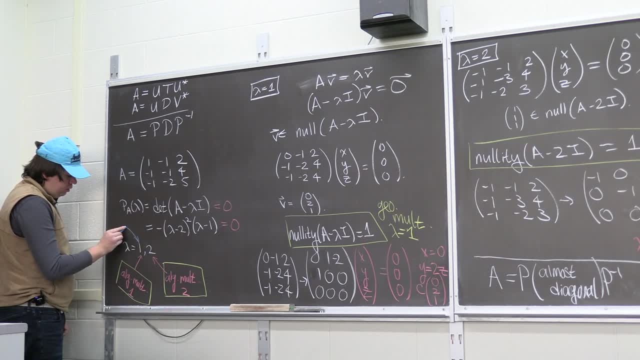 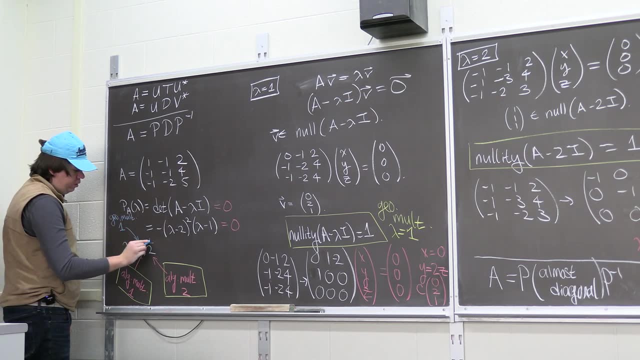 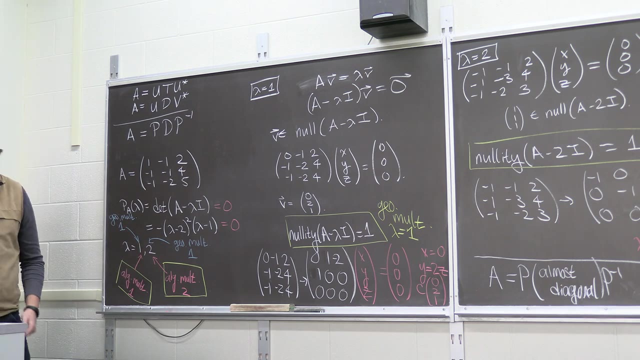 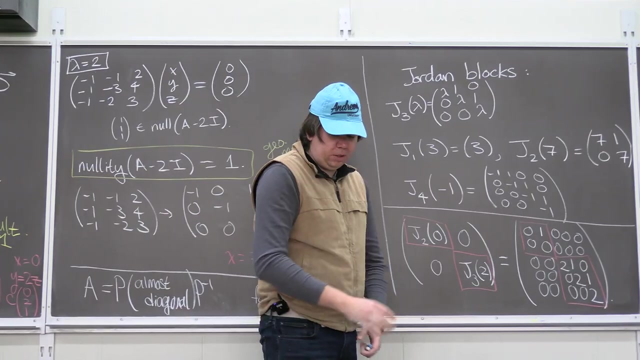 although this guy had algebraic multiplicity one and two, reset here that his geometric multiplicity was one for both of them. So those both have geometric multiplicity one. Okay, So so maybe I should just like pause for a second Um. 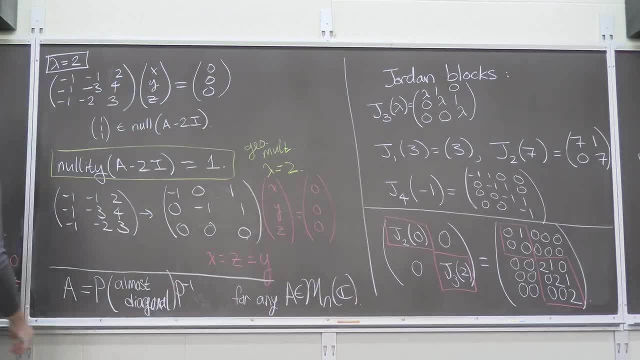 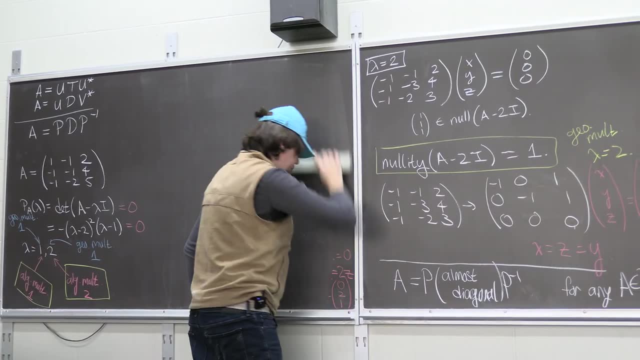 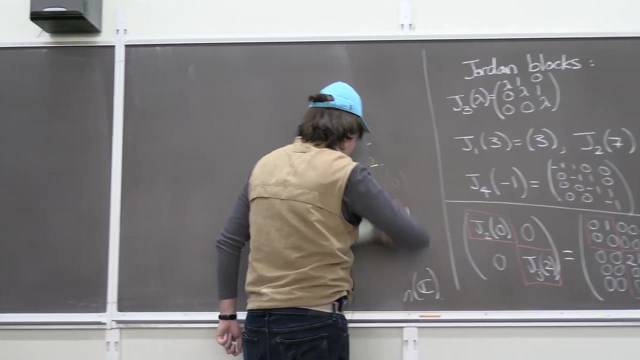 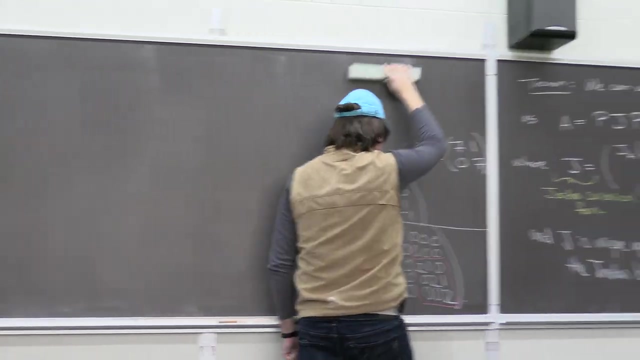 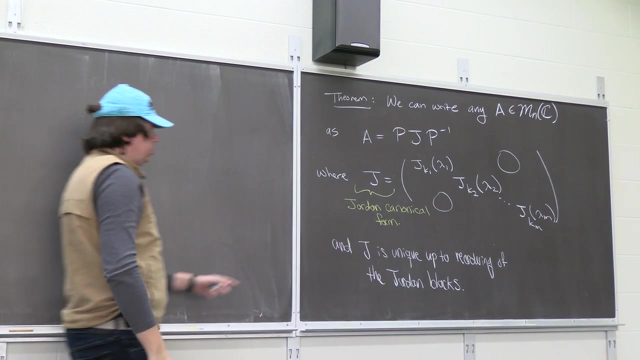 are there any questions about what's theorem is saying Yeah? if not, yeah, A P is a change of basis. It's not necessarily unitary, So it's just any invertible matrix, right It? um, we're not guaranteed. It's a nice unitary matrix. 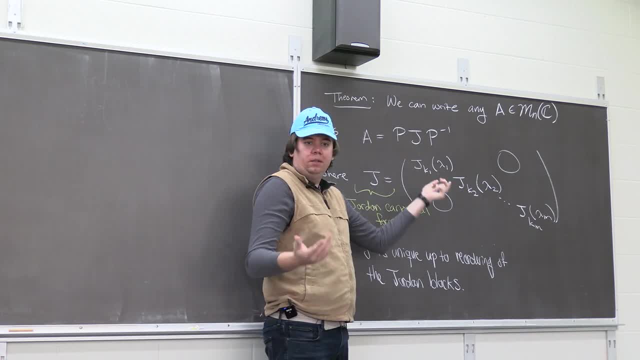 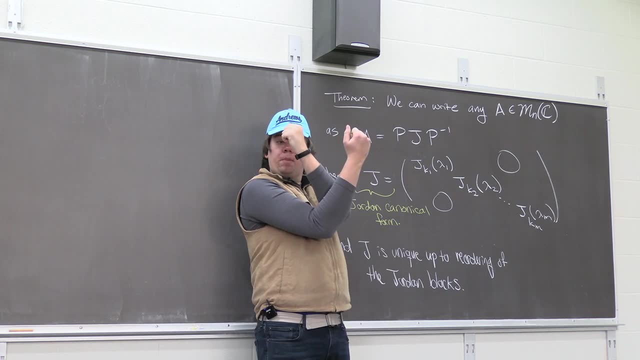 It's just some square matrix that's invertible, nonzero, determinant, so that it has an inverse right. So you just change in basis from your standard basis to some other basis and it may no longer be an orthogonal basis. It may no longer be orthonormal right. You could have whatever the other basis. 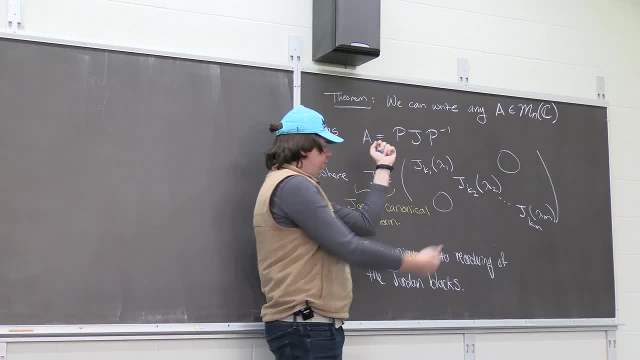 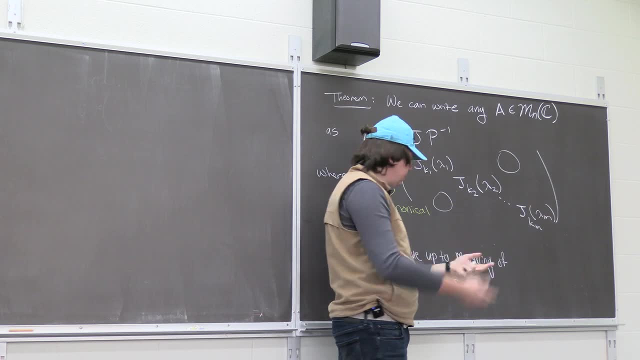 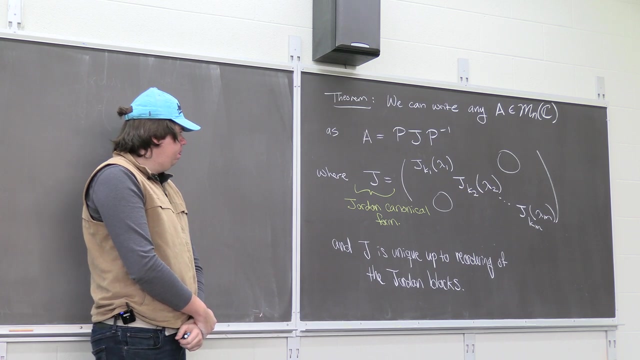 be, you know, maybe something like that. right, P is just finding some basis so that the linear operation represented by a is under this new rep, uh, under this new basis not represented by this matrix. Well, yeah, So reordering the value? 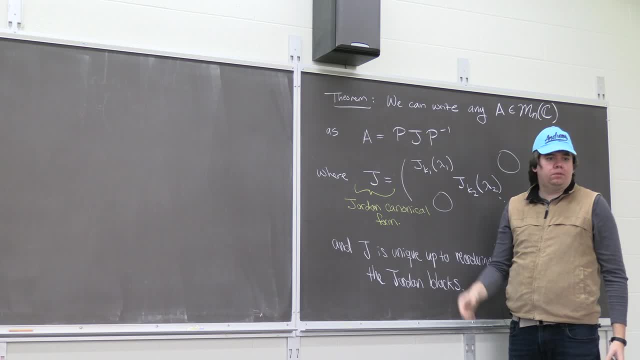 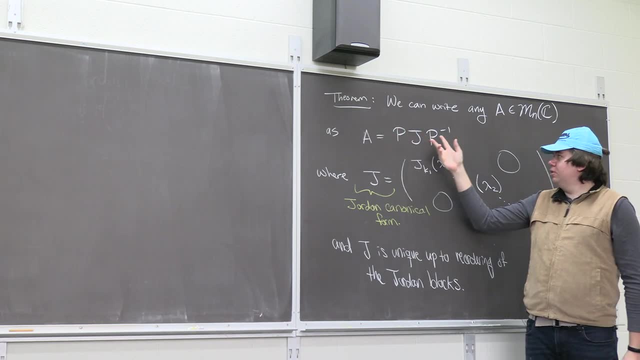 reordering these blocks would be like reordering the columns of P, Right, Um. and then of course, you can do things like: if you scale one P, uh, if you scale it by two, you're scaling the inverse by one over two. 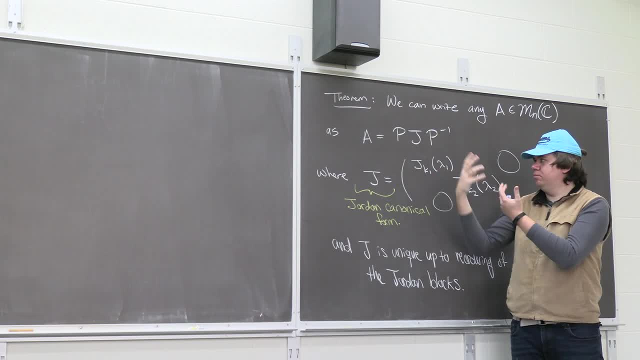 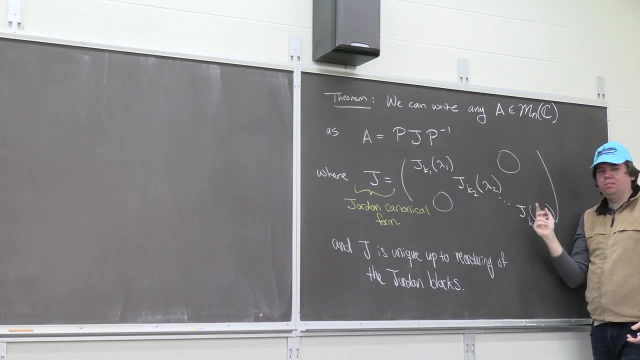 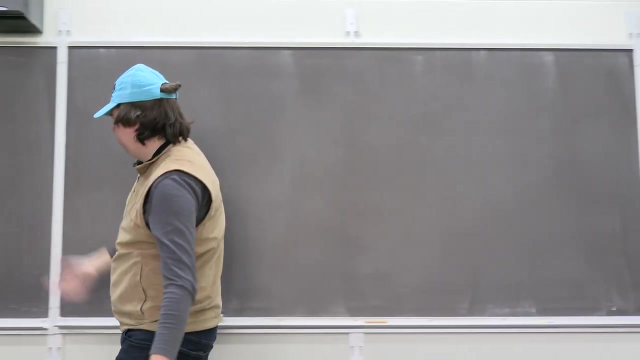 And so that wouldn't change anything. So you'll, you'll be able to um. P has a little bit of some some freedom where you could scale it or you can reorder the columns of P to reorder these blocks. But I guess what I really want to do is actually find 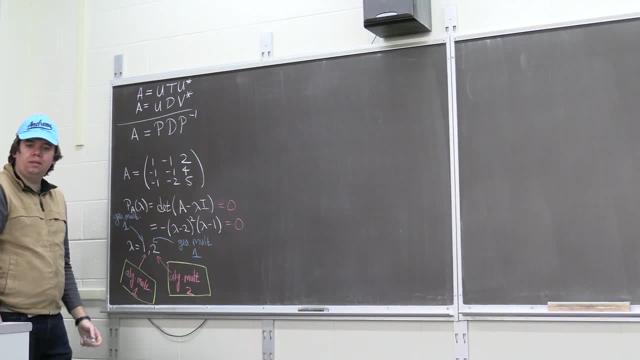 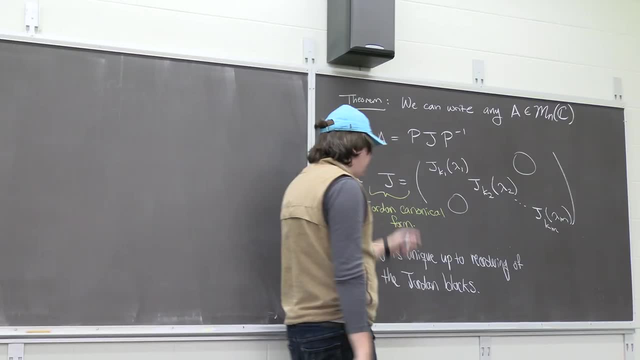 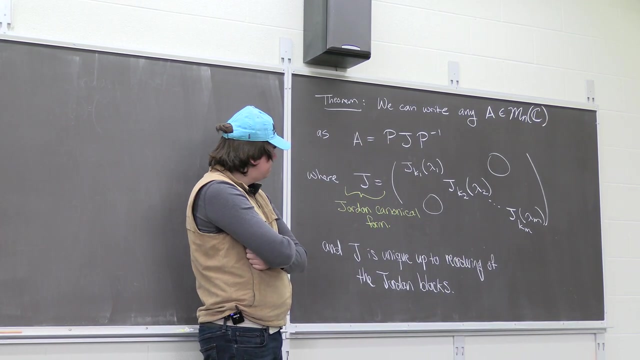 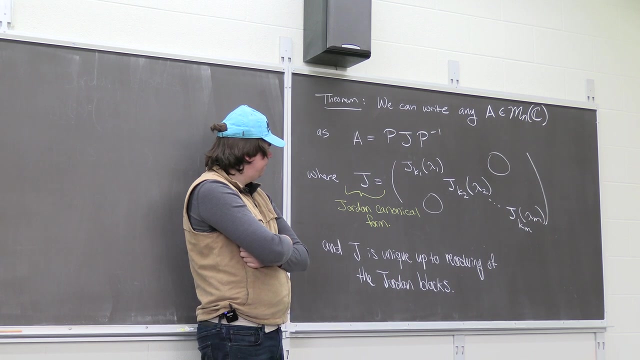 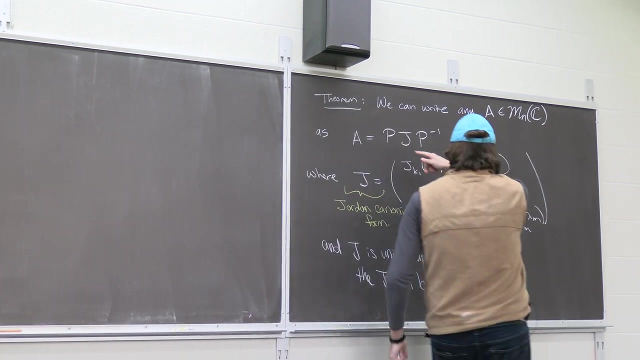 um what the Jordan canonical form corresponding to a is, And so my first observation is going to be: well, what are the eigenvalues of J? Why Good, Since it's an upper triangular matrix. it's not quite diagonal, It's extra ones on top, but we've said before upper triangular matrices. 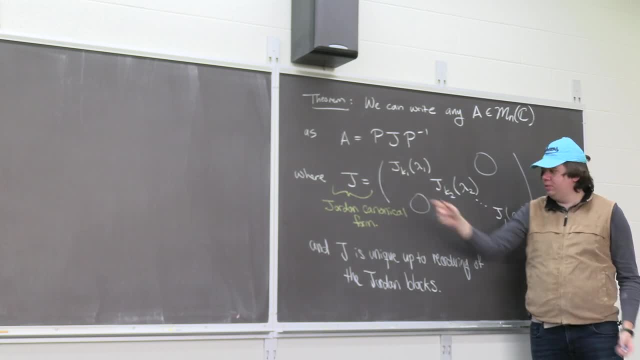 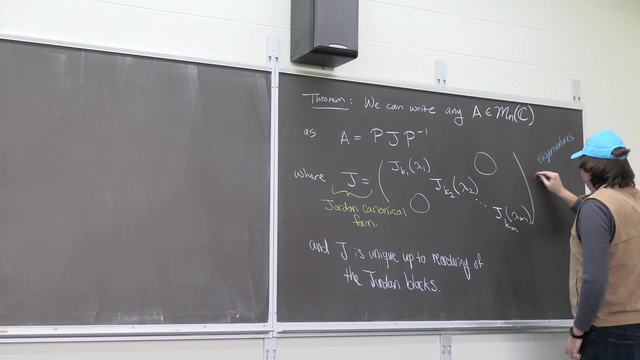 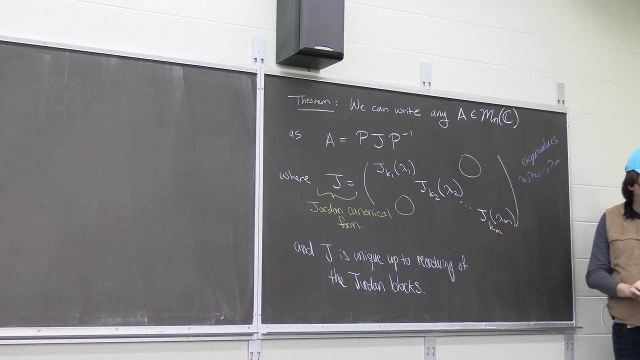 the eigenvalues are just the diagonal entries. So my eigenvalues of J- So this is J- has eigenvalues: Lambda one, Lambda two through Lambda M. I mean, it was kind of suggestive when I started using Lambdas that we're talking about eigenvalues, but but since it's upper triangular, 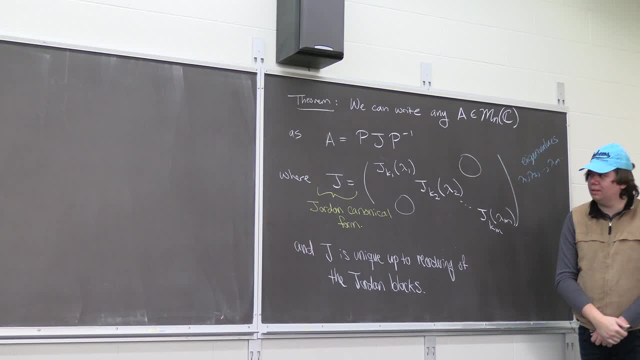 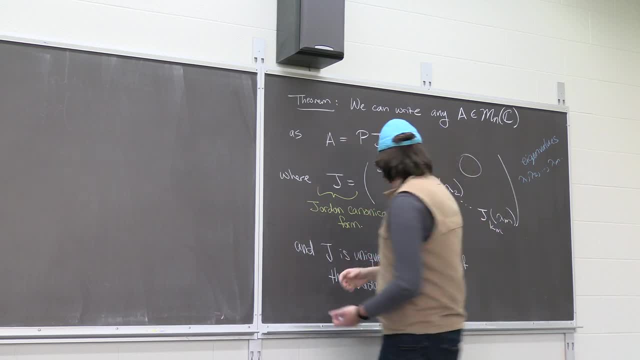 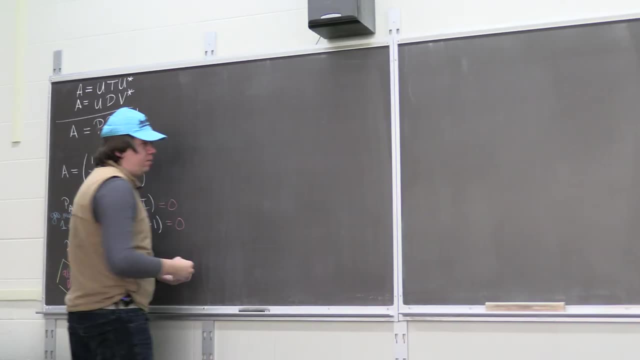 What happens when you change base. Well, I mean, let's, let's just prove this really fast. I mean maybe you forgot this, but change of basis preserves eigenvalues, So let's do it over here. So like I want to argue that a and J of the same eigenvalue right? 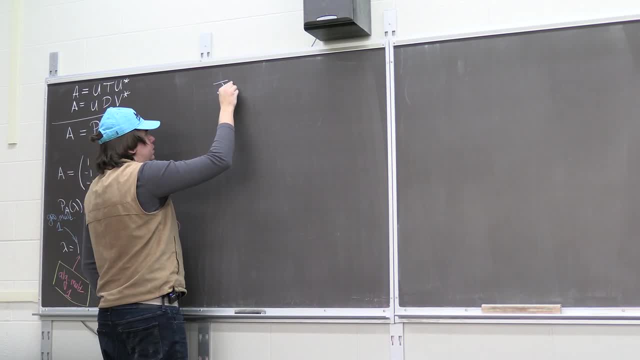 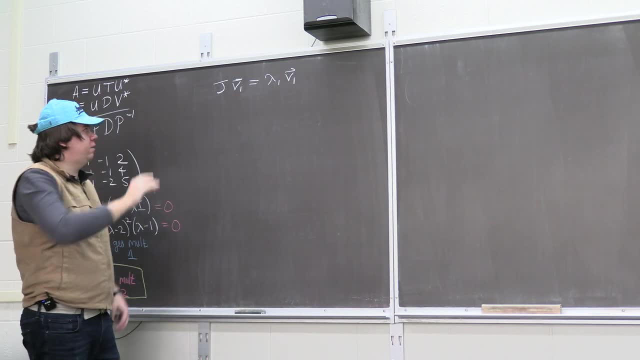 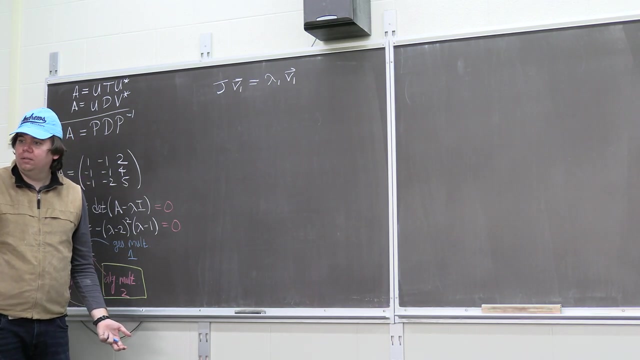 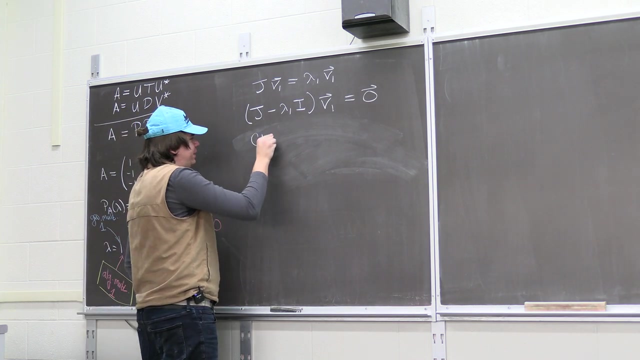 So I know that, like J times, some V one is Lambda one times V one, Lambda one is some eigenvalue of J. I claim that it's also an eigenvalue of A. How can I see that Change of basis? so change of basis. 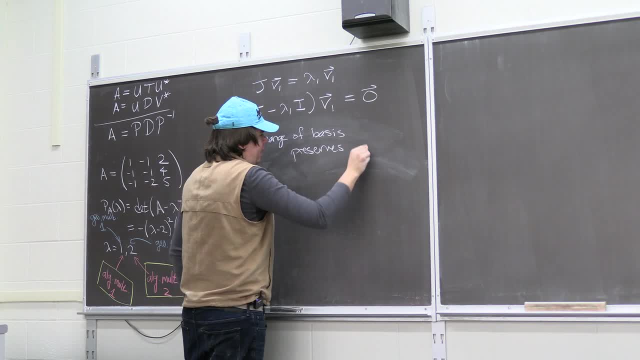 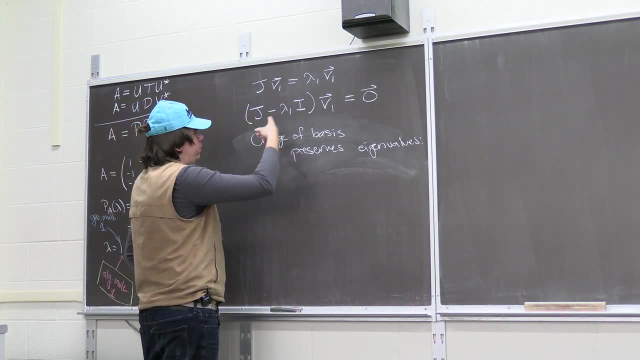 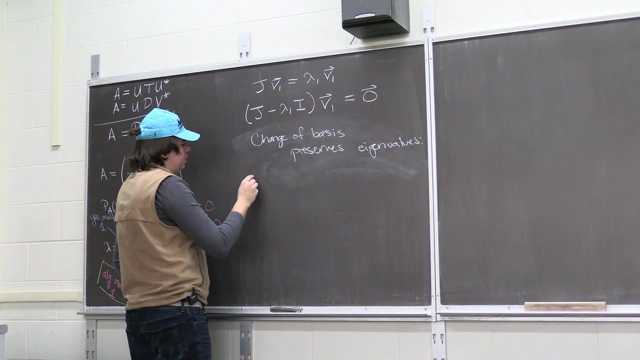 preserves eigenvalues. So why is that? Well, here's why I mean, we didn't have to write it like this, We could have just done the original guy. So the claim is that: well, let's just see it here. 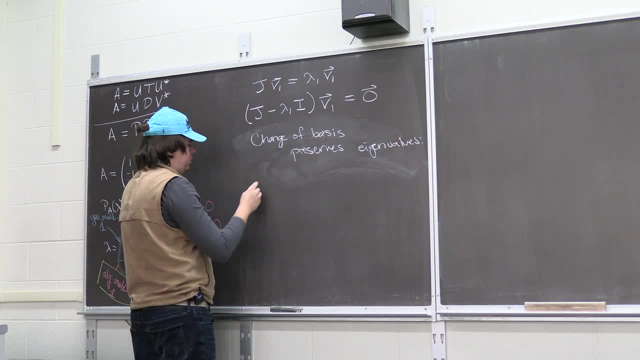 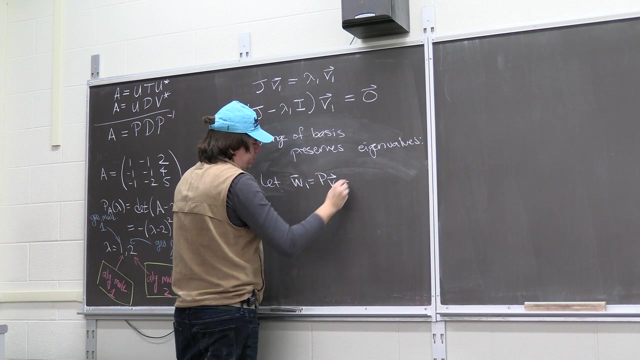 that if you, instead, if you change your basis. so, if you want to change your basis, this is now A, But instead of looking at V1, I'm going to look at P. So let's just write like this: Let W1 be P. 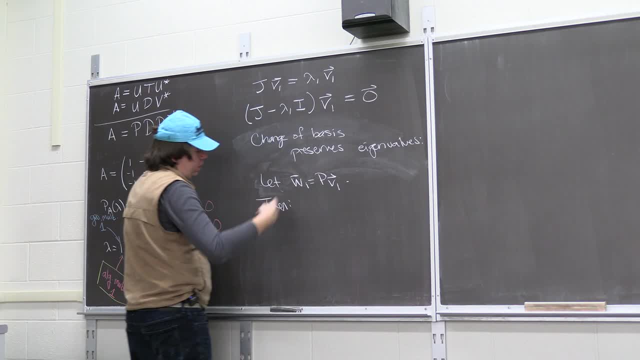 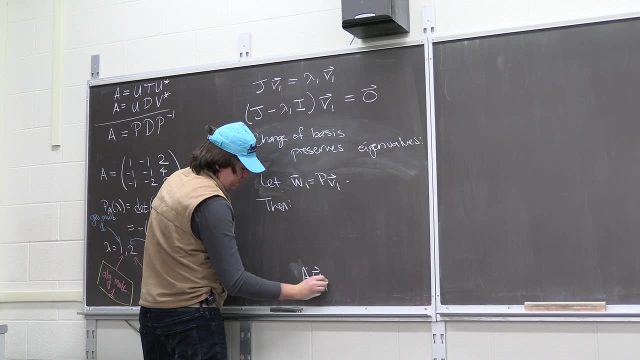 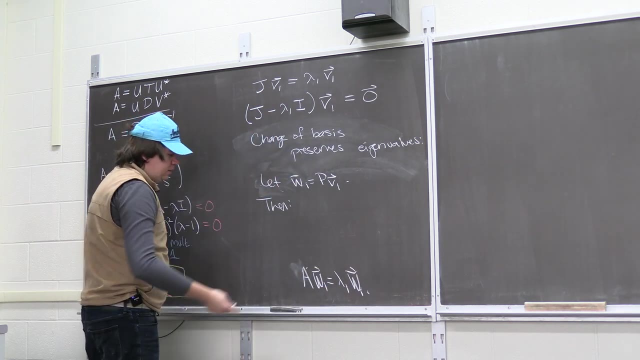 Then I claim that. well, let's see, I mean, my claim is that A, which is your change of basis, W1 is lambda 1 W1.. Okay, I didn't plan to do this, but this is what I want to show you. Why is that true? 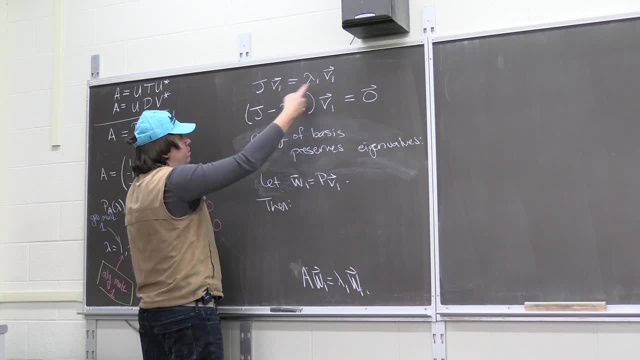 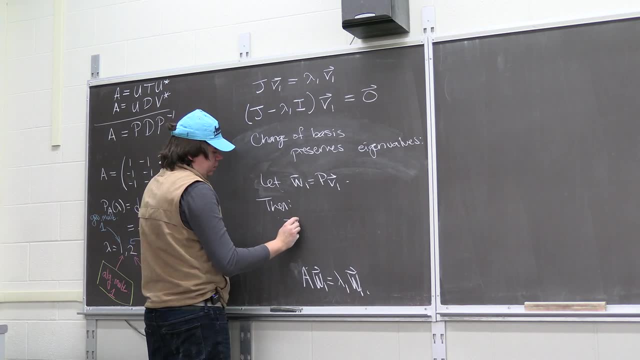 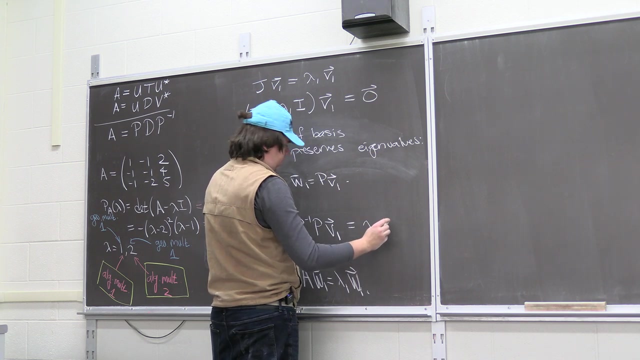 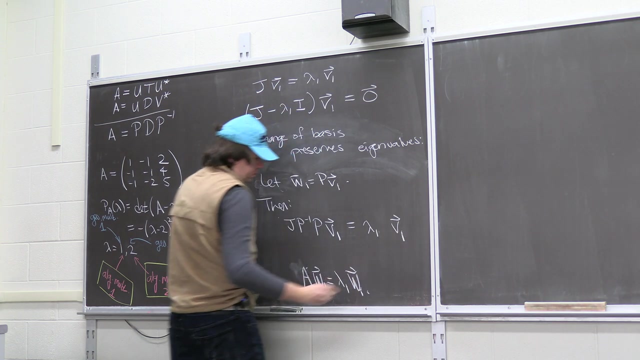 Well, the reason this is true is because from this relation we get that J V1 is the same thing as J P inverse P V1. Because these just cancel, Which is the same thing as lambda i times V1.. Now I'm going to multiply the left-hand side by a copy of P. 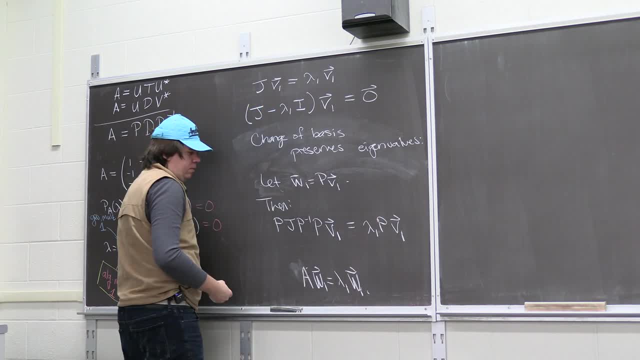 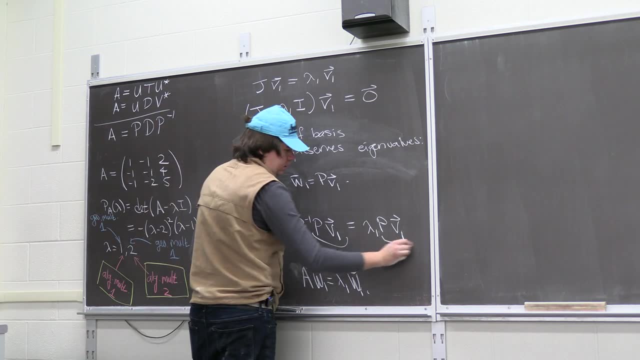 So I'm multiplying this by a copy of P, I can pull out lambda 1.. And now, what do you have? Well, this is exactly A. This is exactly W1.. Is lambda 1 times p. lambda one times W? one. 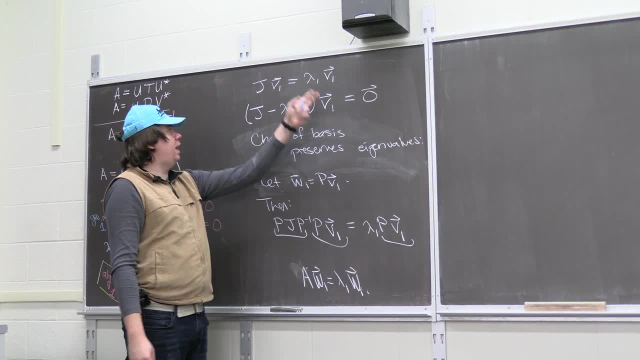 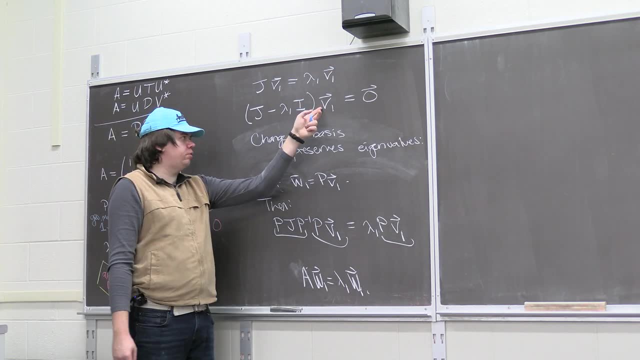 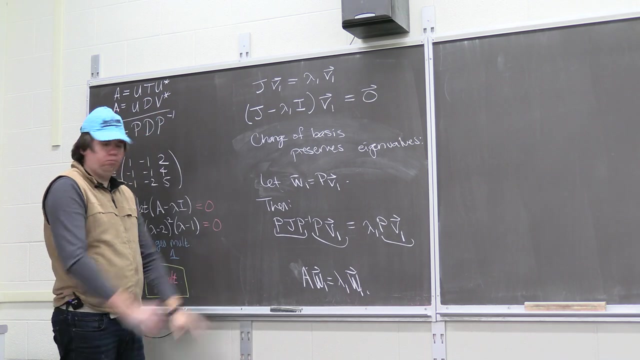 So if lambda one is an eigenvalue for J, then lambda one is also an eigenvalue for A, where the corresponding eigenvector changes from V one to P times V one. Your change of basis just changes the eigenvector. Is that good? 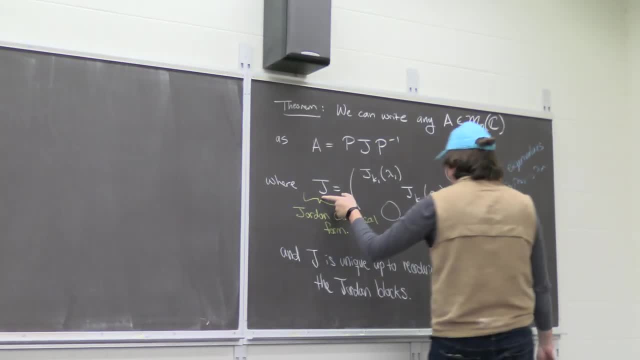 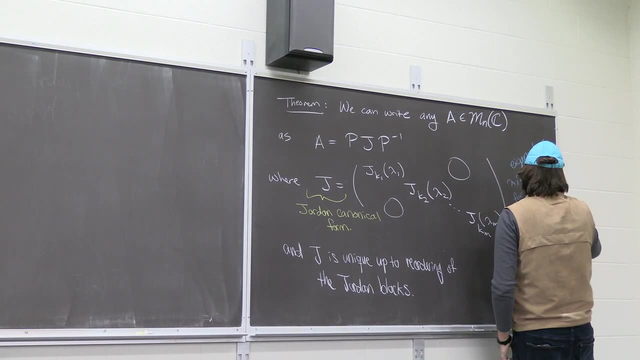 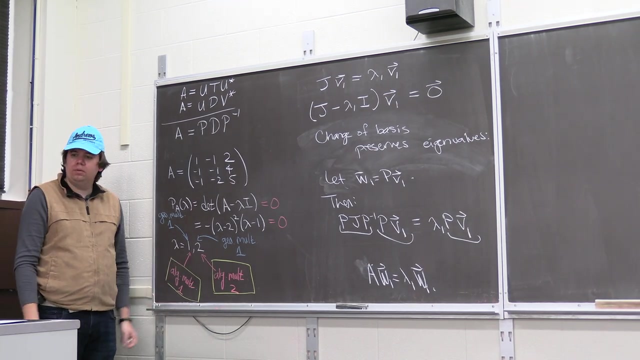 So we're saying that A and J have the same eigenvalues. Lambda one through lambda M are eigenvalues for both A and J. So it's like: okay, so what can J look like? Well, I know J has to have eigenvalues one and two. 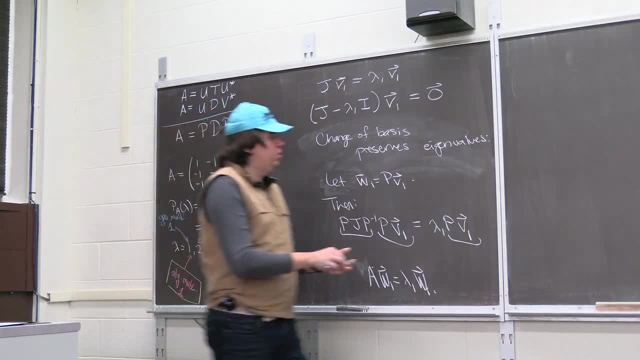 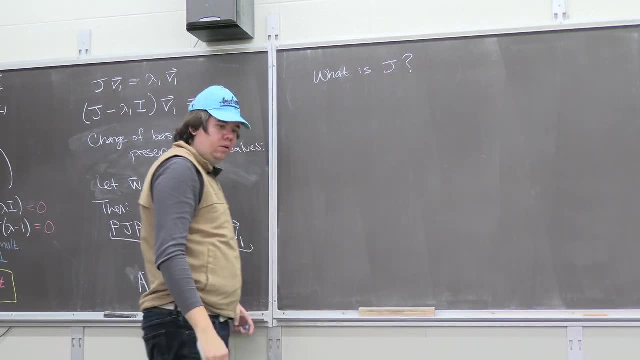 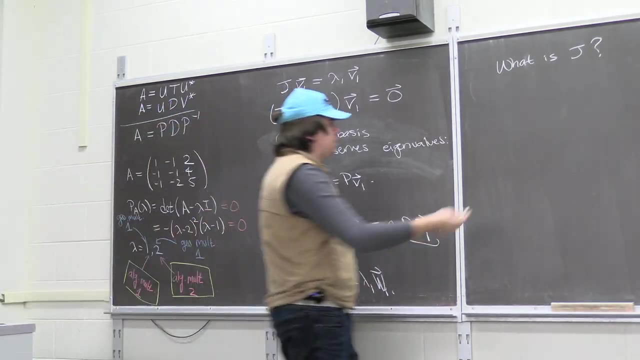 So what is the J corresponding to my A here? So, given this A, what is J? Well, it has to have values one and two. So you might look at this and you'd be like, well, maybe, maybe it has like a one by one block. 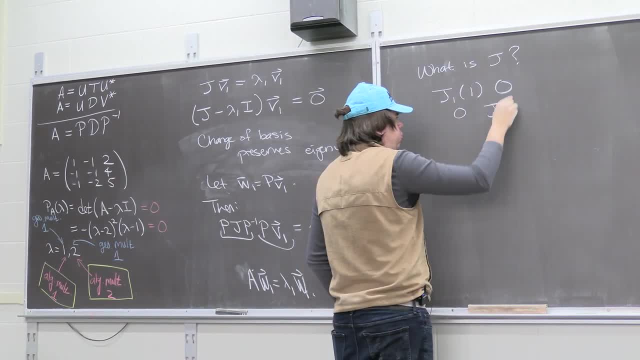 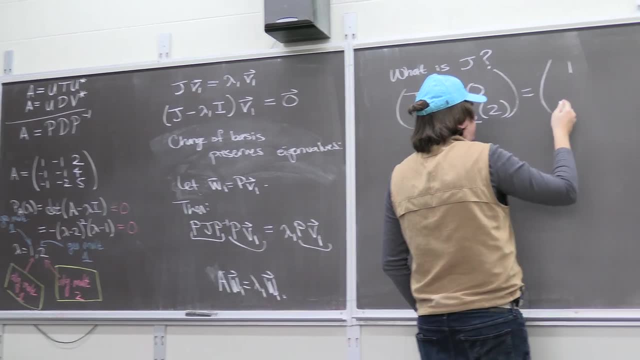 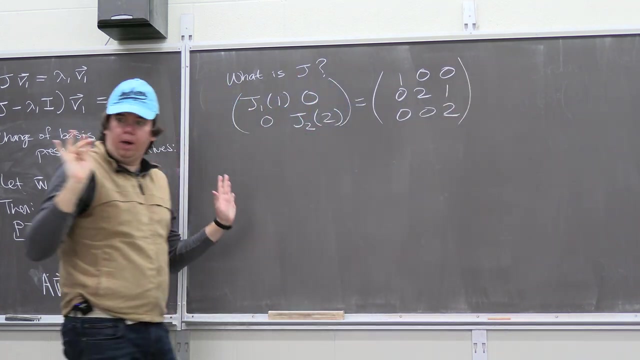 for your one and a two by two block for your two. So maybe my J looks something like this: Maybe it looks like a one by one block for my one and a two by two block for my two. So maybe my J looks something like this possibly. 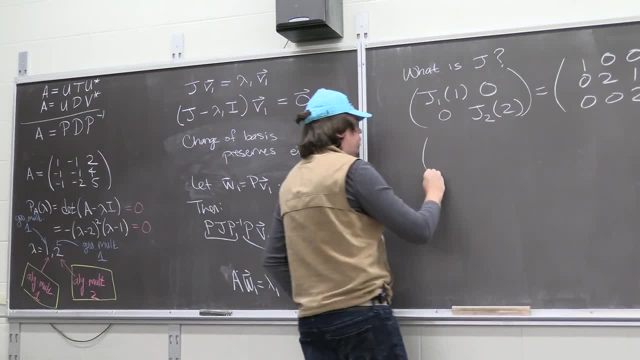 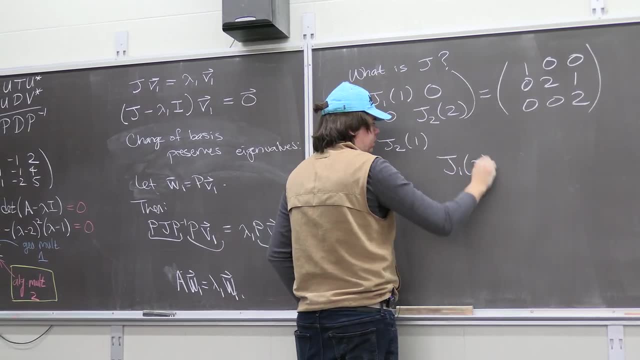 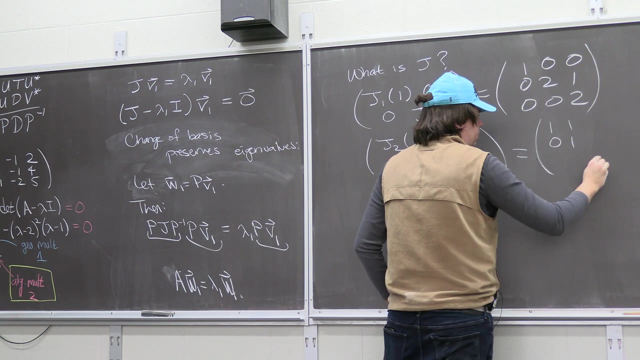 Or you're like: well, maybe, maybe the one has a two by two block and the two has a one by one block, Like that could be how it looks. So it could look like one, one, one and then a single two. 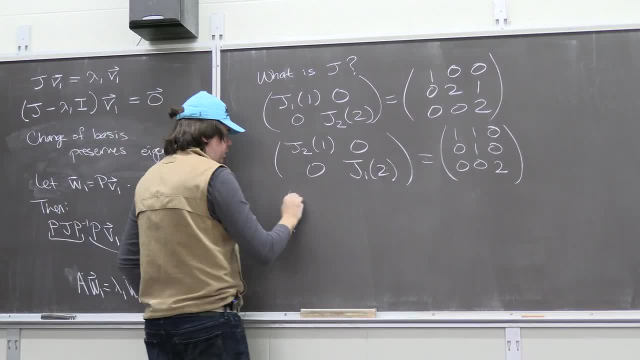 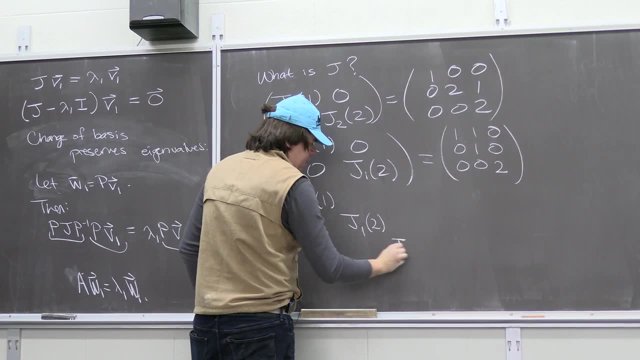 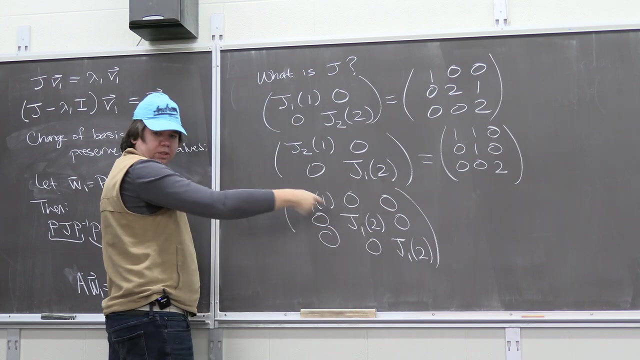 Or maybe it's like: your one has a one by one block, Your two has a one by one block, And then your two has another one by one block. This would be also something which is eigenvalues- one and two. This would be well. then it actually comes out. 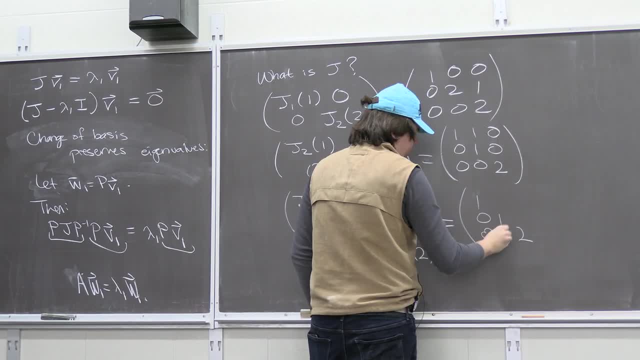 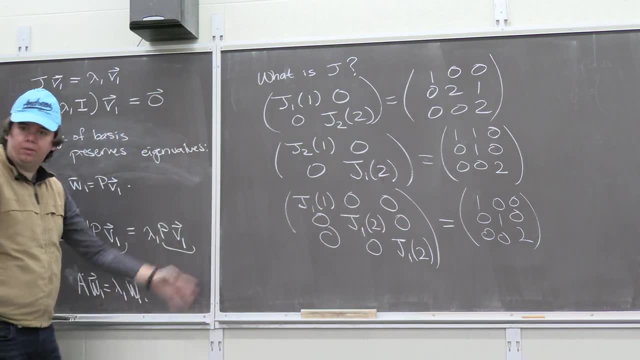 to be just diagonal One, one, two. I guess we rule this one out because we know it's not diagonal right, But in principle there's a lot of options, is what I'm trying to show you. right, Like I know, it's one of these guys. 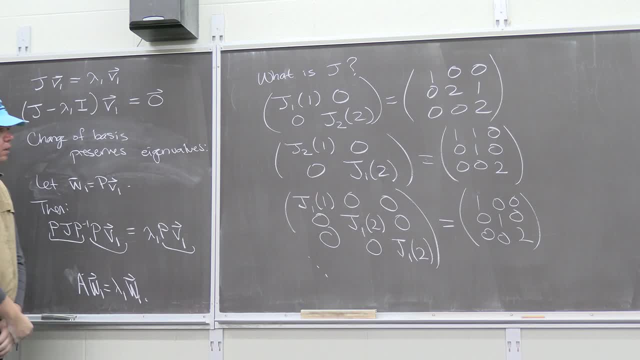 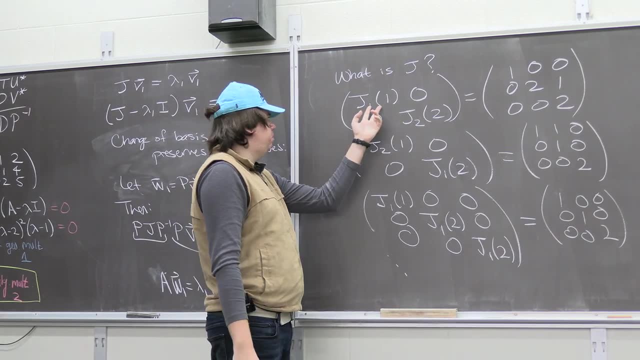 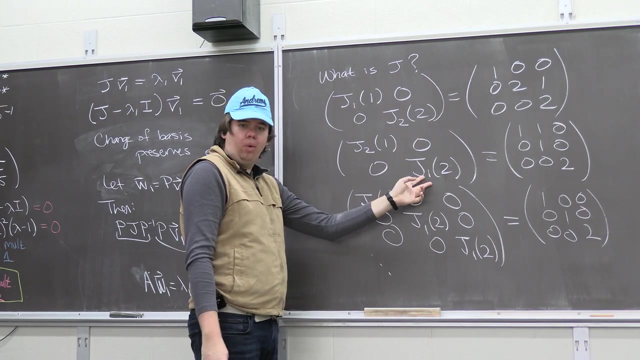 But I don't know which one it is. So what I need is I need some way to count how many like J one blocks are there of size one and how many of size two, or like how many of the J twos are there of size two or of one right. 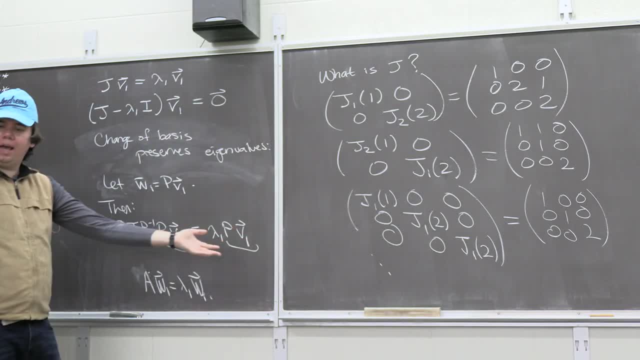 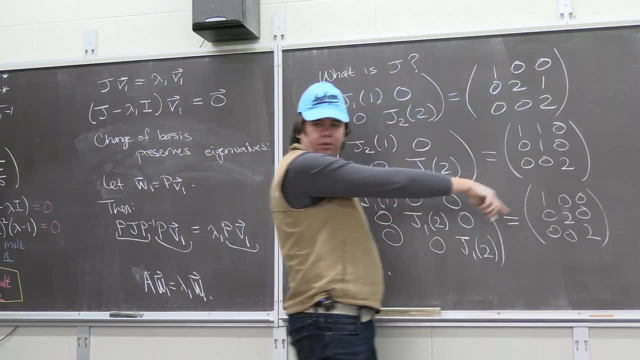 Like that's what I need to know is, like, what combination of these should I have? Yep, Yeah, great, This one is two twos. you're right, I could have also had one, one, two, but the way I wrote it was wrong. 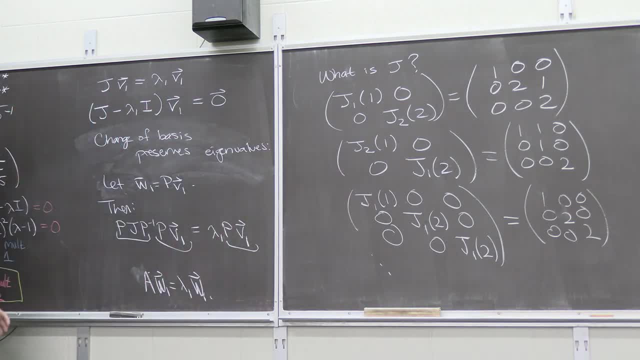 It was one, two, two. We know that's not gonna work. the last one because we said this is not diagonalizable, but you can imagine, you know, especially if you have like a 10 by 10 matrix, it's like there's a lot of different ways. 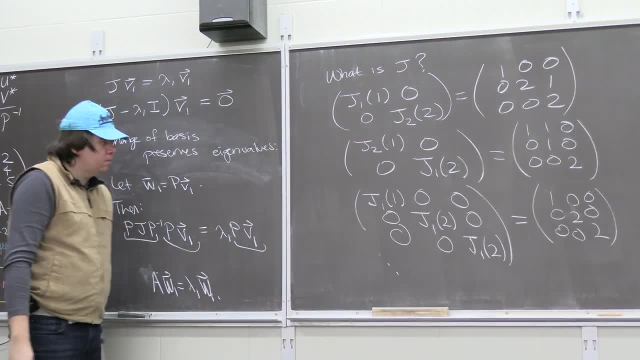 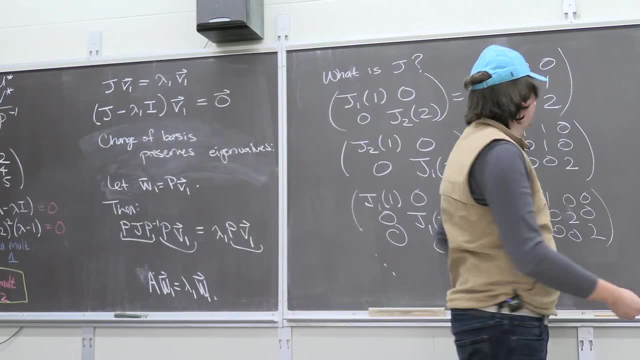 you could put these blocks together with a couple of eigenvalues, right? So it's like which one is it? So we need some result, And so I'm going to give you a theorem and maybe say it just briefly, outlined the sketch of the proof. 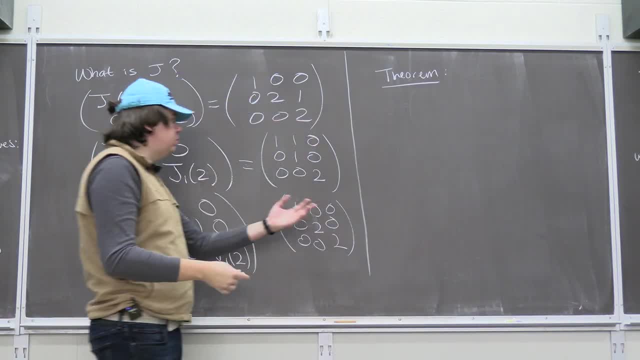 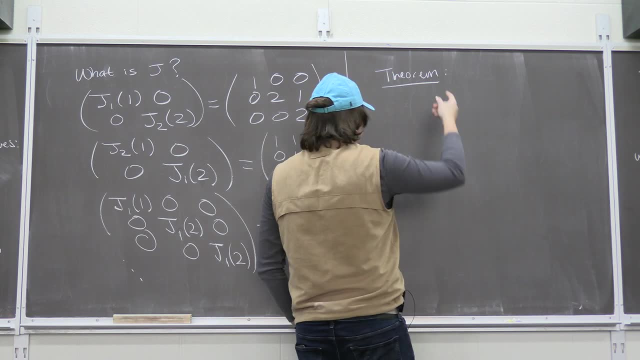 And once I do, I'm then really going to say, I'm then really gonna be focused on using that theorem to give us some information in this case, and recovering some facts for us. So here's the theorem, Here's the answer of how many of each size block there are. 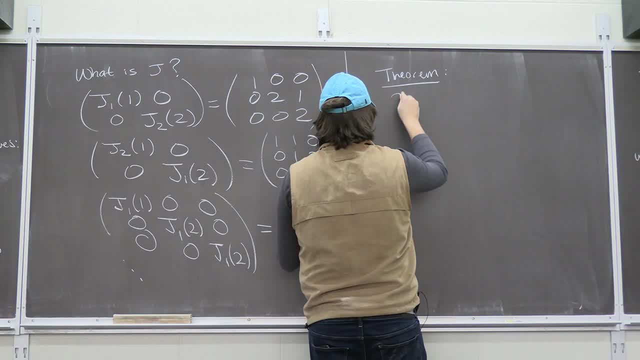 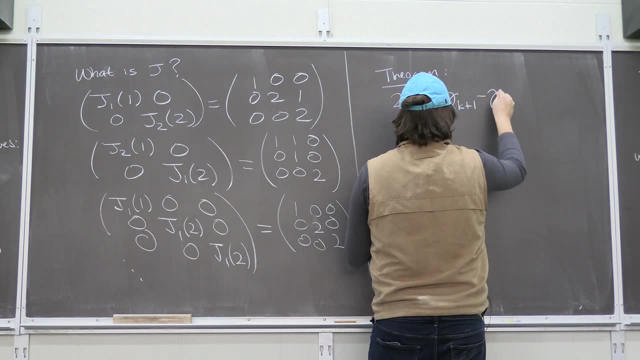 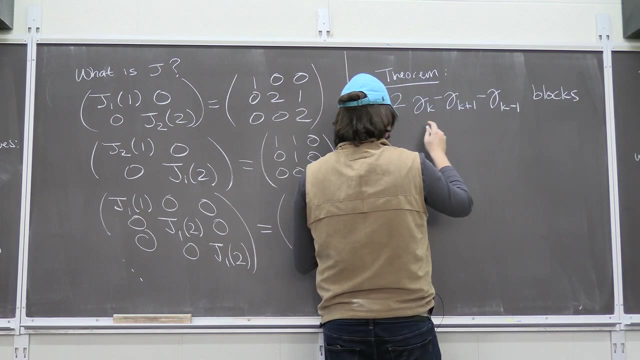 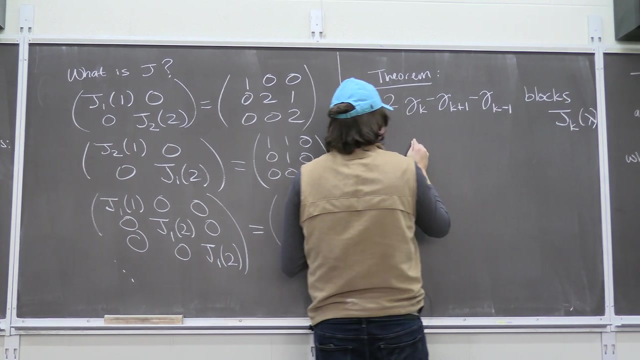 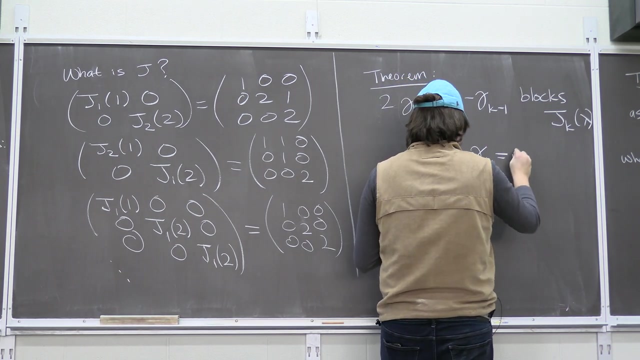 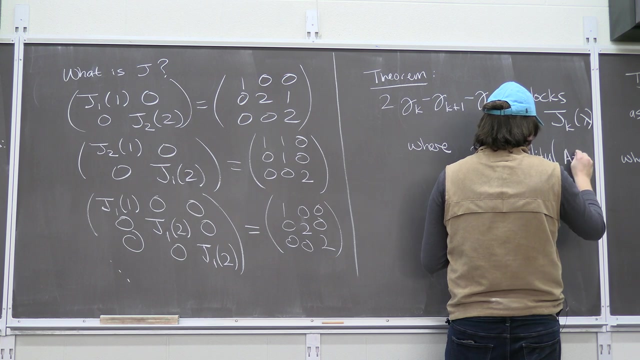 The answer is there are two gamma K minus gamma K plus one minus gamma K minus one. blocks of the form JK, lambda, where each lambda K is just equal to the nullity, the dimension of your null space of A minus I. lambda to the K. 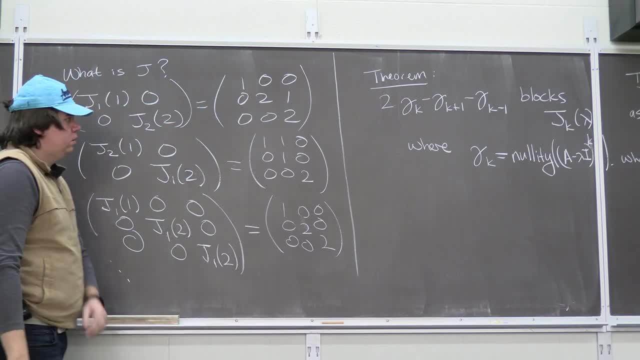 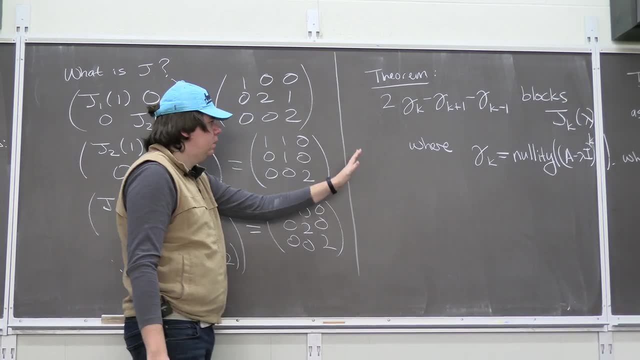 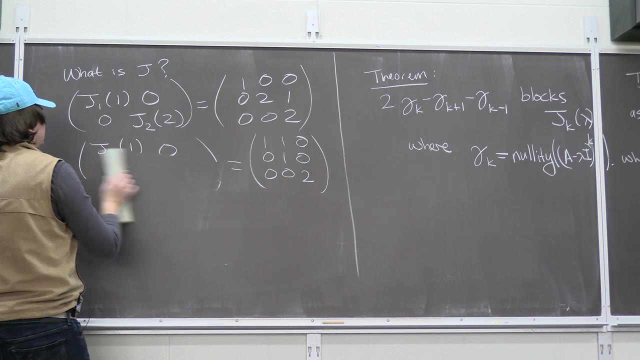 So hang on. Okay, Maybe we should use this theorem and then I'll say a few words how to prove it. But let me just make sure we're clear on what it's saying. We're still trying to figure out what J is. 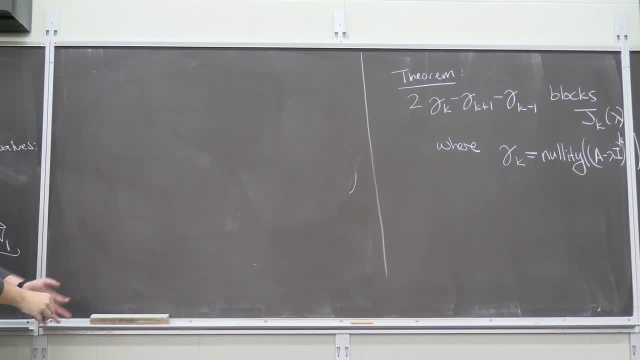 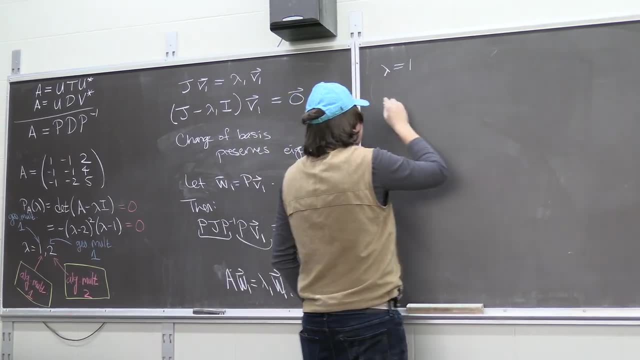 And so the theorem says, if we want to know what J is, we need calculate these guys gamma right For each Eigen value, for the Eigen value lambda equals 1 and for the eigenvalue lambda equals 2, we need to calculate. 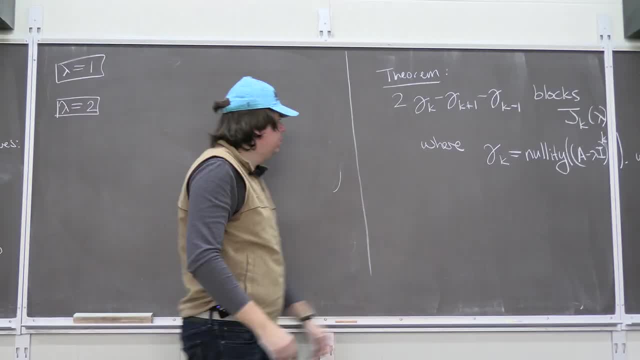 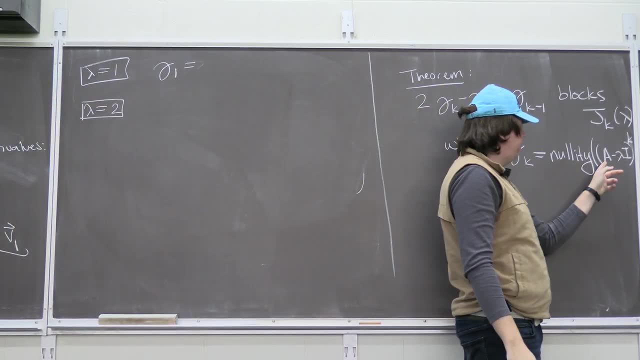 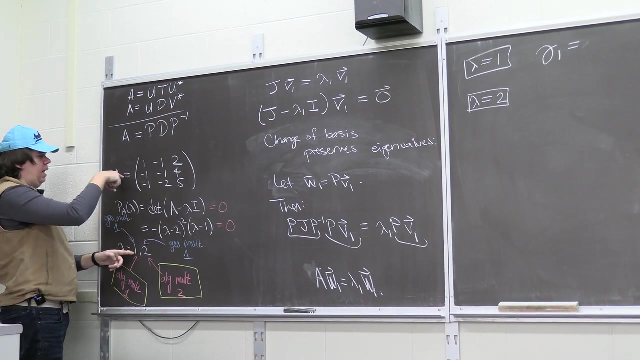 these gamma values. Now we've already calculated one of them. Gamma 1 for 1 is just the nullity of A minus lambda I, which we've already said. we already looked at this. we've looked at A minus a copy of the identity. we found the 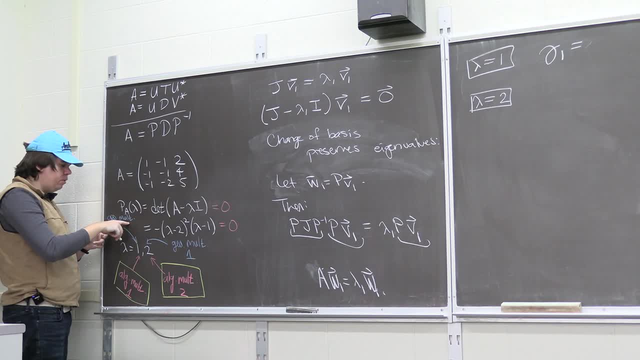 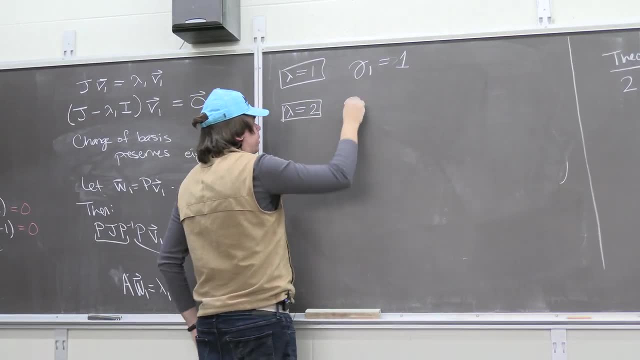 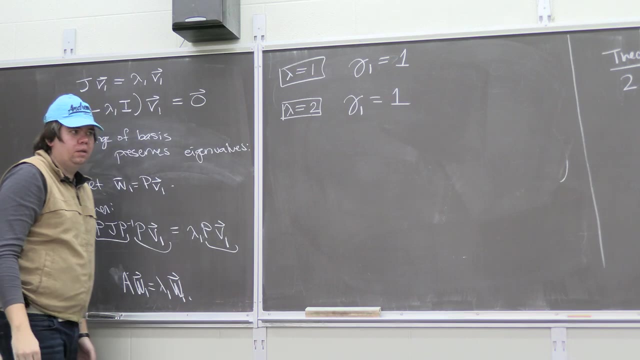 nullity. that's just our geometric multiplicity, right? So gamma 1 is just geometric multiplicity. we already found that it comes out to be 1.. And same thing down here. your gamma 1 for lambda equals 2, is also just equal to 1.. But if you 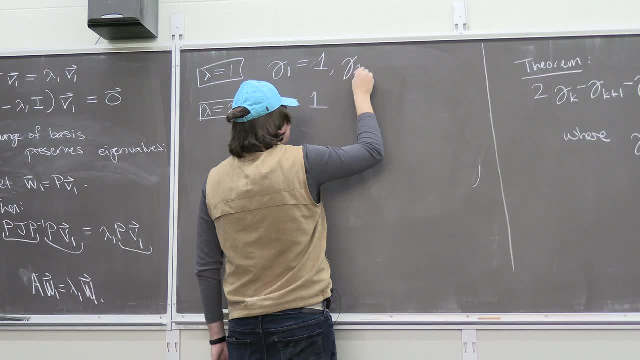 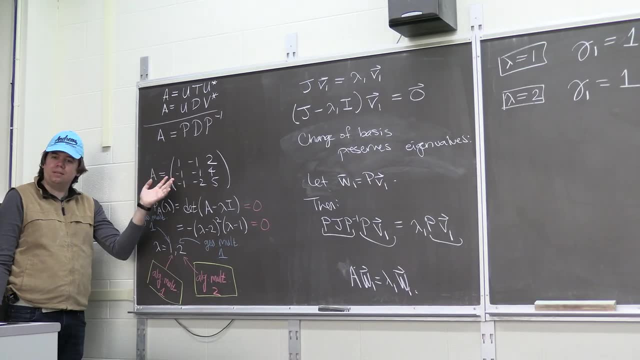 want to figure out what gamma 2 is. what we need to do is calculate for lambda equals 1, A minus 1 times the identity, square it, and then find the degrees of freedom in your null space that I mentioned in your. 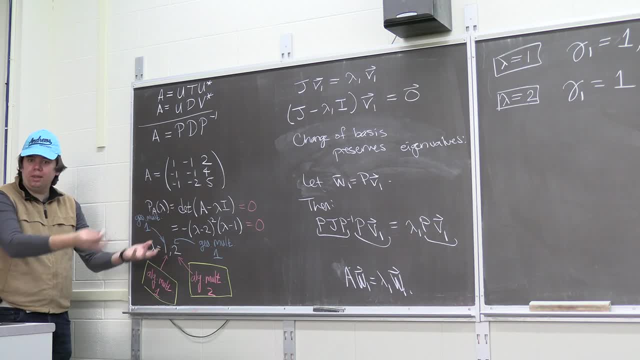 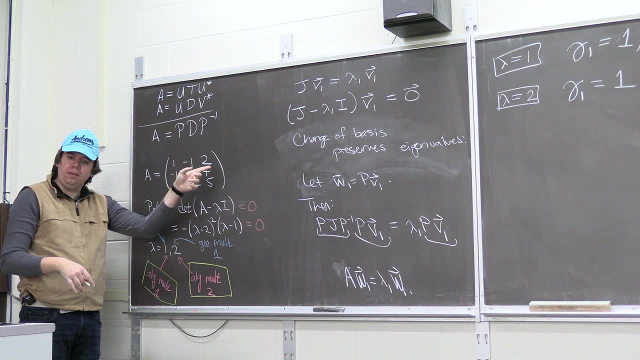 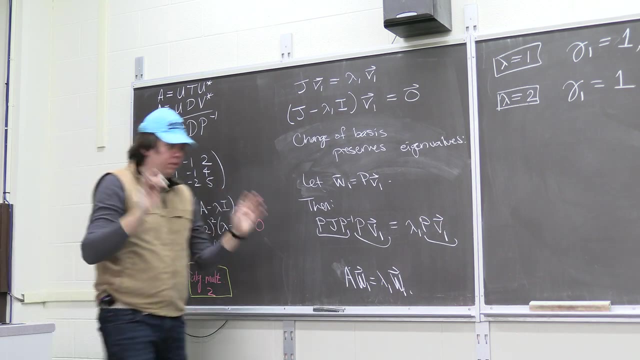 null space. We could spend a blackboard doing that. or you could type into Wolfram Alpha. you could be like you know this matrix minus 1 times the identity. you could say to the second power: you could just ask for the nullity, Wolfram Alpha would give it to you or whatever. 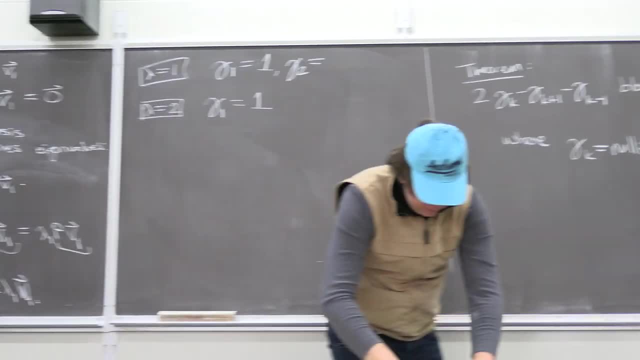 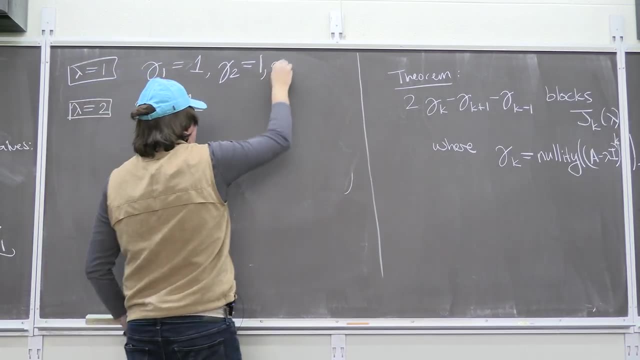 algebraic computing system you want to use. I did this last night. it came out to be dun-dun-dun, 1.. And then I kept going. I was like, what is gamma 3?? He's also 1.. And if you want to keep going, 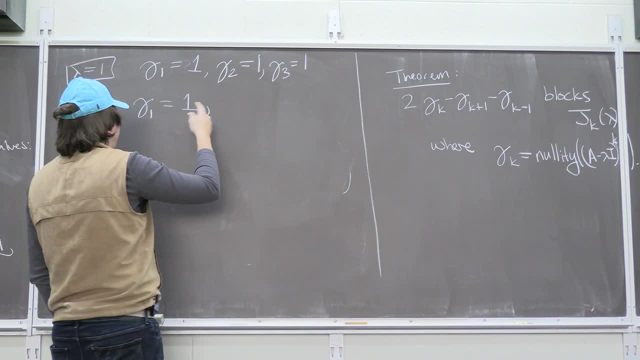 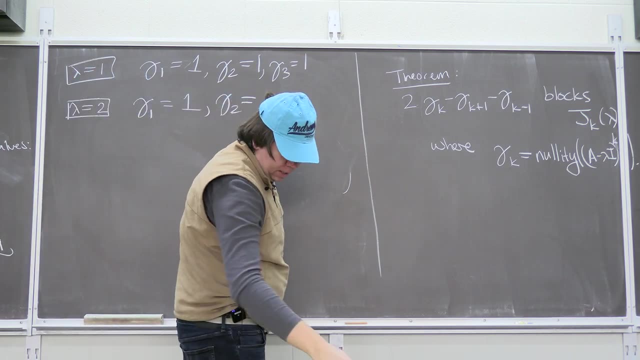 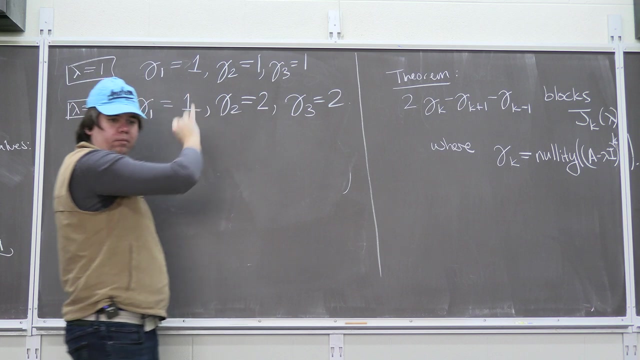 you can, but that's gonna be enough data for us. And then here we can ask: what is gamma 2, when your eigenvalue is 2, so now you subtract 2 times off the identity and it came off to be 2.. And what is gamma 3?? It's also 2.. You just type this into Wolfram Alpha, right? 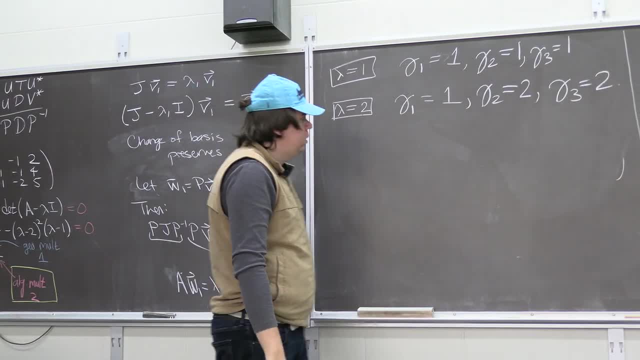 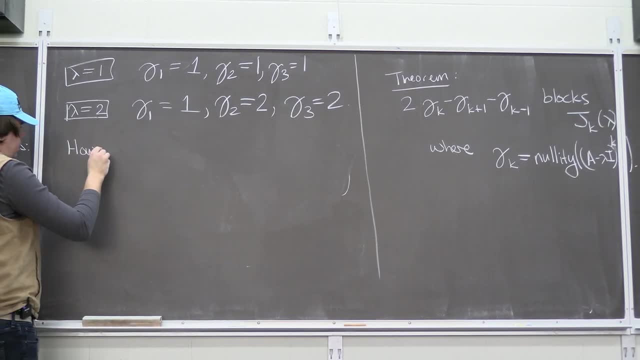 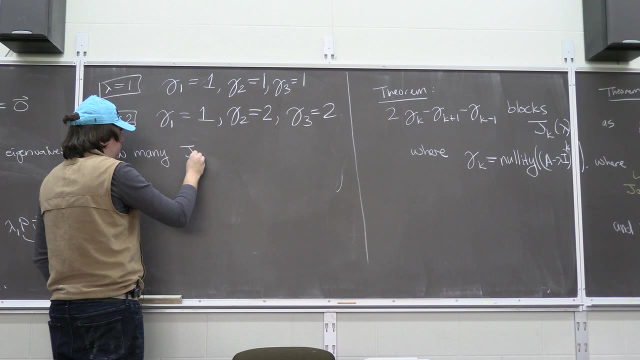 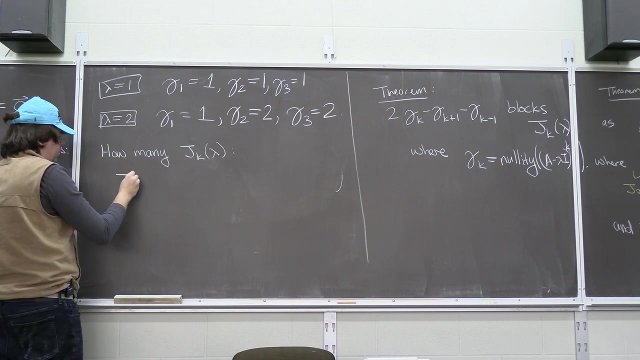 So what is this formula saying? Well, if you want to know how many blocks are there of the form jk lambda, we can just let's consider different values. Let's first do like: how many guys will it be? how many 1 by 1 blocks will it be for the eigenvalue? 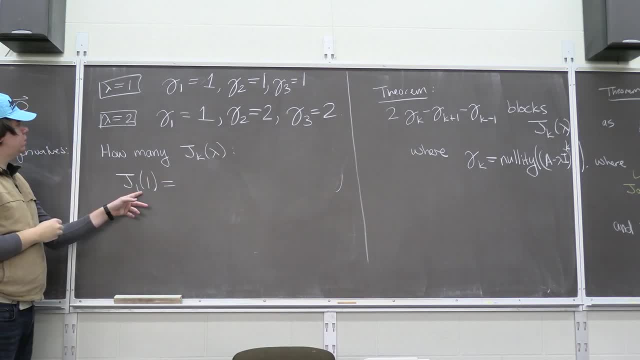 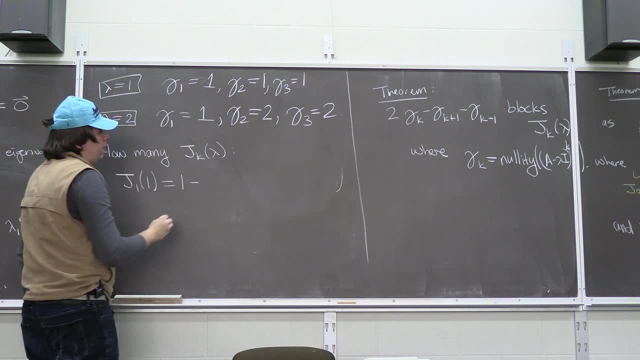 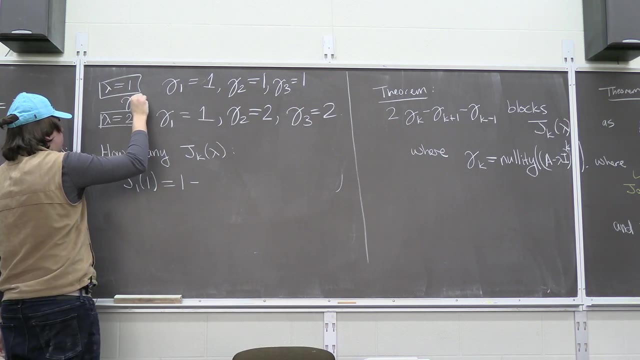 And you just say: well, according to the formula, it's 2 times 1 minus. okay, I haven't told you what lambda 0 is, Gamma 0.. So what is gamma 0?? Like, let's come over here and think Gamma 0, by. 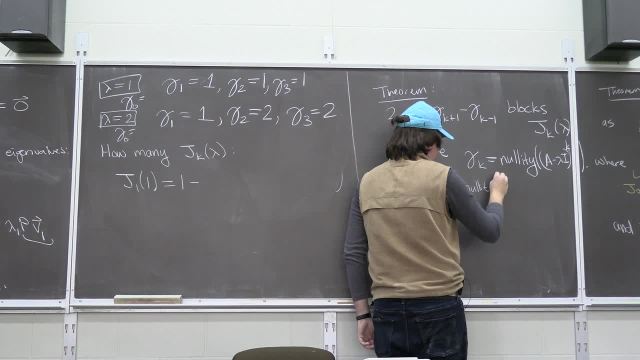 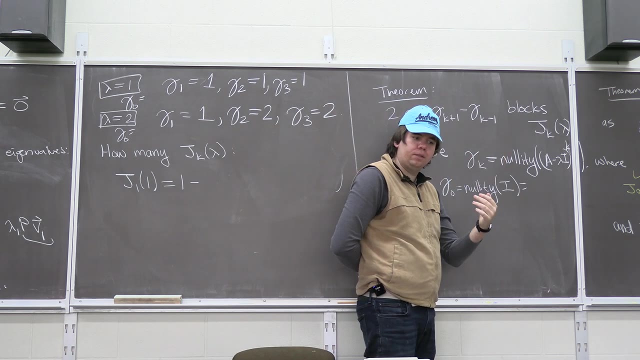 definition is just the nullity of what Some matrix to the 0th power. That's the identity matrix. What's the null space of the identity matrix? Just a single point, right. It's just the vector 0,, 0,, 0, or however many zeros you have. 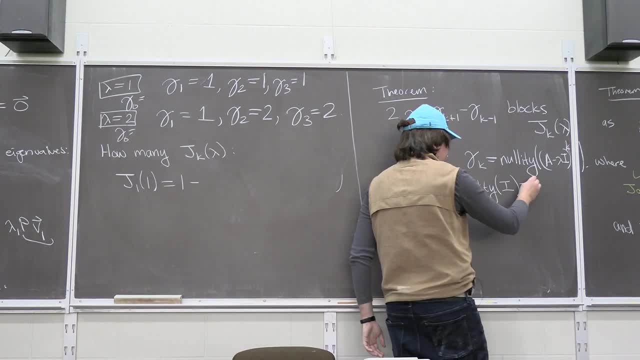 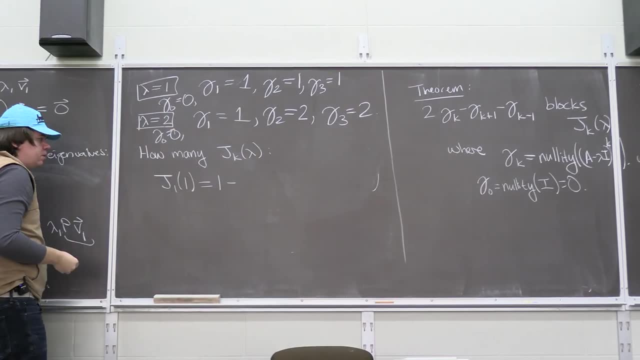 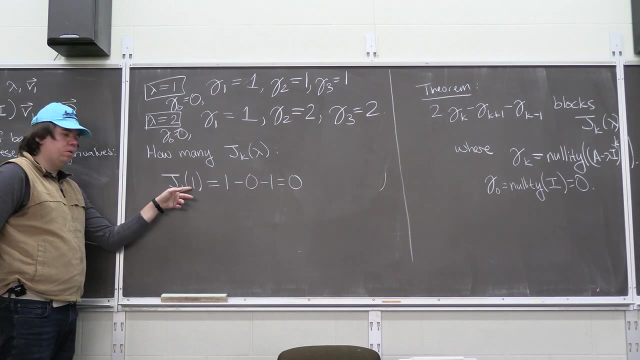 So the dimension of that is 0. So your gamma 0 is always 0. So my gamma 0 is always 0, regardless of the choice of matrix. So it's 1 minus 0 minus 1.. So this tells me there's gonna be 0, 1 by 1 blocks. 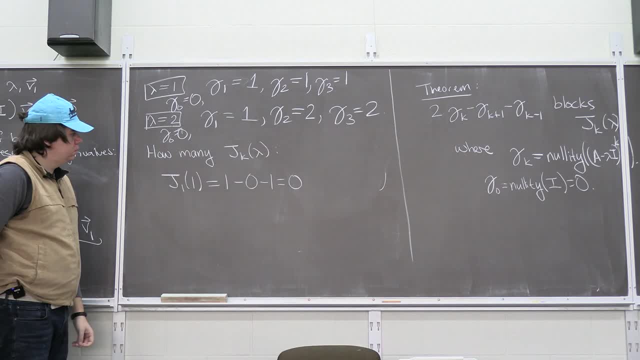 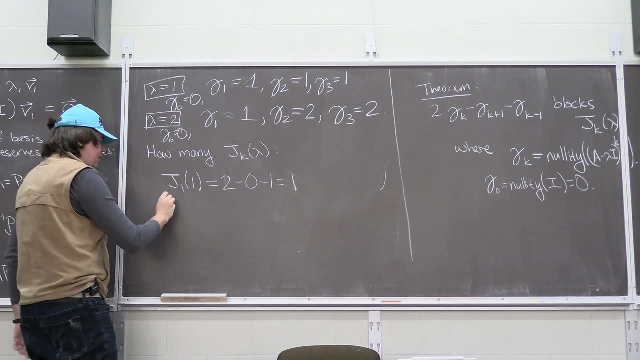 of with lambda 1. Yeah, Should there be 2 times Good, 2 times it. So now tells me that it's 1 block. Okay, very good, Thank you, I forgot about the times 2. And then you're like: well. 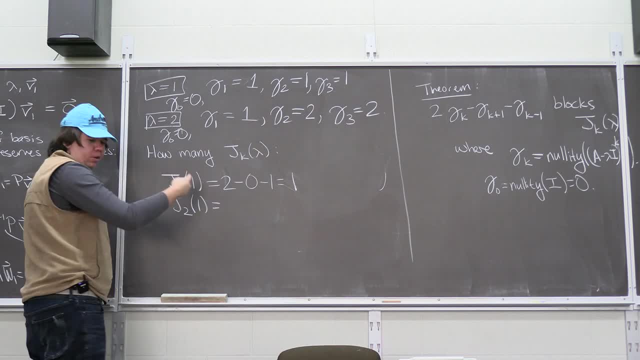 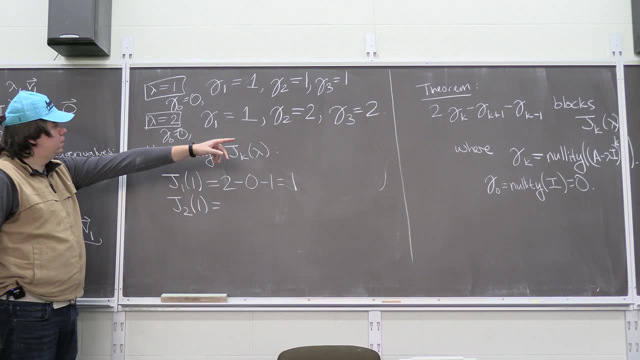 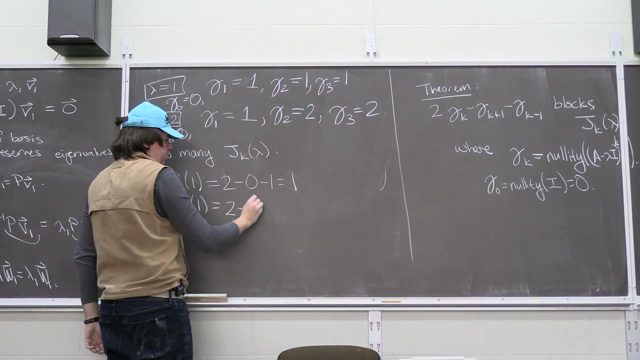 how many 2 by 2 blocks are there? And well, it's just gonna come out to be 0 now, because we've already found our block. There could be another block, but it won't be. I mean, plug this in 2 times gamma 2.. So 2 times 1 is 2. Minus gamma 1.. 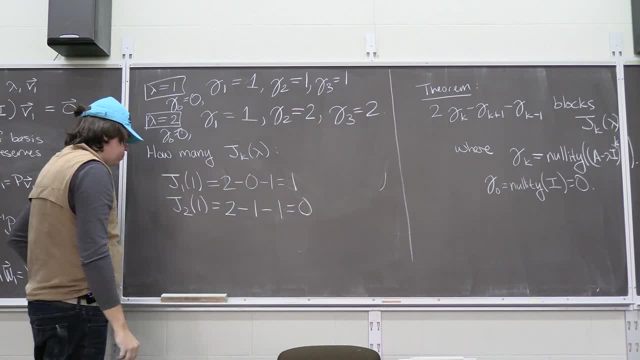 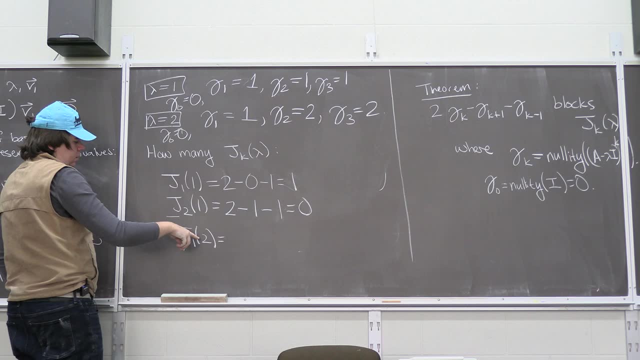 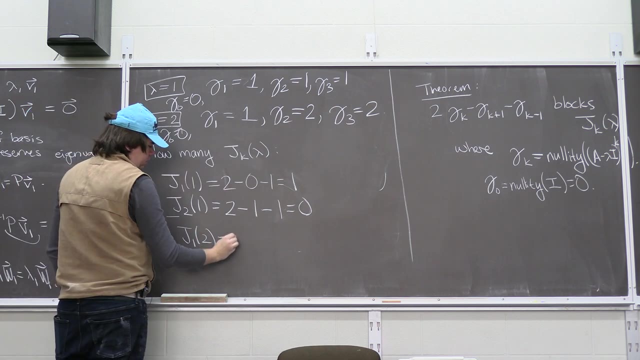 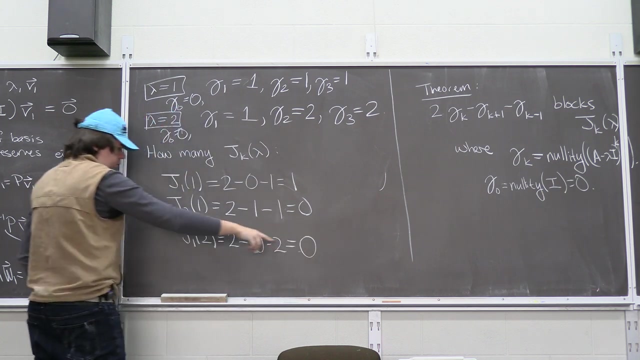 minus gamma three is zero, right? By way of contrast, how many one by one blocks are there, with your lambda equal to two. Well, now we do two times one minus zero. minus your gamma two gives you zero. So there's zero one by one blocks. 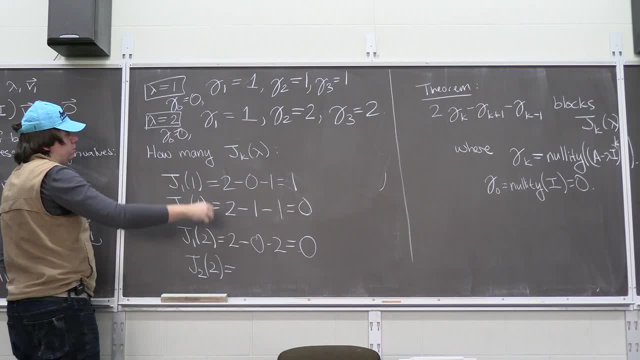 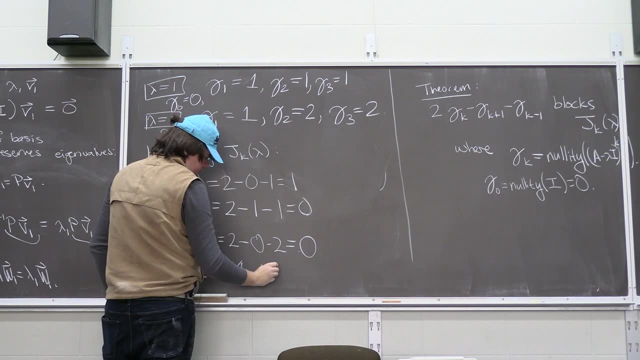 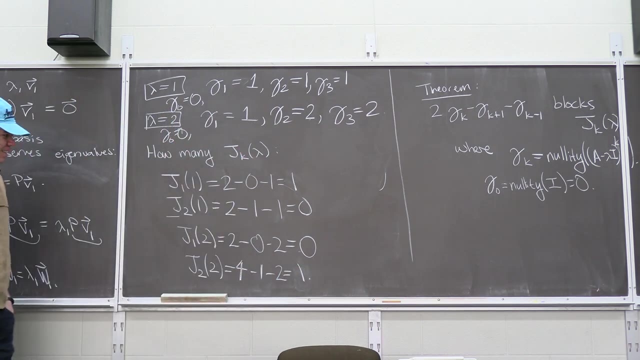 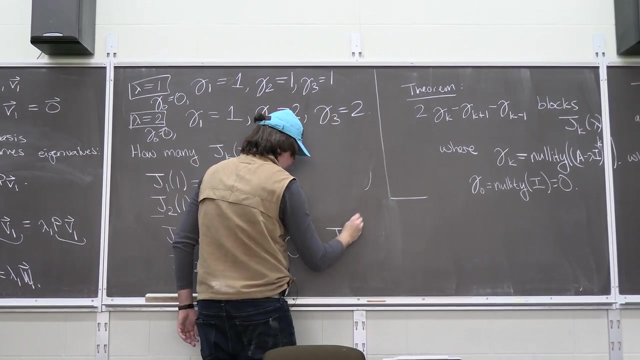 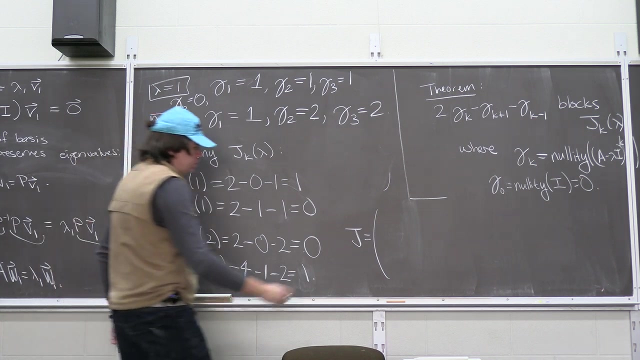 but how many two by two blocks are there? Two times two is four minus one. minus two gives me one. So what is my matrix J? What does J look like? It's got one one by one block with ones. So there's that block. 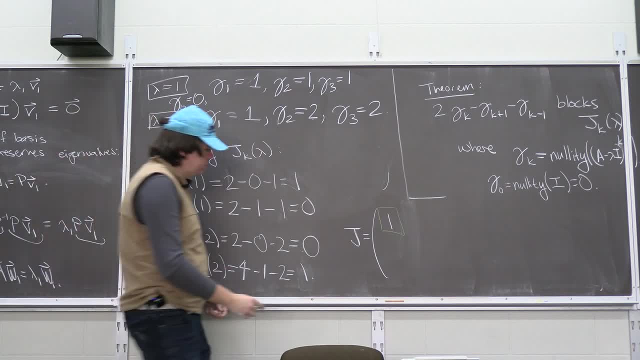 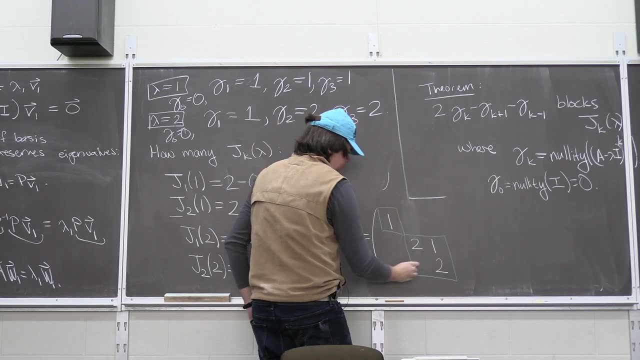 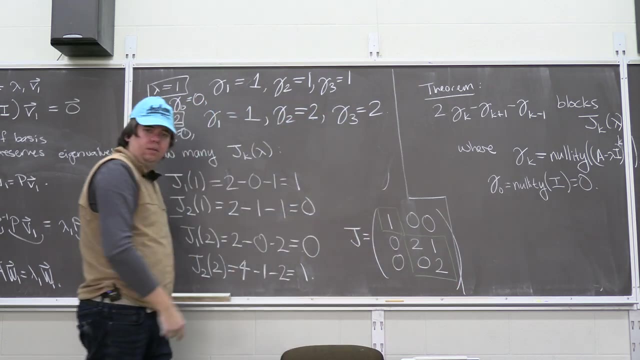 And then one, two by two block with twos, So that two by two block should look something like two, two and then a one up there And ones in the rest of this. So that's what my J looks like. So this theorem is just giving us a way. 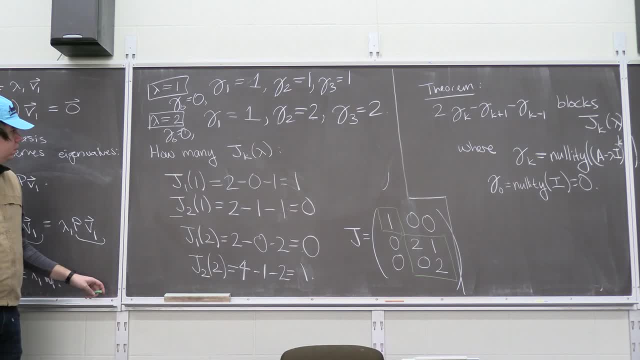 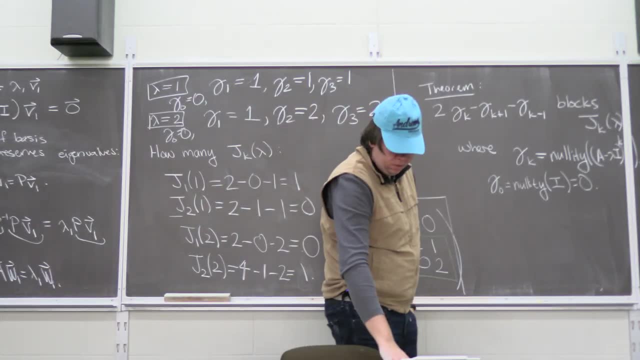 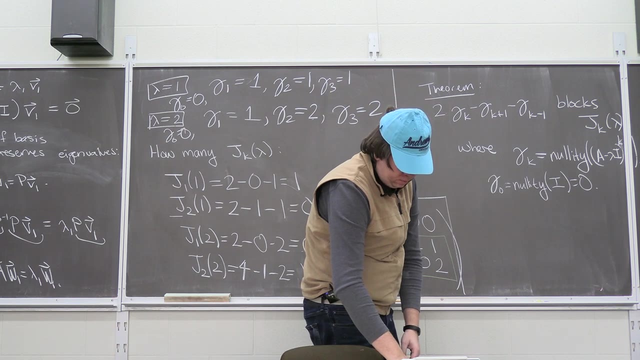 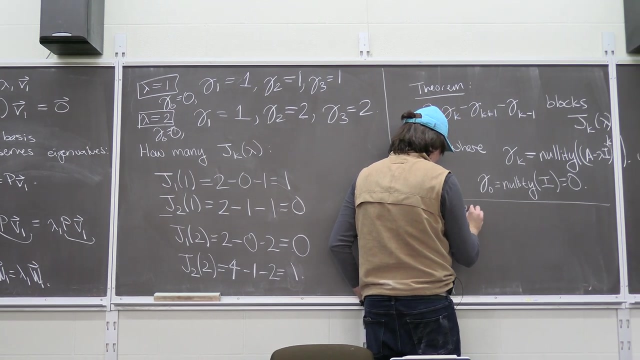 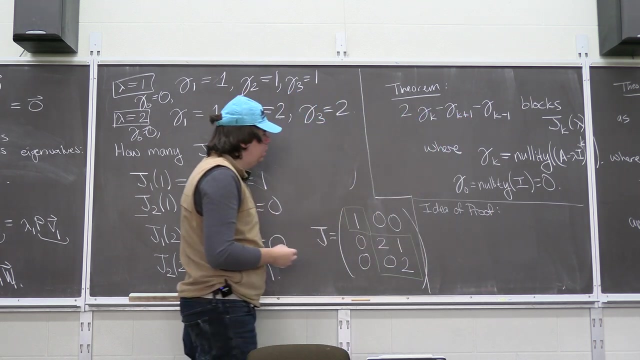 to count the number of blocks. Okay, So how might you prove this? So maybe I'll just say like a few quick words, So the idea of the proof. So we're really trying to. so I guess there's two key ingredients. 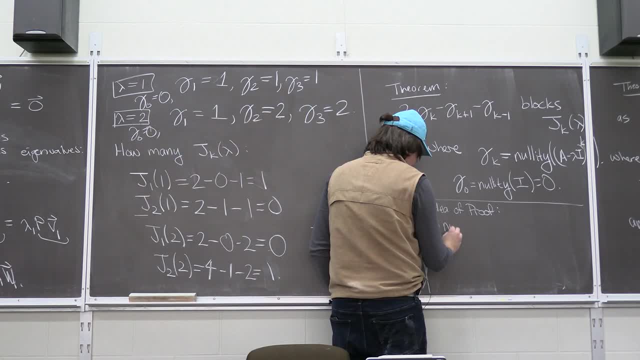 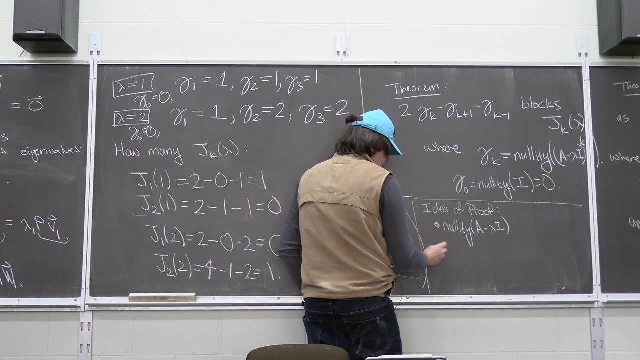 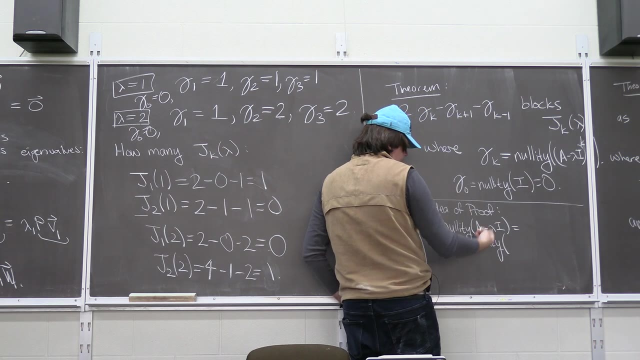 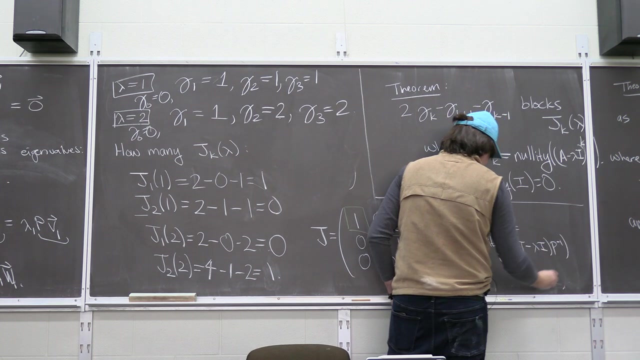 First, you need to convince yourself, when you're thinking about the nullity of some A minus lambda I, that that's the same as just the nullity of. you can pull out a P and P inverse. So it's just changing A to J and there's some change of basis. 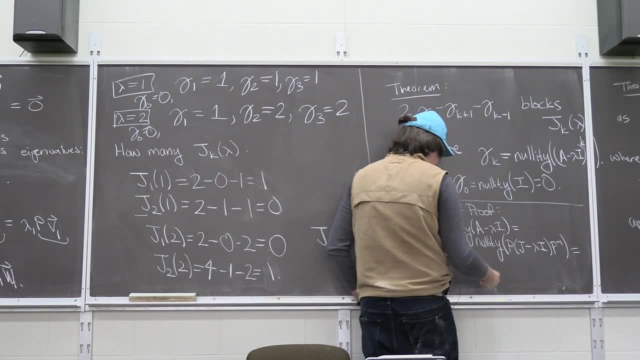 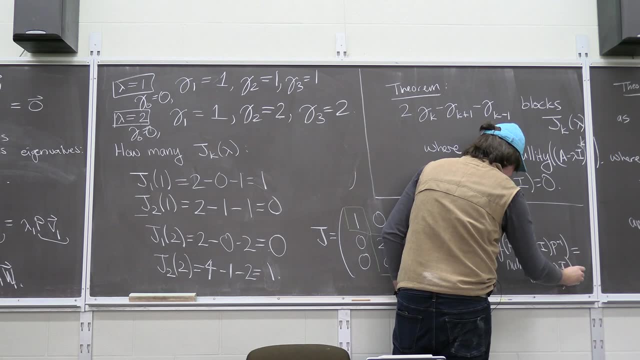 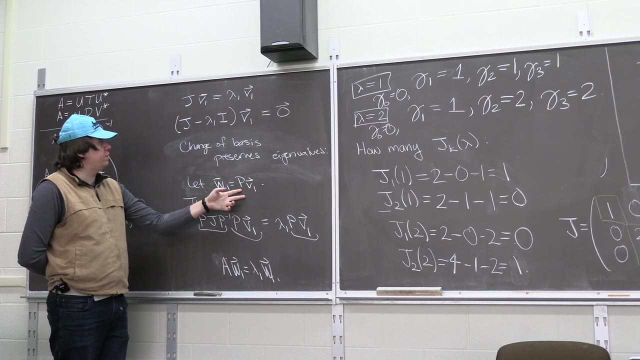 And nullity is preserved under a change of basis. So this is just the nullity of J minus lambda I. So if we come back to this example, your change of basis does not preserve your eigen vectors. your eigenvector changed from V1 to P times V1.. 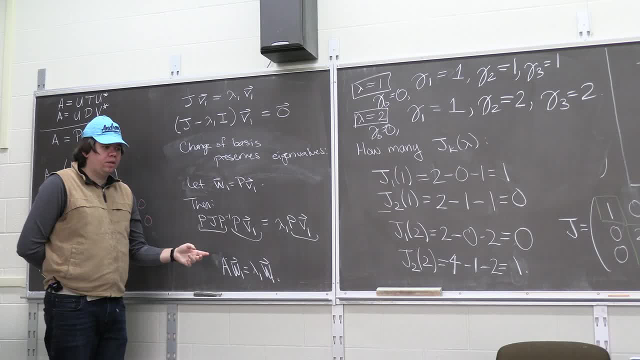 But P is an invertible matrix, So it's going to preserve whatever you should: some collection of vectors of dimension three And you multiply it by an invertible matrix. nothing gets lost, right? Nothing's getting sent to no. non-zero vectors can send to zero. 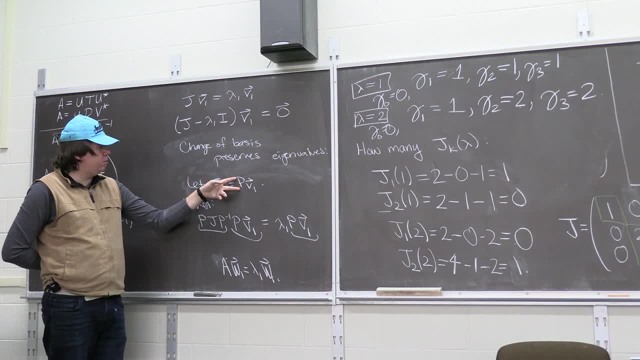 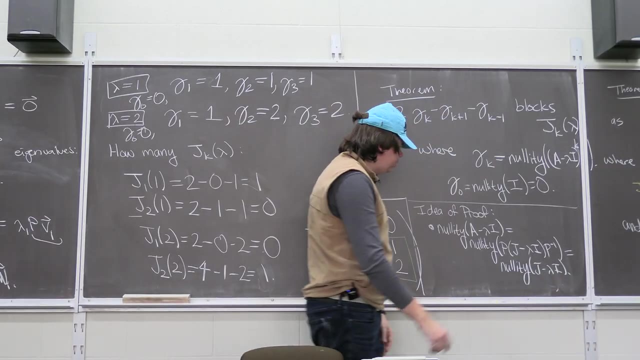 So nothing's been collapsed away. So, since P is invertible, your nullity is is preserved, the dimension of your null space is preserved, the particular vectors are changed from v1 to p of v1, but the dimension is preserved, so that allows you to move from here to here. okay, so then? 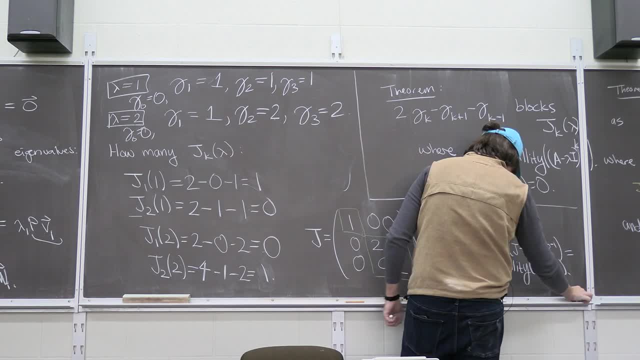 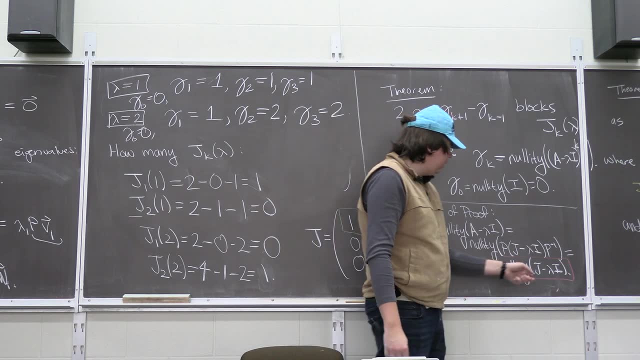 what you just do is you just sit down and you spend you know 20 minutes thinking about what the nullity of j minus lambda i looks like and you're like, oh okay, well, depending on what your values of lambda are used to be clearing out all those lambdas into zeros for one of those blocks. 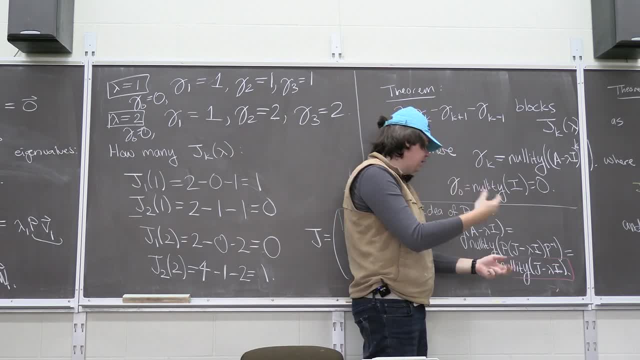 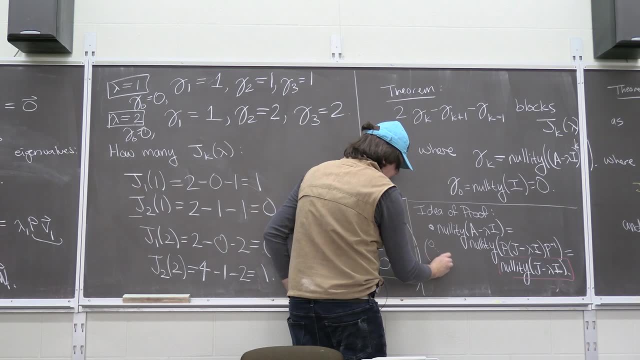 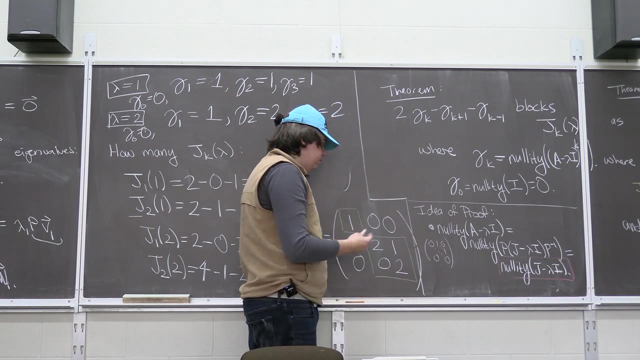 right, and then you kind of start thinking about: okay, how does that impact the nullity? and and then you just think a little bit about if you do have a block that has zeros all along the diagonal and ones above it, what does that matrix look like? what's the nullity of that matrix? and it turns 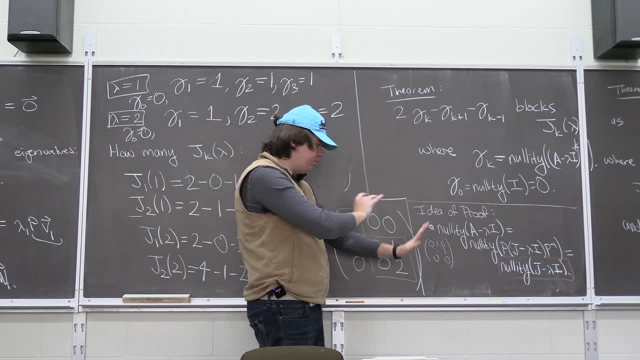 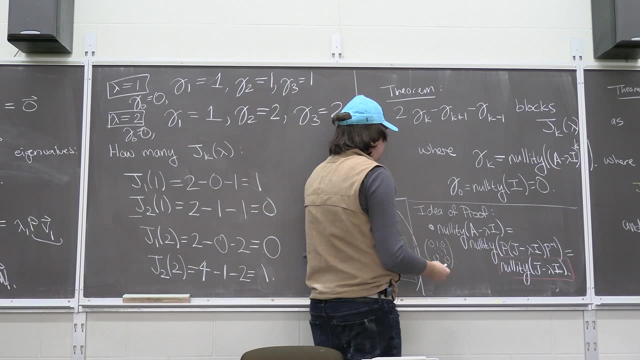 out. if it's like a k by k matrix, it's null to k. you do some clever counting argument, so there's some, you know, chasing there, but what you end up with at the end of the day is you get this nice formula that says that the number of blocks 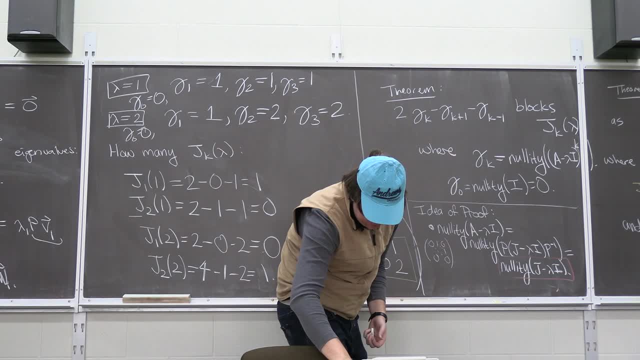 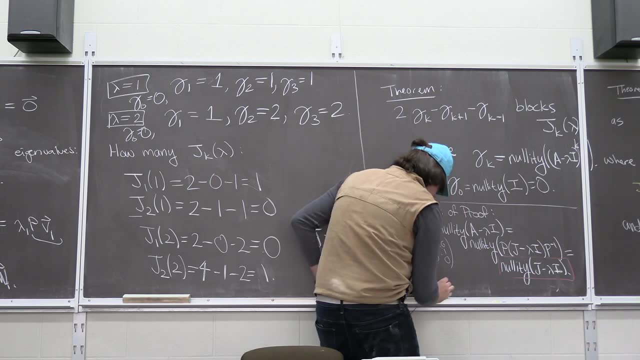 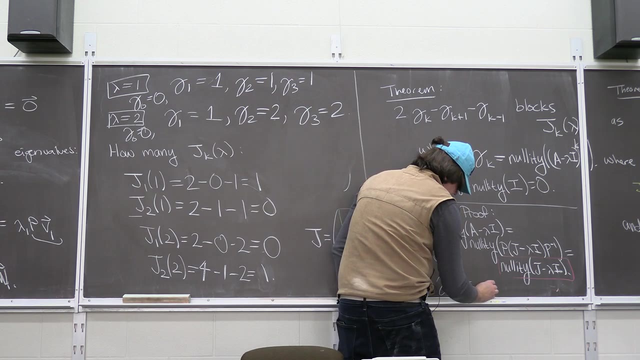 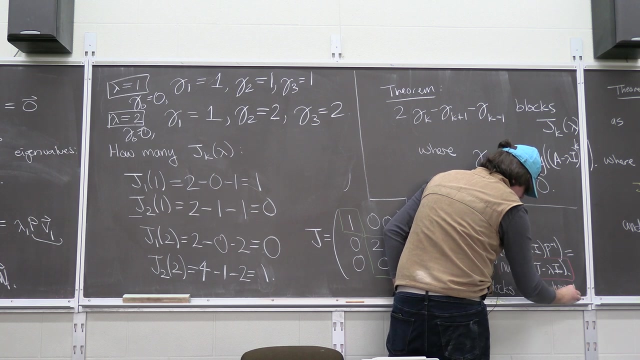 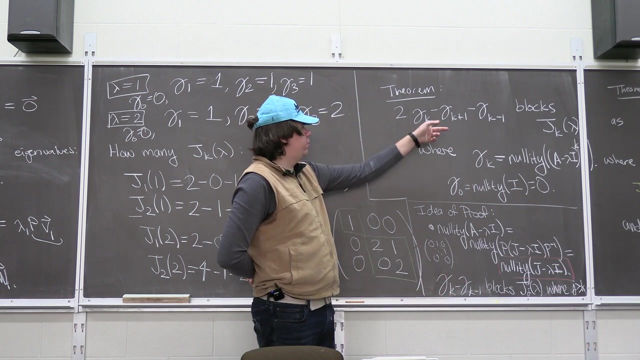 well, let me, let me just write it: the number of blocks of size at least k. you end up with gamma k minus j, a gamma k minus one um blocks j of size at least k, so j sub j, where j is at least k, and then from this you can recover your original formula. 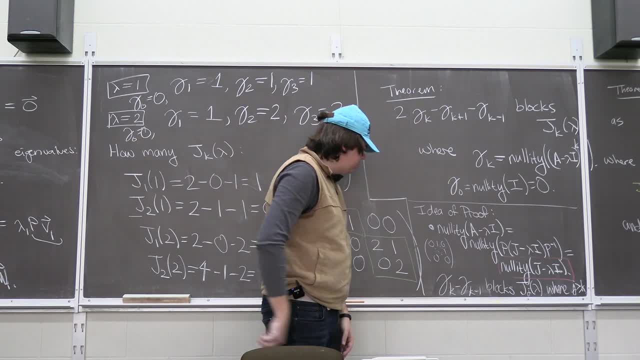 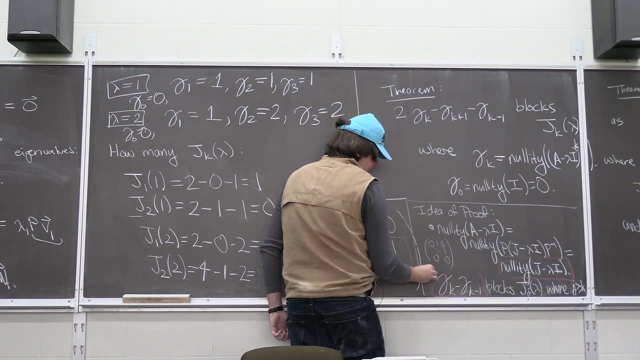 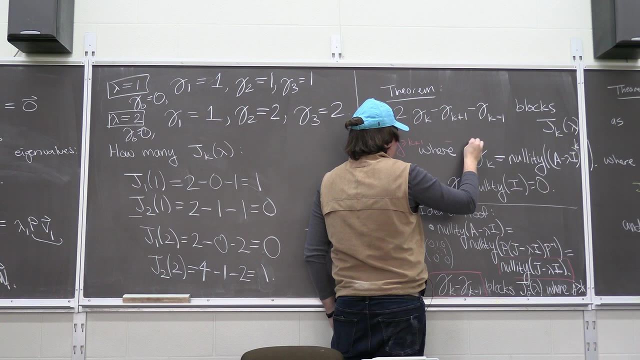 right, like if this is the number of blocks of size at least j. then you're like: how many blocks do i have size exactly k? well, all i need to do is i count the number of blocks where j is bigger than equal to k plus one, and i minus the number of blocks where j is greater than or equal to k. 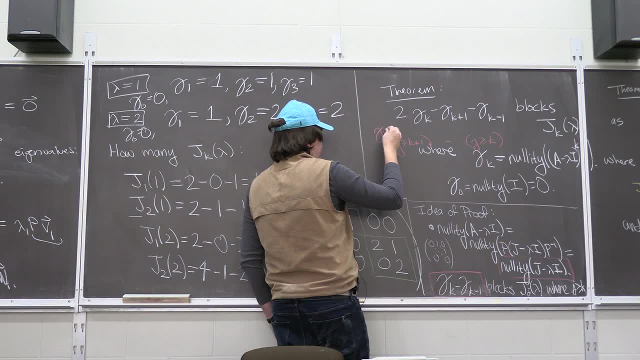 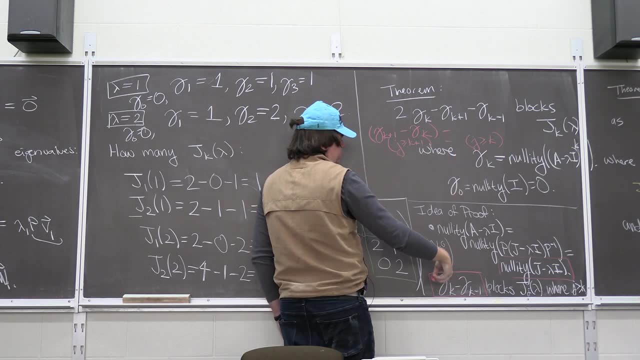 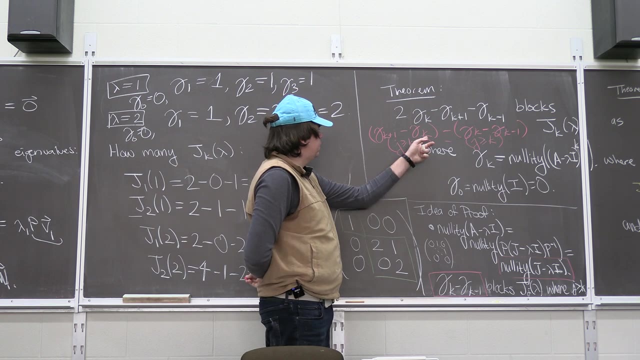 and so you just have this formula: gamma k plus one minus gamma k, because i've shifted it all by one minus what j is at least k, gamma k minus gamma k minus one. and then you do some arithmetic in your recovery. original formula: oh, did i do that backwards? 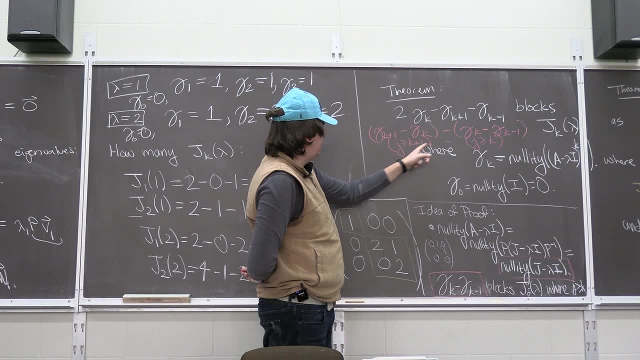 ah, yeah, i did this backwards. i want to count the number of blocks exactly size k, so i want to subtract off all the ones that are bigger than size k, and so here you get gamma k plus a copy of gamma k, so it's two gamma k's. 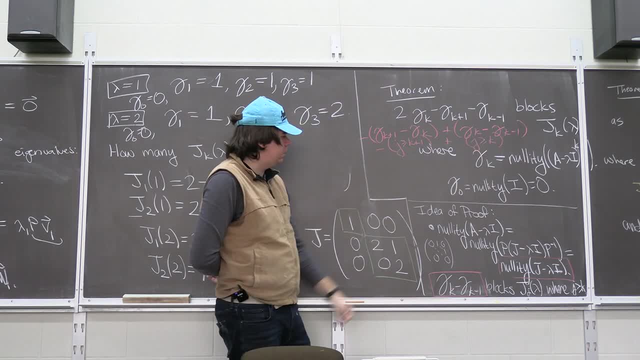 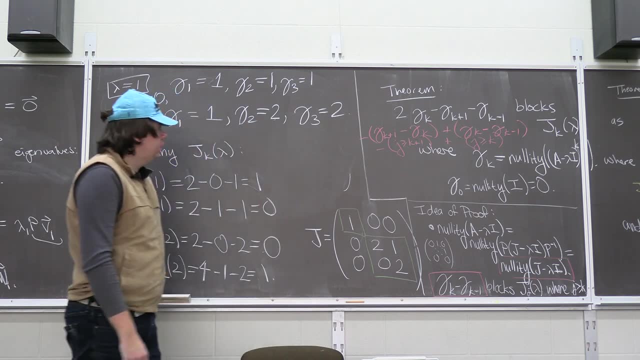 here you have your minus gamma k minus one. here's your minus gamma k plus one. okay, so you're getting traced to that proof. that's fine. but what i want to point out in closing is we have a theorem that tells you the number of blocks. yeah, i'm just gonna give you a little bit of time so you can see that you'll get your number of blocks. 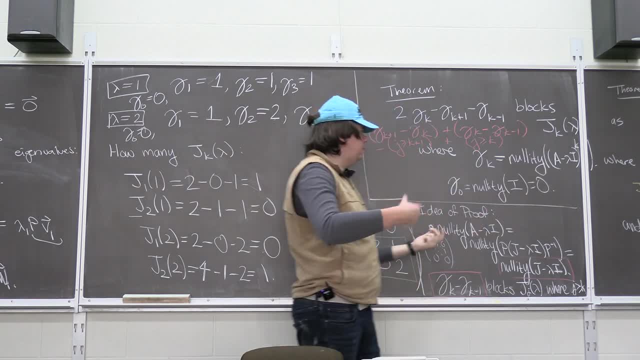 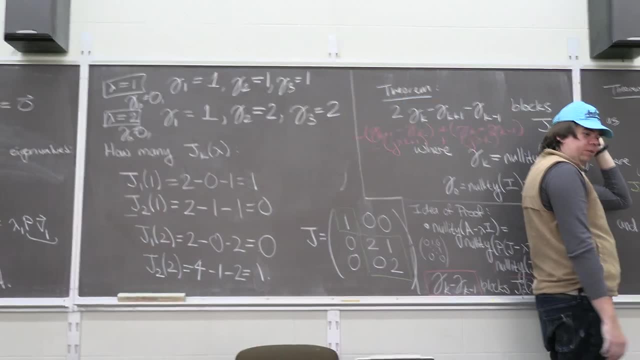 blocks you get. So it's like it's not. it's not like it's like some mystery. It's dictated to you how many blocks you have of each size, And hence given a matrix A. there's now an algorithm that 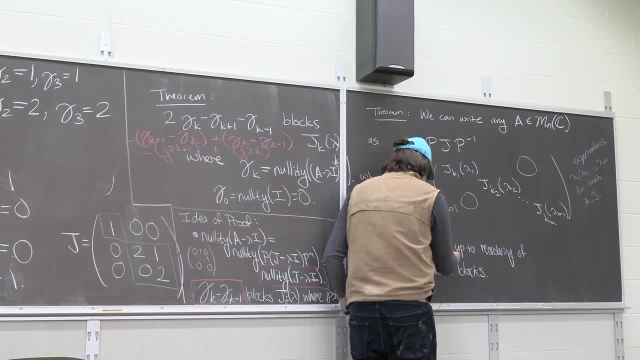 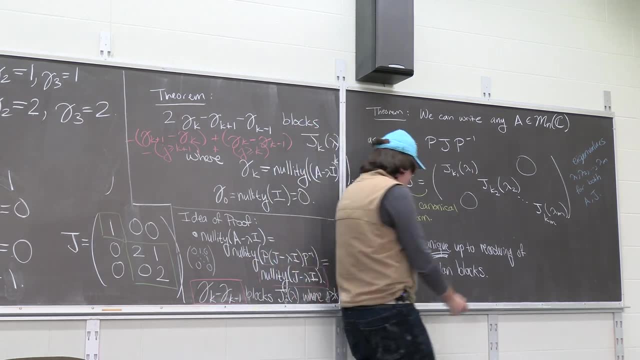 tells us how many there will be of each size And thus it's unique, right? It's not like you can come up with anything else. You just follow the algorithm and it tells you Unique up to reordering, because it only tells me the number I have of each size and I could always, you know, change them. 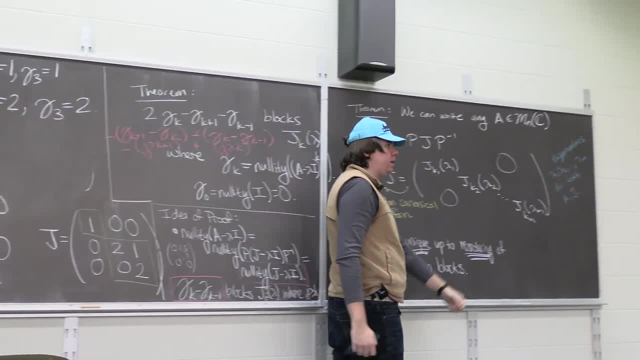 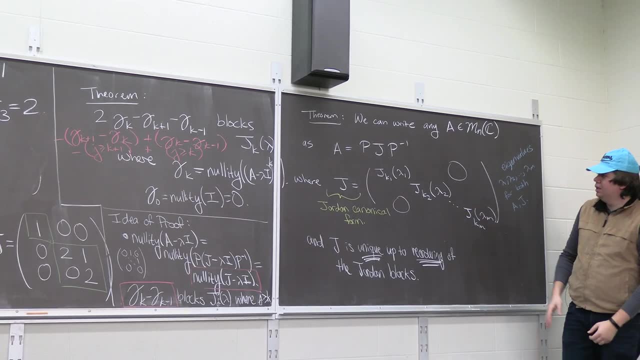 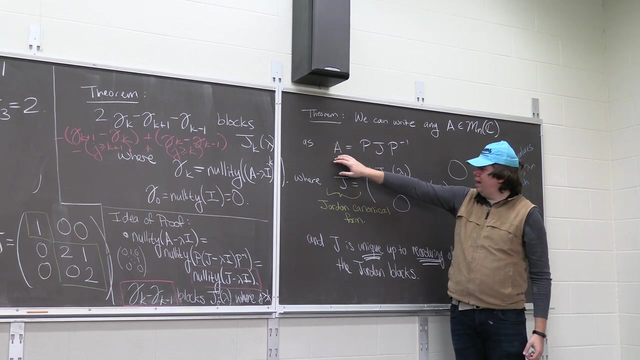 around, which exactly corresponds with changing the columns of P. So here's the big theorem. We're going to come back to it Wednesday. We'll talk about some corollaries of it. We're going to try and prove the existence, part of it, But at least we see the uniqueness that every matrix A has a. 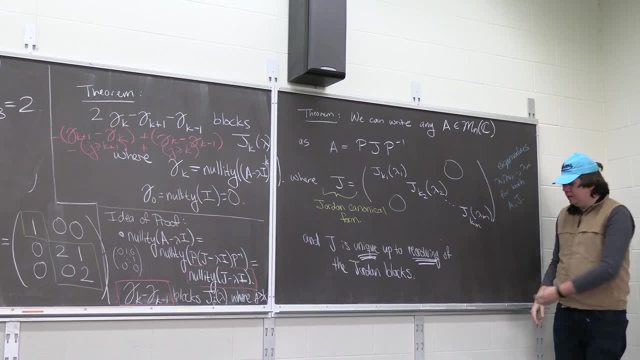 unique Jordan canonical form corresponding to it, And so we'll talk about the implications of that in our next lecture. Professor Dave here, let's talk about quantum electrodynamics. 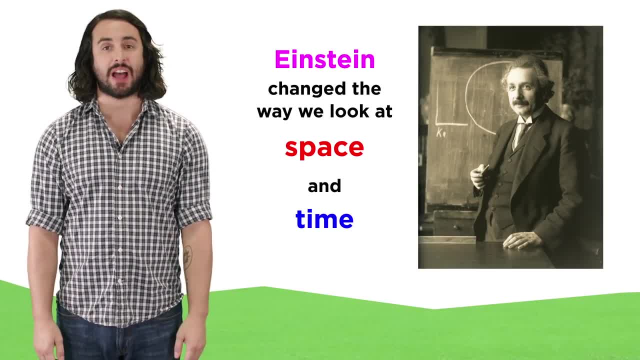 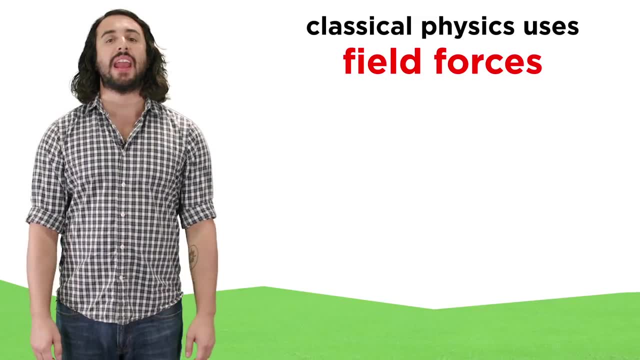 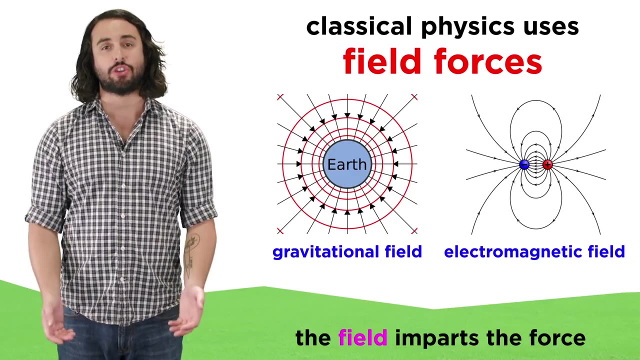 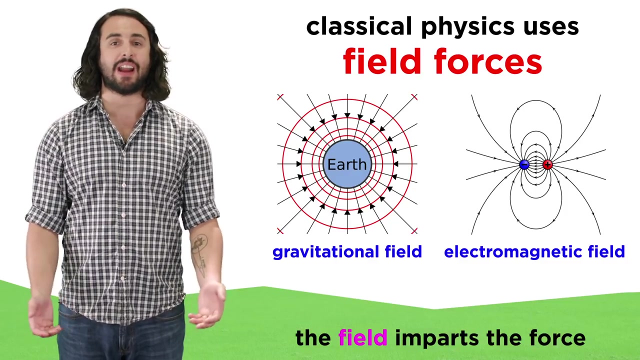 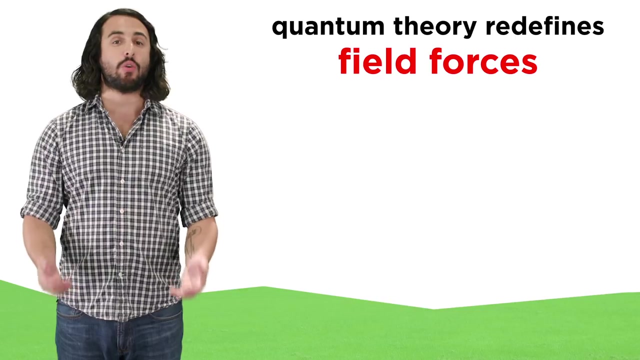 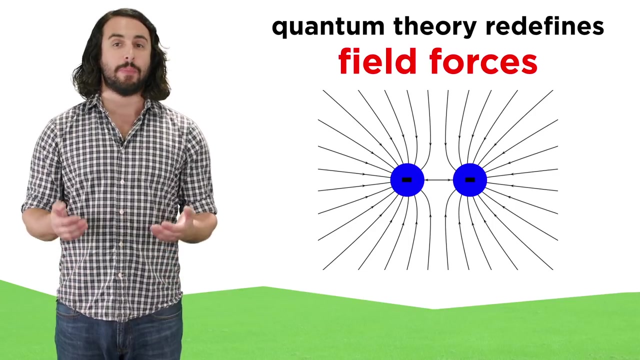 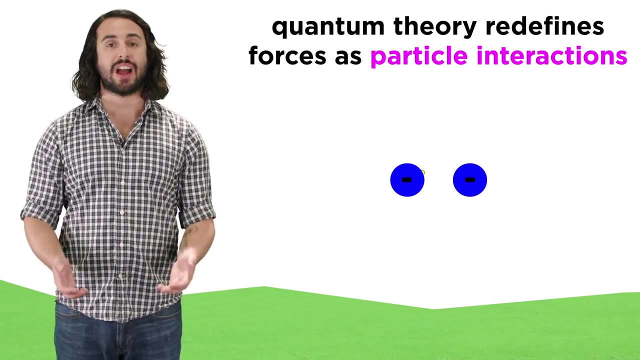 After spending some time with Einstein looking at the nature of space and time, we have to go back to the quantum realm and pay some attention to particles. In classical physics, we became aware of field forces, like gravity and electromagnetism. These are forces whereby a gravitational or electromagnetic field imparts force onto some object, which generates an acceleration in that object, like a rock falling to the earth, or the attraction and repulsion between charged particles. But as quantum theory progressed, it began to find a way to redefine these field forces and show that the idea of a field becomes obsolete if we are instead able to explain these forces as the interaction between certain components of the field.